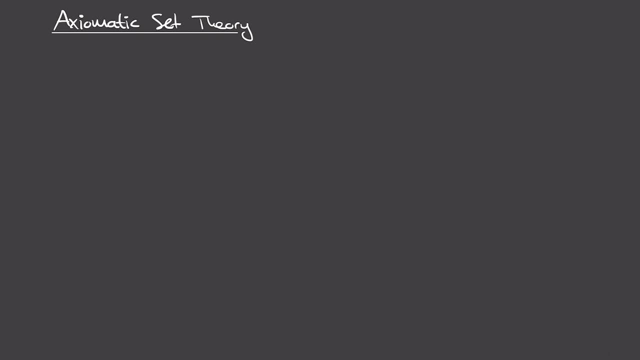 So these are a set of nine axioms that allow us to build up all of set theory based on first-order logic And well from there, because most of the rest of mathematics can be formulated in terms of axiomatic set theory. you can, in principle, think about these axioms as being the foundation for well all of modern mathematics. 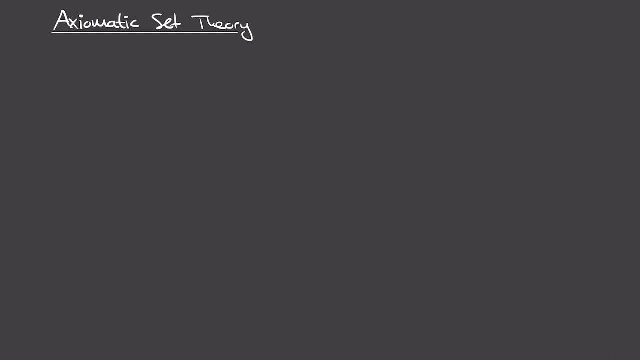 In this video. I'll start out by listing all of the axioms in sort of an informal manner to give you an overview of what they say, And then in the remainder of the video we're going to go through each of them in detail and explain exactly what they mean. 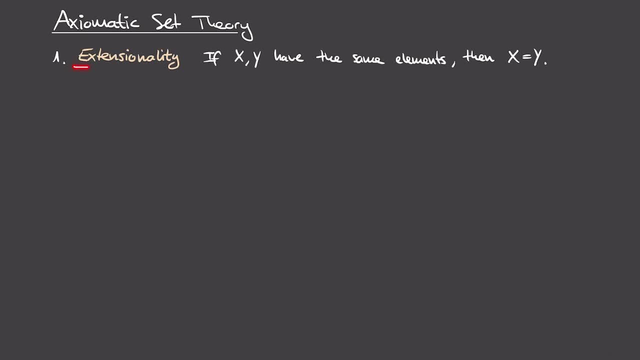 The first and perhaps most important axiom is the set theory. The most fundamental axiom is called extensionality and it tells us when two sets are to be considered to be equal. So it says that if sets X and Y have the same elements, then in fact X is equal to the set Y. 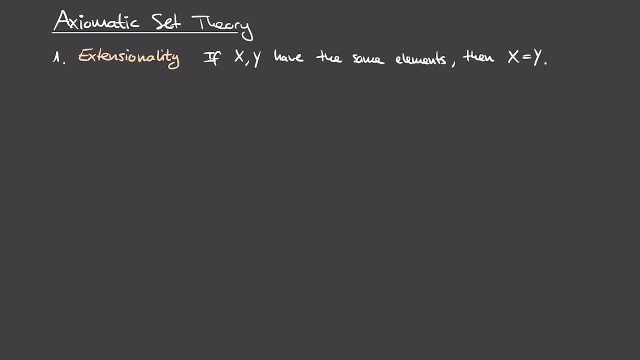 This is precisely the definition for equality of sets we gave in the naive treatment of set theory, and here it forms the first axiom of ZFC. The majority of the remaining axioms of ZFC assert the existence of certain sets. So the second axiom here is called pairing. 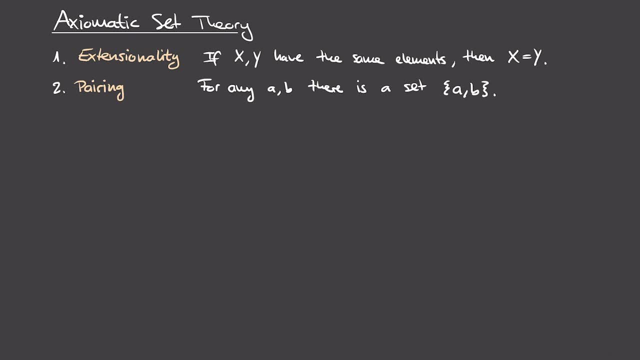 and it tells us that whenever we have two sets, a and b, there is a set that contains exactly those two elements, a and b. In other words, if we already have two sets, a and b, then we can form a set that contains those sets. 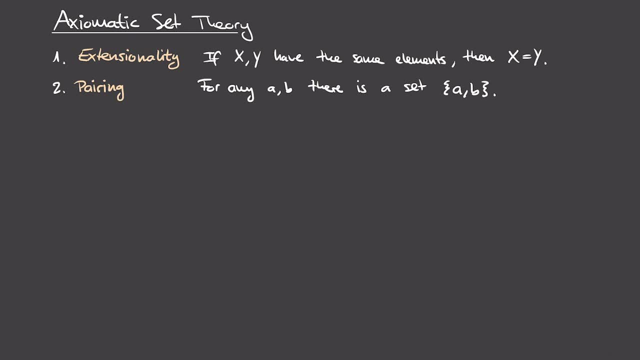 Now I should mention that in this ZFC axiomatic set theory, all the objects we'll be considering are themselves sets. So while in our naive treatment we thought about a set as being sort of a collection of any sort of object, here the objects that we'll be considering are all themselves sets. 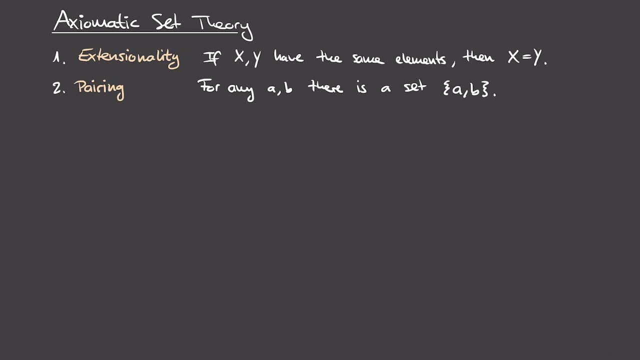 This isn't in fact a big restriction, because you can construct many of the usual mathematical objects based just on sets using these axioms. For instance, you can construct the natural numbers using sets and from there you can basically construct the integers, the rationals and the reals. 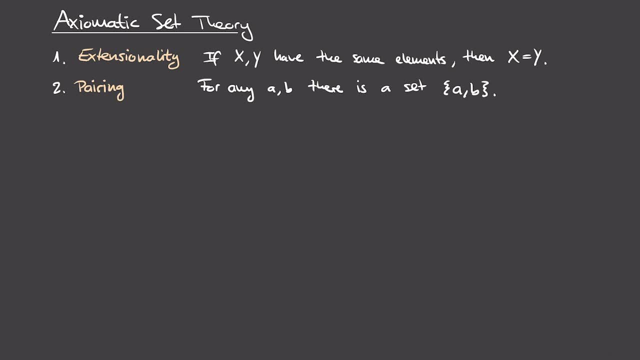 also realized as certain sets, And so in principle sets can then actually be numbers, like real numbers for instance. This means, that the pairing axiom can sort of be interpreted as saying: if you have any two objects, a and b, then there is a set containing those two objects. 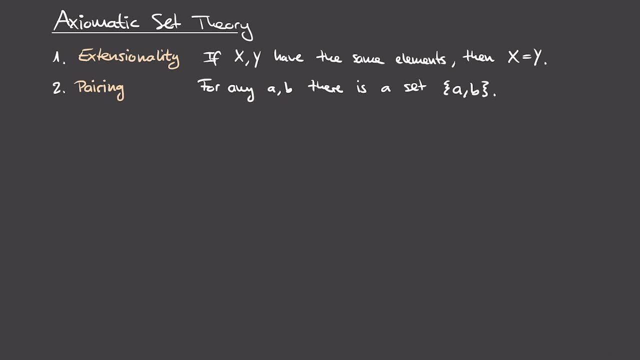 but while these objects here in ZFC are themselves sets, but they could represent things like numbers too. So, for instance, The third axiom is called separation, and it gives us this weaker version of the comprehension property we saw in the last video. 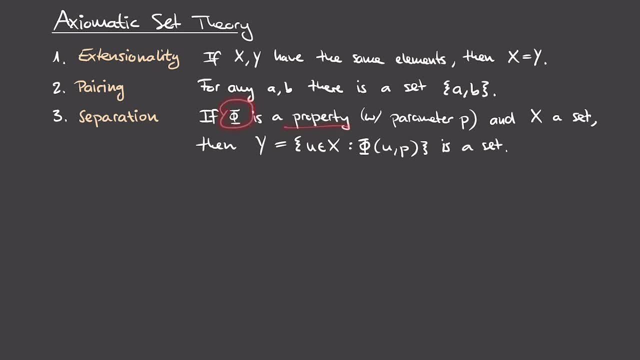 It says that if capital Phi is a property, which means that it's some first-order logic formula that possibly can depend on a parameter p, so p here is just some sort of free variable occurring in this formula, and then we take some set x. 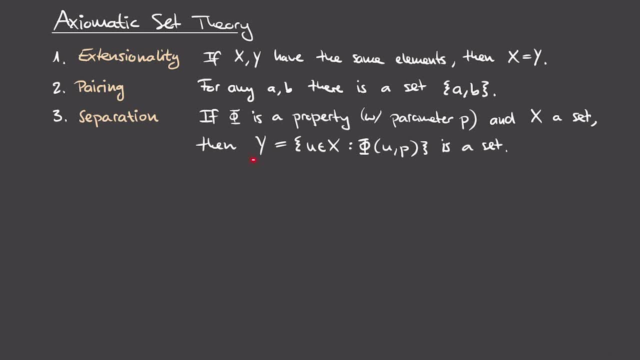 then we can form a set y that consists of all the elements u and x that satisfy this property, capital Phi. And moreover, this y, which consists of sort of a filtered version of the set x, is itself a set. In other words, if we have any set x and we have some property. 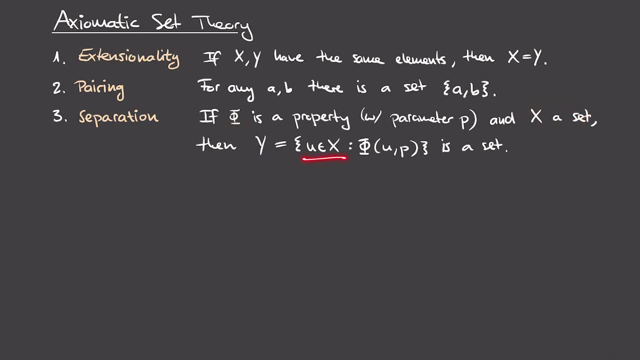 then we can form the set of all elements occurring in x with that property, and that thing, according to this axiom, is again a set. Now, the reason this is a restricted version of the comprehension principle we saw in the last video is that here we're sort of only filtering this set x. 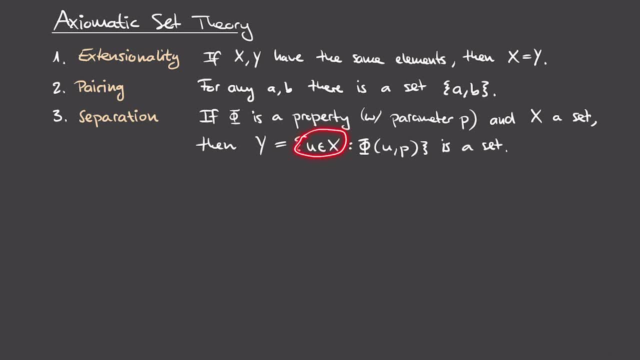 so we're only considering elements u that occur in the set x that satisfy the property, and we're not considering any sorts of elements whatsoever that satisfy the property. In other words, using this separation axiom always only gives you subsets of existing sets. In particular, this means that you can't. 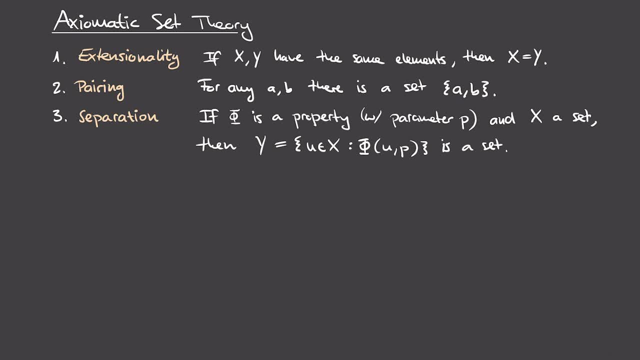 use this comprehension principle here to construct very large sets like the set of all sets or that sort of thing. The fourth axiom here tells us that unions exist, and it says that for any set x there is a set y. that is just a union over x. 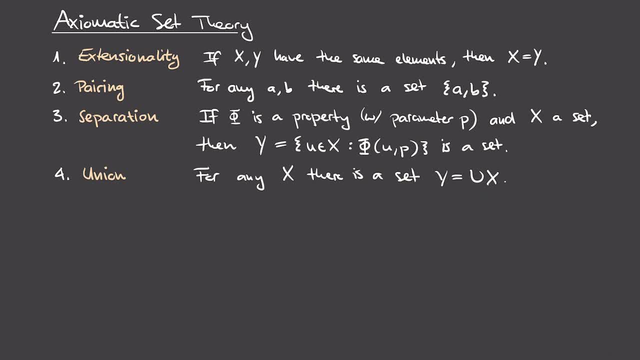 Now here. this is slightly different than the version of unions we saw in the last video. So in the last video we saw like binary unions, so unions of two sets, and a union of two sets just contained all the elements that occurred in either set or both. 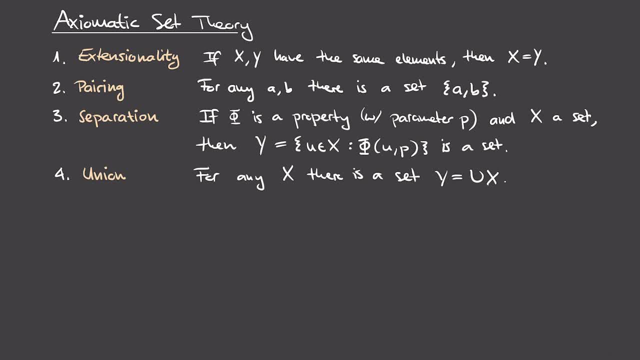 This version of unions here works in a different way. So here we think about x as being a set of sets, namely the set of sets that we want to union together. For instance, if x consists of, let's say, sets a1,, a2, and a3,. 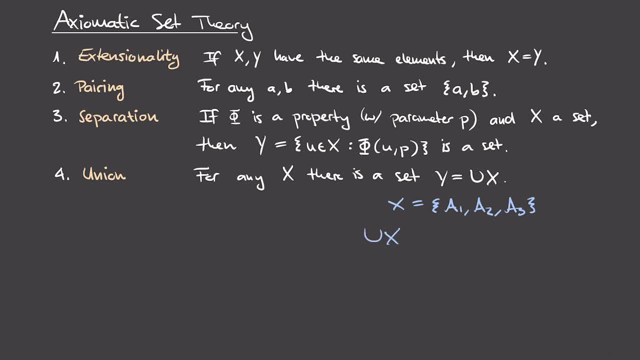 then the union over x would consist of all the elements that occur either in a1, in a2, or in a3, or in multiples of them. So if we would write this with our binary union notation, this would somehow be the set a1, union, a2, union, a3,. 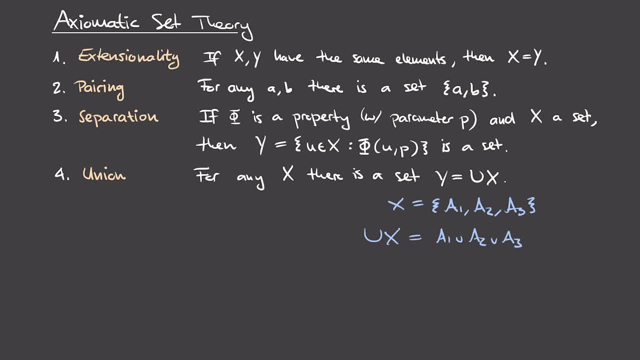 where this small union symbol here is the binary union. In other words, this big union here is just a way to union together a family of sets, and this family of sets is well x In particular, we can realize binary unions. 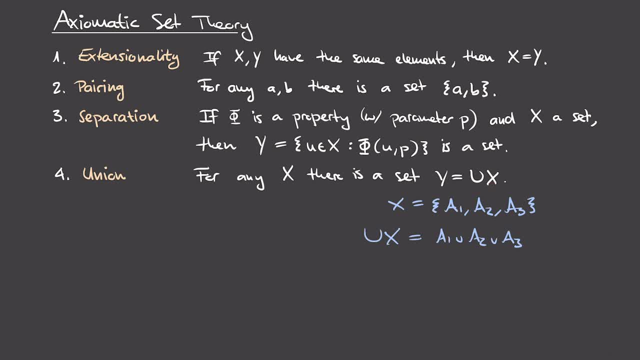 but we can also union over an infinite collection of sets using this axiom. Next, axiom 5 tells us that power sets of sets exist. So for any set x, there is a set y, namely the power set of x. So that's the set of all of the subsets of this original set x. 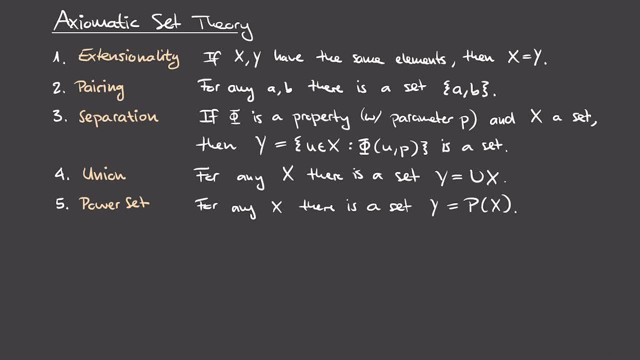 Okay, so axioms 4 and 5 together are necessary because, well, this separation no longer allows us to construct unions and power sets. So far, all of our axioms here, 2 to 5, have been of the form: well, if you have some sets or a set, then you can get some more sets. 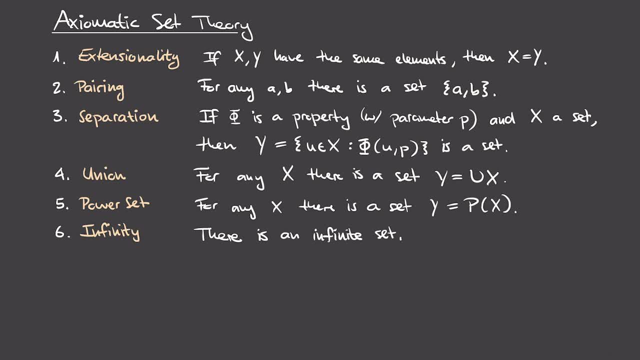 But none of these axioms actually tell us that there are sets at all. Therefore, we need some axiom that tells us that certain sets exist, and axiom 6 does precisely this. It's called the axiom of infinity And it says that there is an infinite set. 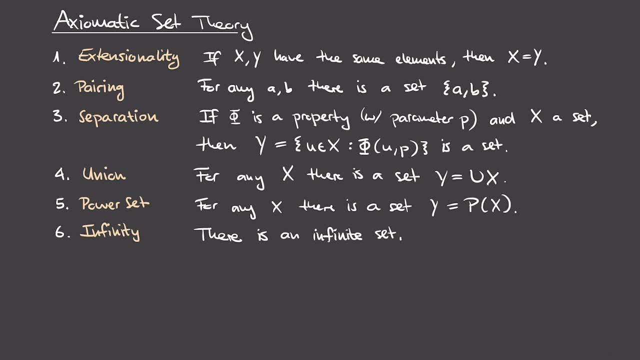 Now, when we go over this axiom in detail, we see exactly how you would define an infinite set. So there's a precise formulation of this, But here you can just imagine that this axiom is stating that there exists some infinite set. In particular, there exists some set. 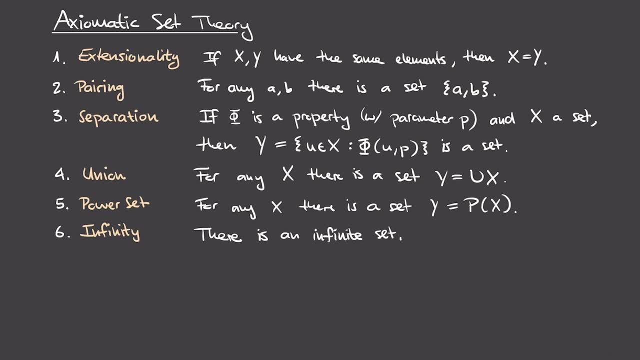 And based on that one can then actually form the empty set using separation. The final three axioms are maybe a bit more complicated. So axiom 7 is called replacement, And it says that if a class f is a function. so here you can just think of f as a function in the sense of assigning elements. 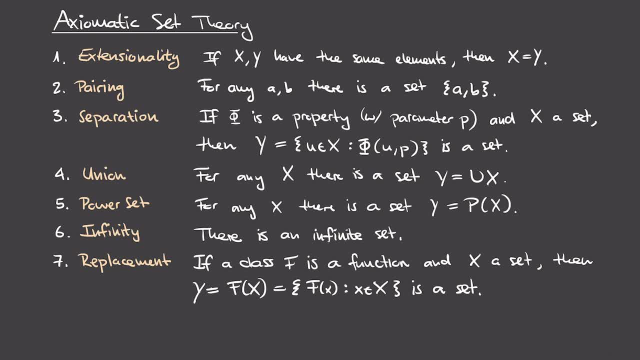 and the domain to elements in the codomain, And moreover x is a set, Then we know by this axiom here that the image of x under this function, f, is also a set. So the image here is all of the image points f of x. 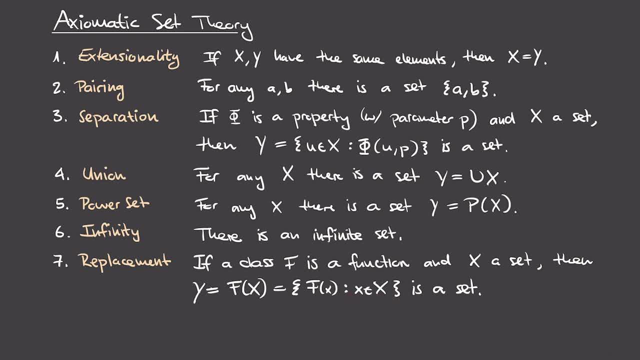 where the points x lie in the set capital X. In other words, this axiom here is telling us that, well, if we have some set we can start out with and we have a function that has that set as a domain, then the image of that function is also a set. 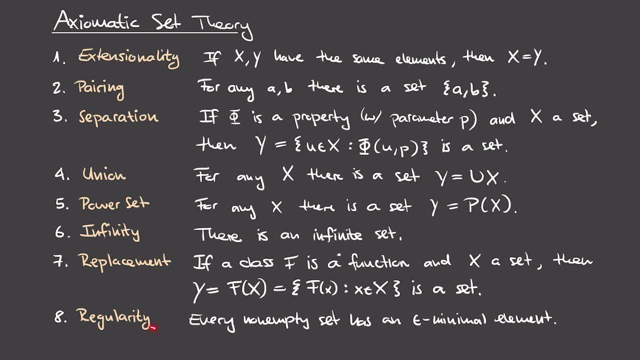 The second-to-last axiom 8 is called regularity, And it ensures that we can't have these paradoxical situations where we can have sets that are an element of themselves. The statement of regularity here says that every non-empty set has an element-minimal element. 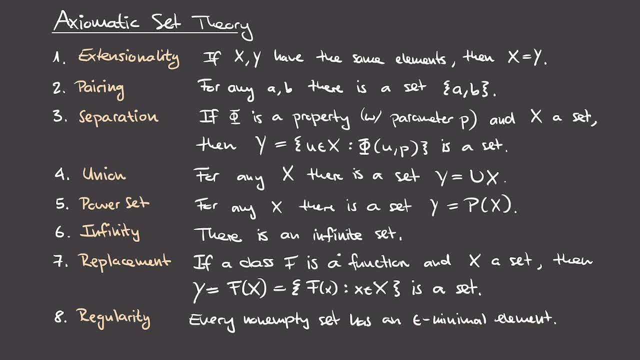 We'll see exactly what this means when we go over this axiom in detail. But, as I said, one consequence of regularity will be that we can't have sets that are elements of themselves. Finally, there's the axiom of choice, which is the last axiom of ZFC. 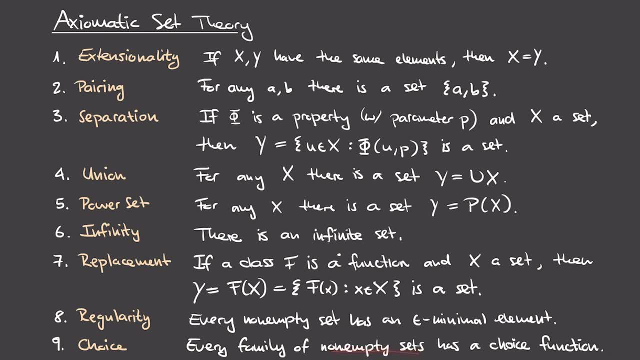 It says that every family of non-empty sets has a choice function Intuitively. what this means is that if we have some family of sets, then, regardless how large this family is, we can choose one element from each set of the family. 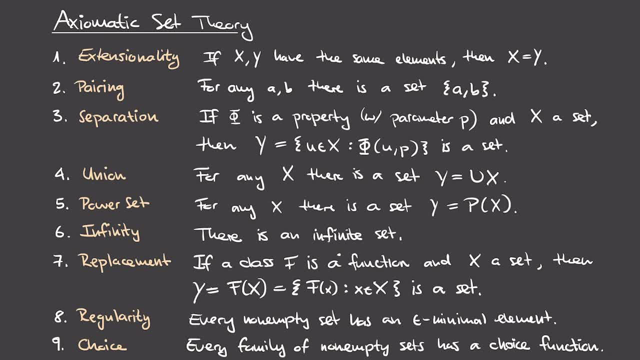 So here you can imagine. the setup is that you have a bunch of bags with things in them And the question is whether you can simultaneously choose one element from each bag, And the axiom of choice is essentially saying that this is always possible, regardless of how many bags you have and what they contain. 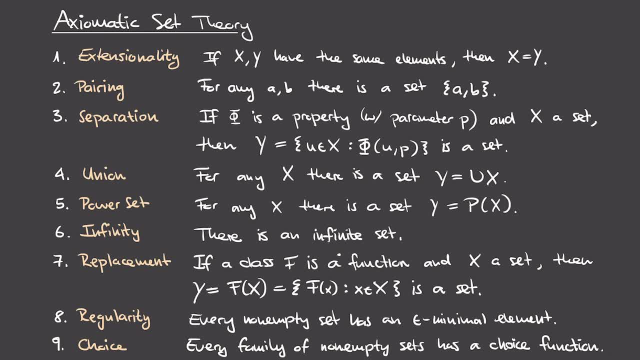 And as such it's a really strong axiom, And we'll discuss a bit what consequences this has. All right, so this concludes the overview of the axioms. So I hope that right now you can see that, while there's quite a few of them, 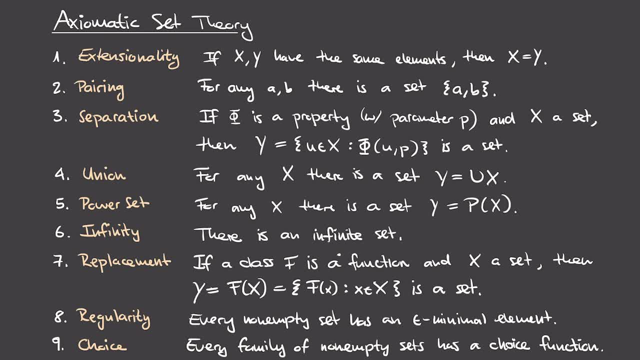 they're not actually so bad, And I hope that you can already start seeing the purpose of each one. In the remainder of the video, we're now going to go through each of these axioms in this order, And in the process, we're also going to build up the basic definitions. 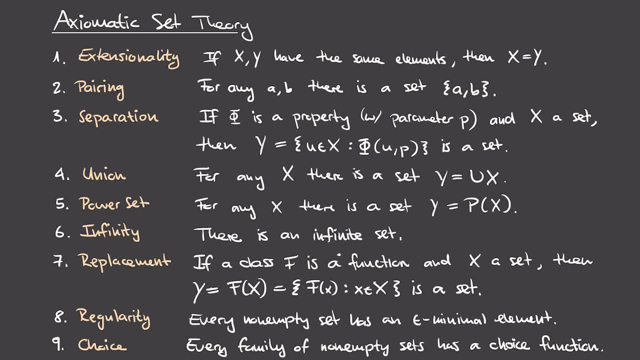 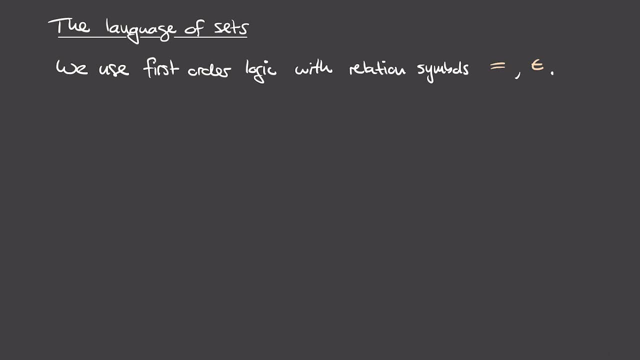 of set theory based on these axioms. By the end of the video we'll actually have basically all of the foundations necessary to start doing usual mathematics using this axiomatic foundation of set theory. We're going to start by taking a step back and talking about the formal language. 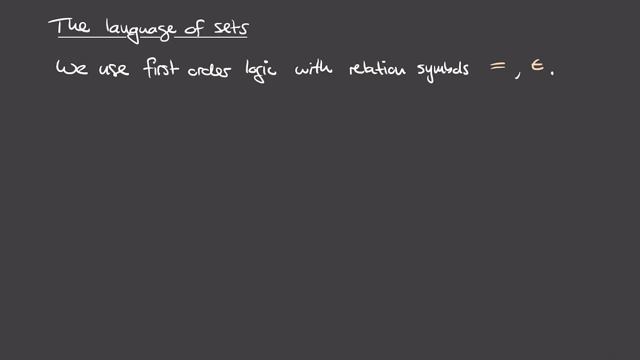 that we'll be using to talk about set theory. As I mentioned previously, the language of set theory will basically be first-order logic, but we have this additional relation symbol for being an element. So the two ways that we can compare sets are going to be to use equality. 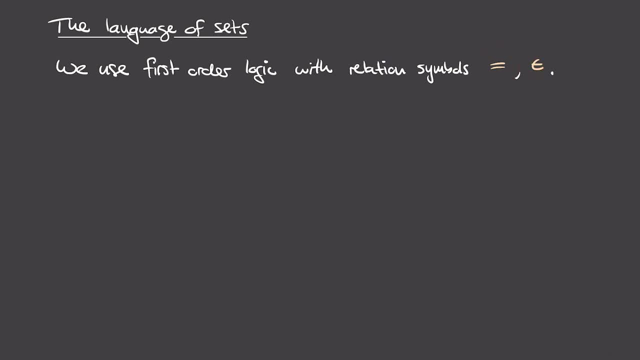 and also being an element. So these are the basic relations that we can have between sets. Moreover, all of our variables that we'll be using will represent sets. So, in this axiomatic version of set theory, every object that we consider will be itself a set, and then we'll have some sets being elements of other sets. 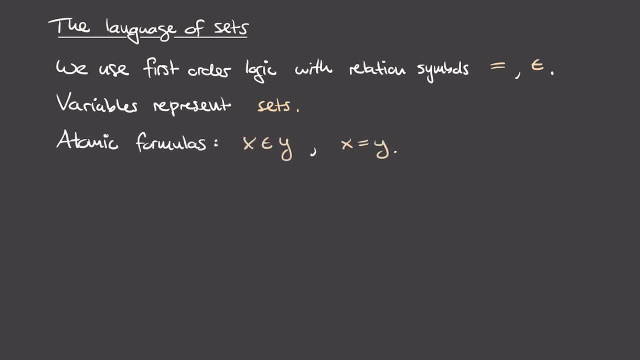 and so on. Now, using these relation symbols, here we get the following form for atomic formulas. So atomic formulas are either of the form: x is an element of y or x is equal to y. And well then, based on these atomic formulas, we can use the usual. 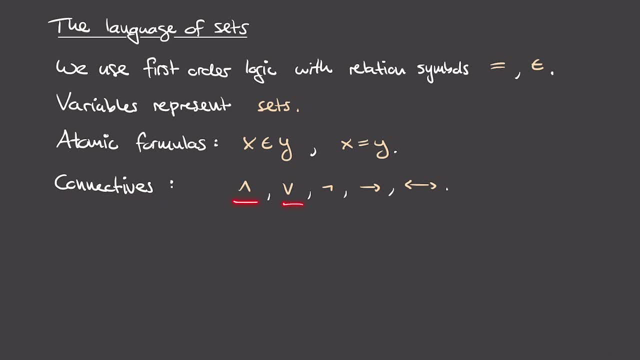 logical connectives here. so that's conjunction, disjunction, negation, implication and equivalence, in order to build up more complicated formulas that allow us to state various properties. Because we're in first-order logic, we also allow for the use of quantifiers. 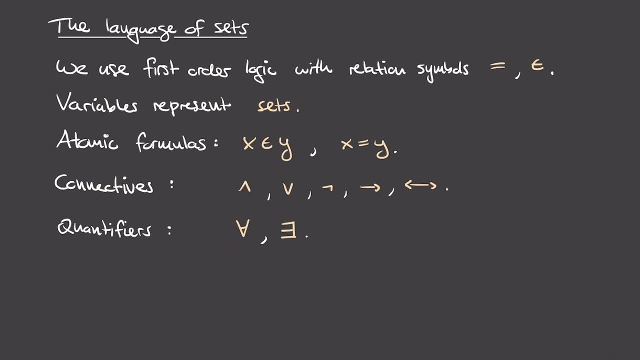 so we'll have the universal and existential quantifiers as well. Finally, we introduce some notation for formulas. So we write phi of u1 up through un When phi is some formula, and moreover, all the free variables in phi occur among these variables: u1 through un. 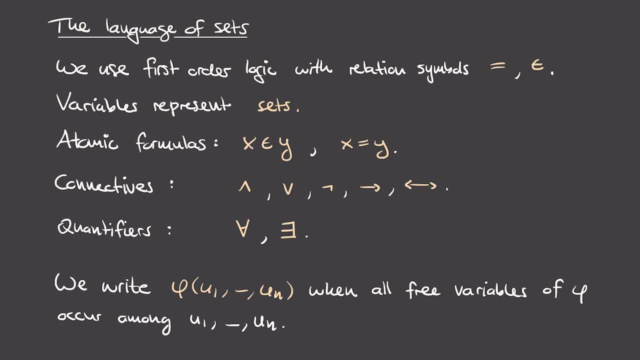 Remember from the video on first-order logic that a variable is free if it's not bound by one of these quantifiers. The significance of these free variables is that, depending on what object you insert for the free variables, the truth value of your formula might change. 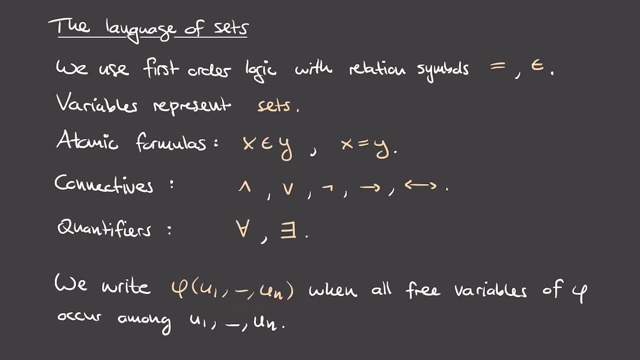 Therefore we have this notation here that says that, well, if we write it like this, so phi of u1 through un, then it means that all of the free variables that occur in phi are among these variables that we put in the parentheses after the formula. 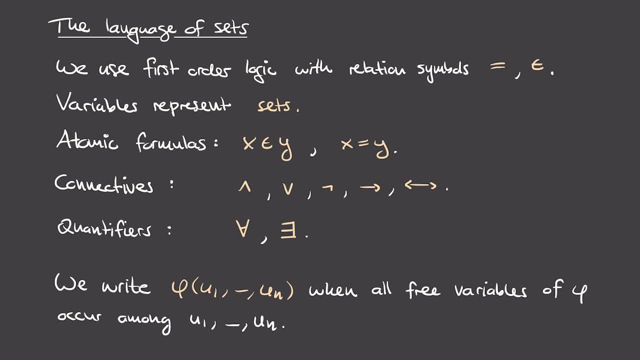 Now notice that here I'm just saying that the free variables occur among these, so in fact I could put additional variables here that don't occur as free variables in the formula. but the important thing is that all the free variables that in fact 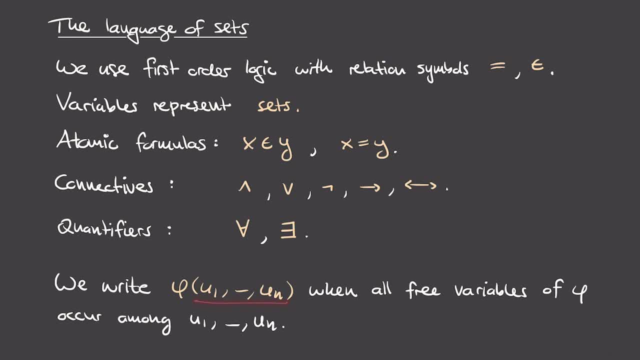 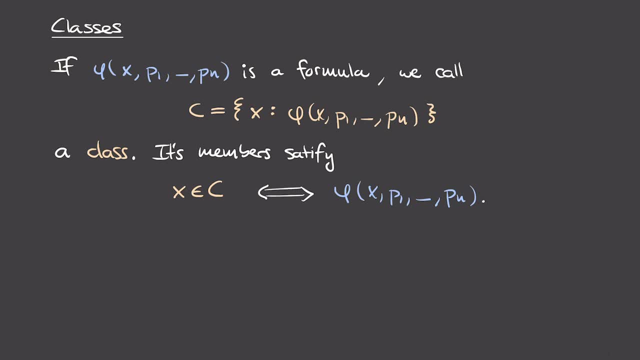 do occur in the formula also appear in this list. The second preliminary thing we'll introduce are called classes, and essentially classes just give us a convenient way to talk about formulas Now in some versions of axiomatic set theory, but not in ZFC. 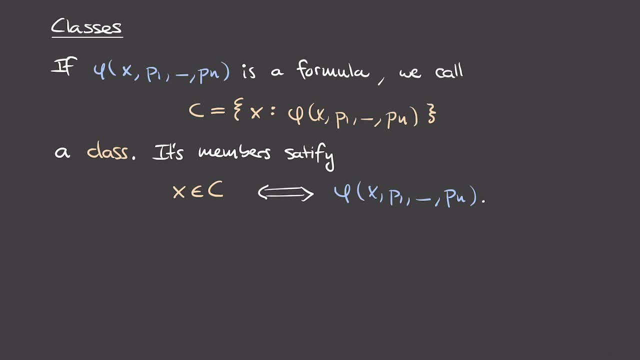 classes actually form objects in the theory, but here classes will just be sort of an informal way of talking about formulas in a more convenient manner. In fact, classes will sort of realize this unrestricted version of comprehension that we had in naive set theory, and then, well, we'll be arguing that certain classes are in fact sets. 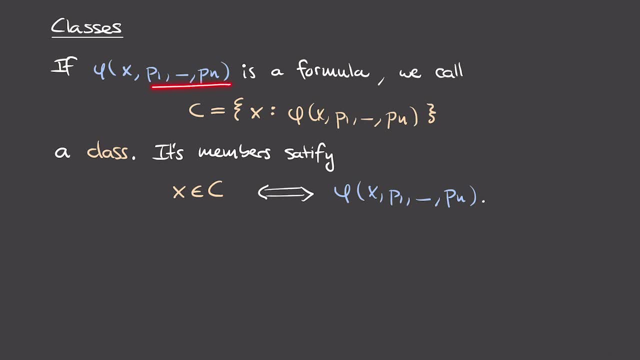 So in order to define a class, you need some formula. so here let phi be a formula which depends possibly on x and on p1 up through pn. Well then we call the following comprehension a class. so this is the well class of all x that satisfy this formula. 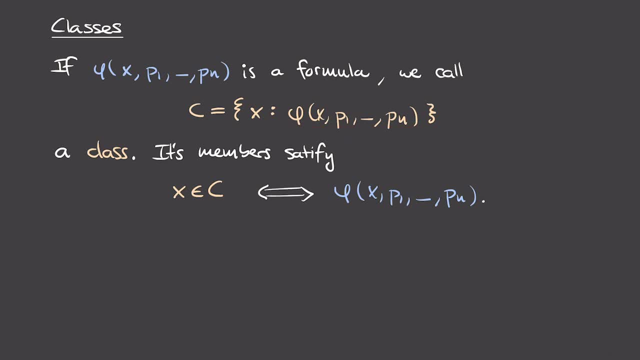 phi of x and p1 up through pn. So x is a member of C. so it is an element of C if and only if. well, this formula holds for x. Now, because of this expression, the equivalence here, it means that classes are completely determined. 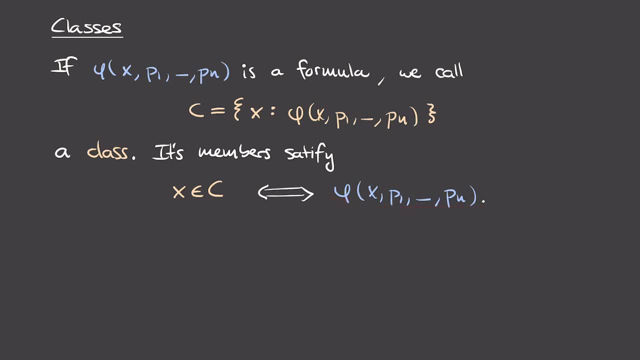 by the formula that defines them, and in this sense classes are just another way to talk about logical formulas. but it's convenient because classes somehow look like a set comprehension. As is the case for sets, two classes will be considered equal if they have precisely the same elements. 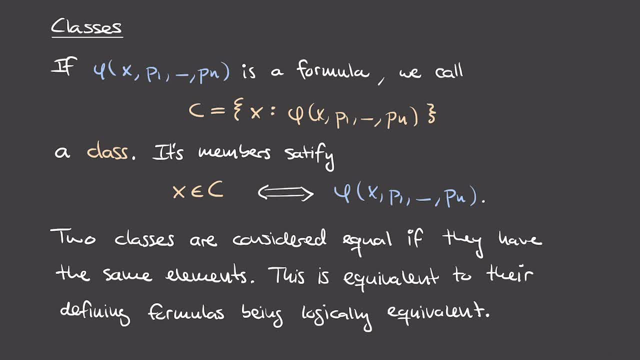 In fact, because of the way we've defined classes in terms of their elements being precisely those that satisfy this formula, it means that two classes are, in fact, equal precisely when their defining formulas are logically equivalent to one another. This is again compatible with the idea that classes are just ways of talking about formulas. 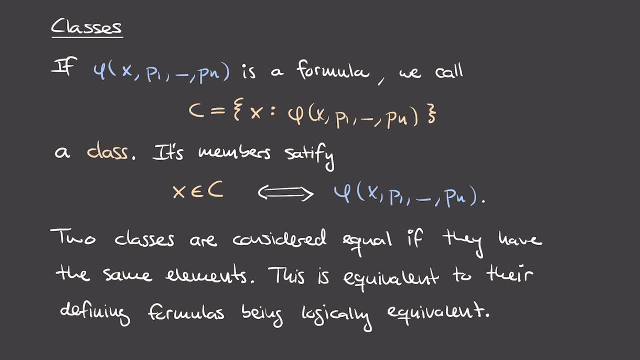 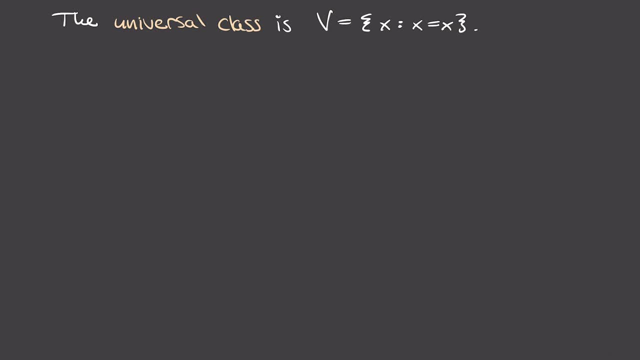 because, well, equality of classes is just logical equivalence of formulas. Now, because we don't put any restriction on the formulas that define classes, we can, for example, define this universal class, so this is all the x, such that x is equal to x. 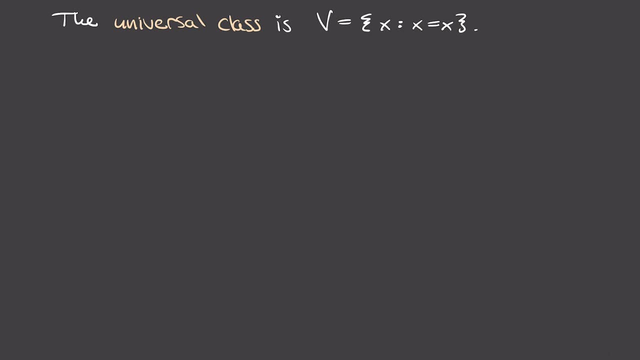 and this is in fact like the class of all sets, because all sets satisfy this formula here. Next we can define inclusion for classes. so a class C is included in a class D. if well, all elements x in C are also elements x in D. 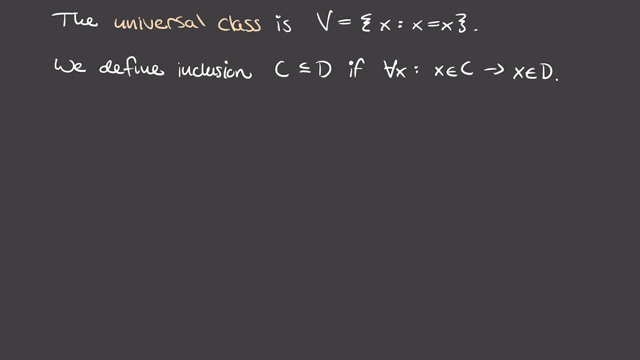 Now, if you think about this in terms of values, the defining formulas of C and D. this is just saying that for any choice of x, the defining formula of C, with that fixed x, implies the defining formula of D. We can also transfer the definitions we had. 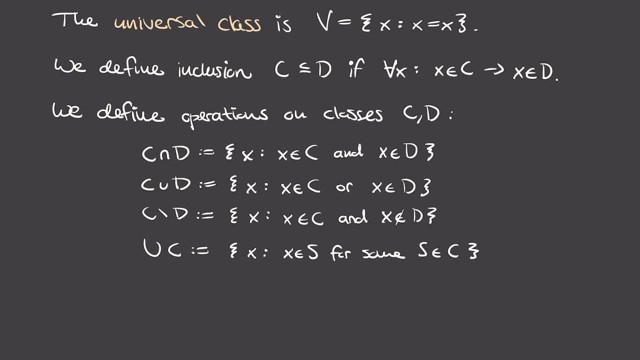 for the set theoretic operations in the last video to classes, because these classes are essentially this unrestricted comprehension we introduced there. So we can define the intersection of two classes, C and D, to be all the elements that occur in C and in D. 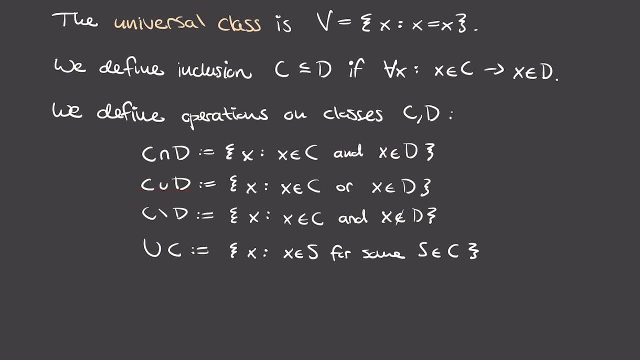 We can define the union of two classes to be all elements x, such that x lies in C or x lies in D. We can define the difference between two classes as being all those x that lie in C but do not lie in D. And finally, we can define a big union over a class C. 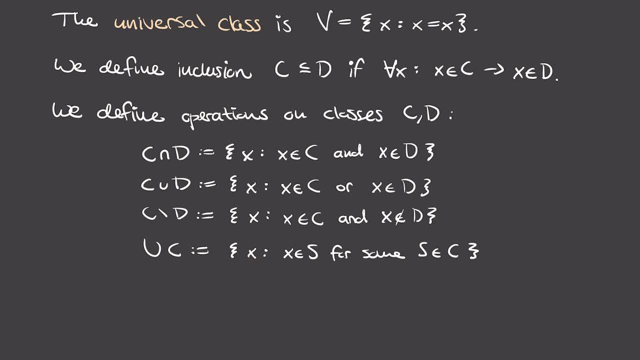 to be all the x, such that x occurs in an S for some S occurring in C. So this last definition is not something we saw in the last video and is maybe a bit confusing. So here we think of C as being some sort of collection, S1, S2, and so on. 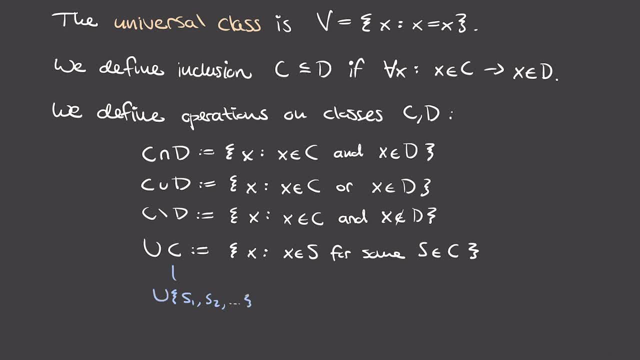 And now, if we take the union over all of these S's, well, this is just. you need to think about this as being somehow the union of S1, S2, and so on. So the union over this C, which is like a family of S. 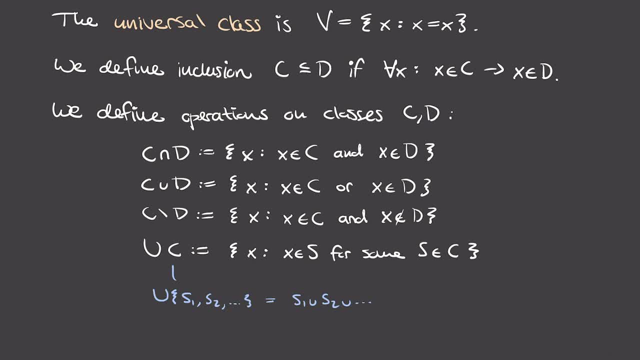 classes. S's is just all the elements that occur in at least one of these S's here. That's exactly what this definition is saying. So it's all the elements x, such that x lies in one of the S's. for some S, that's an element of C. 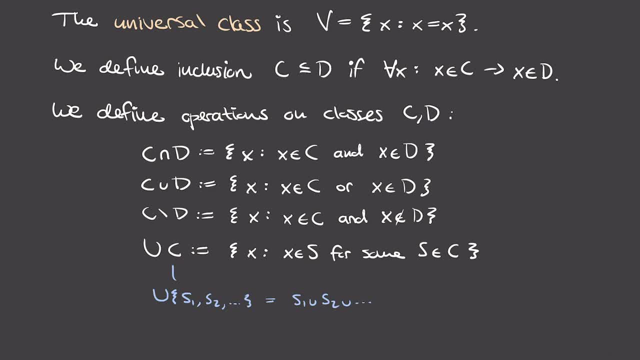 So here C has the role of being like a family of classes, S, which we're unioning together. Finally, we can note that every set S is in fact a class and it's defined by the following formula: So it's defined by being all the elements x, such that x is an element of S. 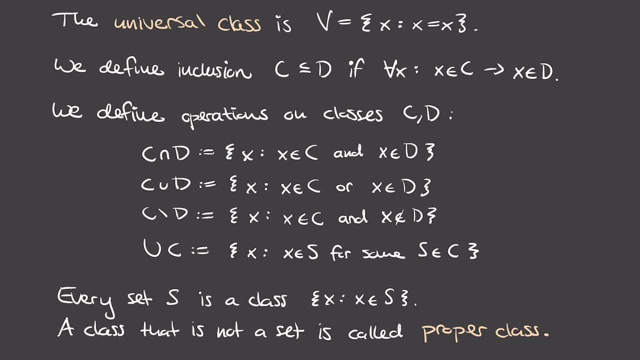 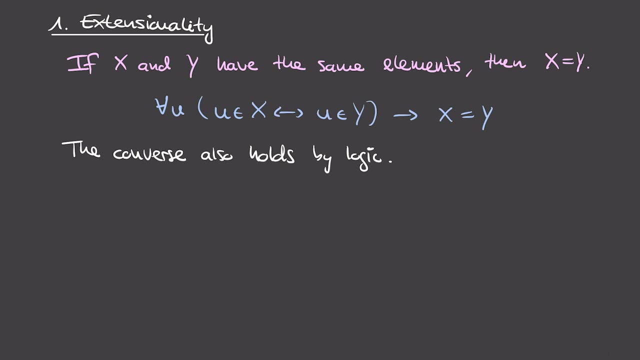 On the other hand, there are classes that are not sets. For instance, this universal class here is not a set, and such classes will be called proper classes. So to get that background out of the way, we can now turn to the first ZFC axiom. 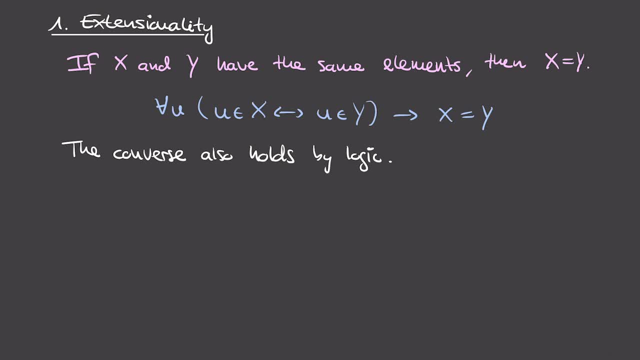 which is extensionality. Remember that extensionality defines what it means for two sets to be equal. So here's the statement in words. So if x and y are sets that have the same elements, then in fact x is equal to y. Now all of the axioms in ZFC. 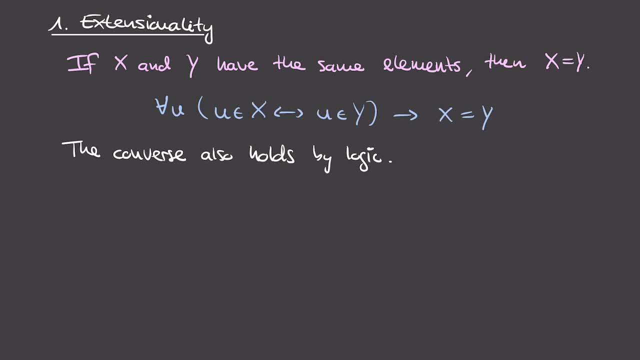 are actually formulated in first order logic. So this description here in words is really just a description of the corresponding first order logic formula down here that I've written in blue. So this formula here says that for all elements u, if u is an element of x. 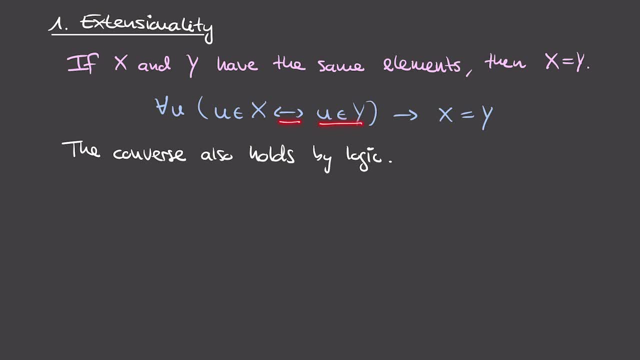 if, and only if, u is an element of y, then this implies that, in fact, x is equal to y. In other words, if every element of x is an element of y and, conversely, every element of y is an element of x, 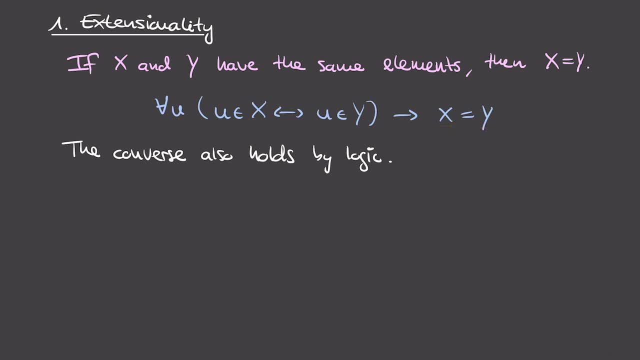 then in fact x is equal to y. So I personally remember these types of definitions based on the statement in words. However, here it's maybe not exactly clear what it means for two sets to have the same elements, and that's made perfectly precise. 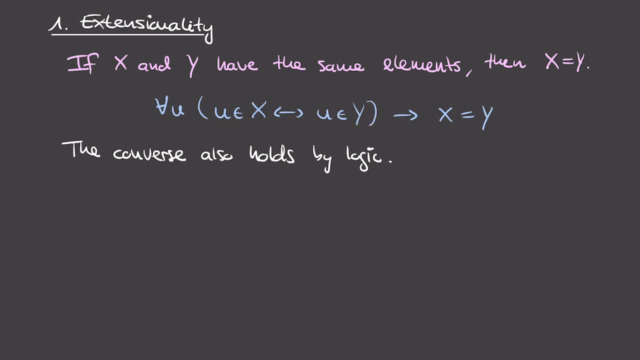 in the first order logic formula. here, As a side remark, the converse of this implication here also holds by logic. So if two things are equal, well then they have exactly the same properties. in particular, they will share the same elements here. 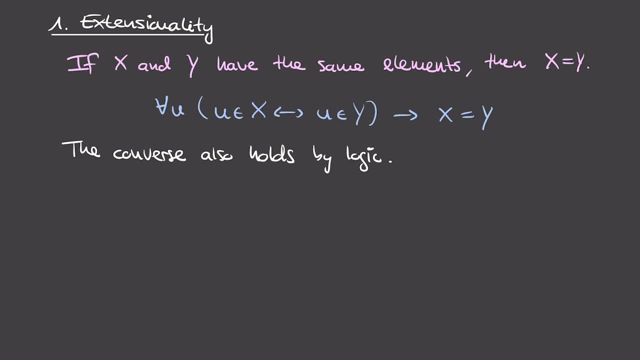 So if we wanted to, we could actually strengthen this axiom here to have this be an equivalence. So two sets are equal precisely when they have the same elements. but this is not really necessary to add as an axiom to ZFC because it already follows just by logic. 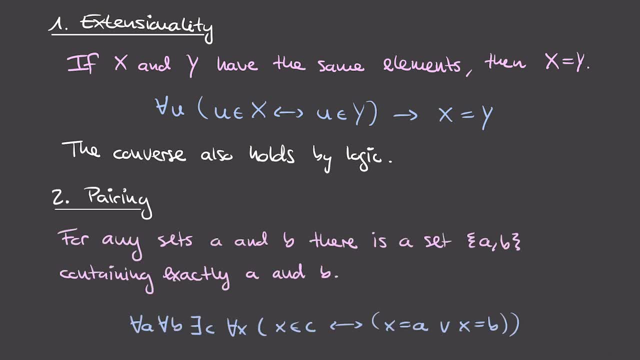 We now move on to the second axiom, which is called pairing. So it says that for any sets a and b, there is a set containing exactly those two sets, a and b. The first order logic version of this statement is as follows: So it's the formula down here. 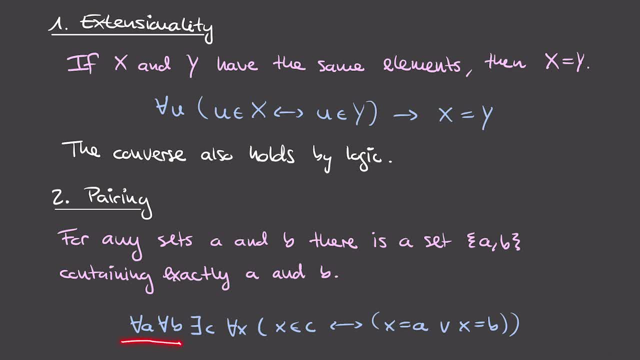 It says that for all a and for all b. so these are the sets we're interested in. there exists a set C, so that's the set we're trying to build such that well, for all elements x. x is an element of C. 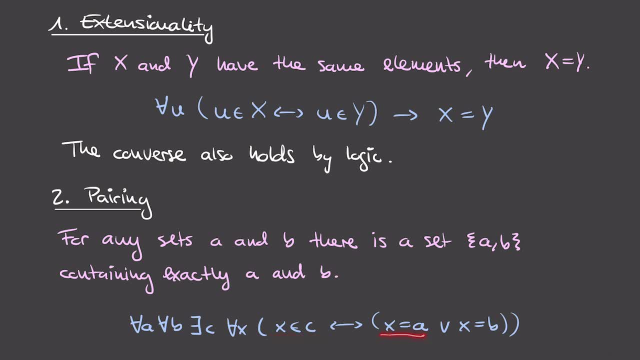 precisely when x is either a or b. Alright, so you need to think about this C as being this set containing exactly a and b, and this condition here is saying that, well, the elements of C, so the elements x of C. 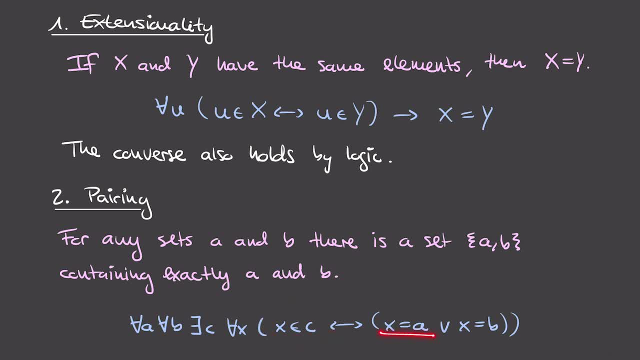 are precisely either a or b, So x is an element of C if, and only if, x is equal to a or b. Therefore x is equal to b. We'll see this type of pattern here cropping up a lot, so it allows us to define exactly what the elements of a set are. 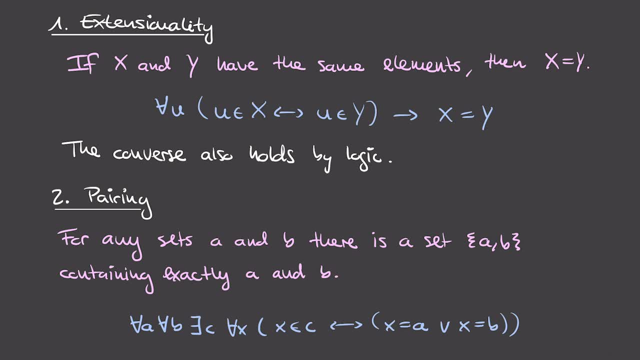 because you just say, well, for all sets, x, x is an element of this set. you're trying to define if, and only if, some condition holds, and that condition defines the elements of the set in question. Moreover, whenever we define a set using the previous pattern, 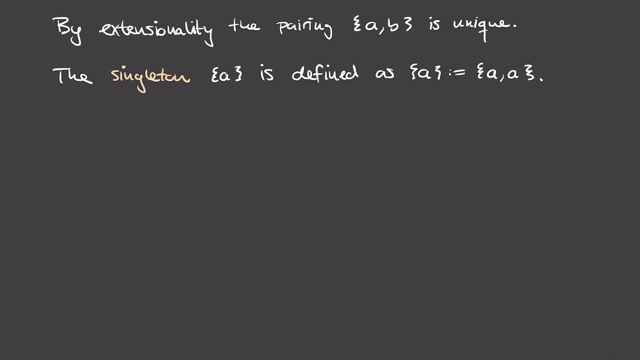 it'll be unique because we're essentially saying exactly what the elements of that set are and therefore any other set that satisfies this property, namely that we exactly specify what its elements are, will be the same. So, by the extensionality axiom, this pairing set containing a and b will be unique. 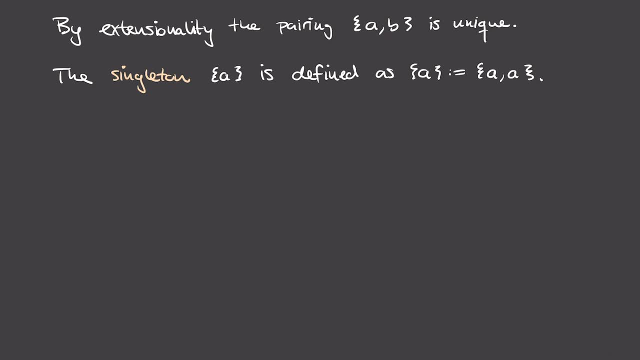 and therefore it makes sense to adopt this notation here. Based on this pairing axiom, we can actually start building up some interesting sets. So the first interesting set that we can define are singleton sets. So the singleton here, so that's a set just containing a. 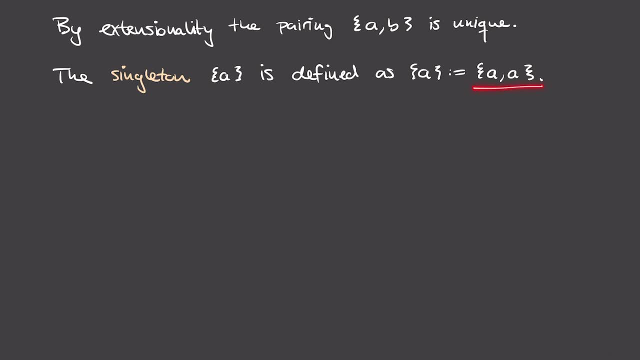 will just be defined as the pairing of 2 times the set a. So if you choose a to be equal to b in the pairing axiom, then you basically just get singleton sets. Perhaps, more interestingly, we can use the pairing axiom to define ordered pairs of sets. 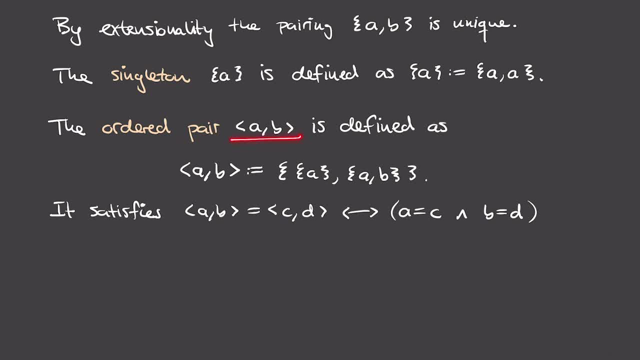 So the ordered pair a- b in these pointy brackets is defined as follows. So we define this ordered pair in the following way. So first we take the singleton containing the set a and then we take the pairing of the sets a and b. 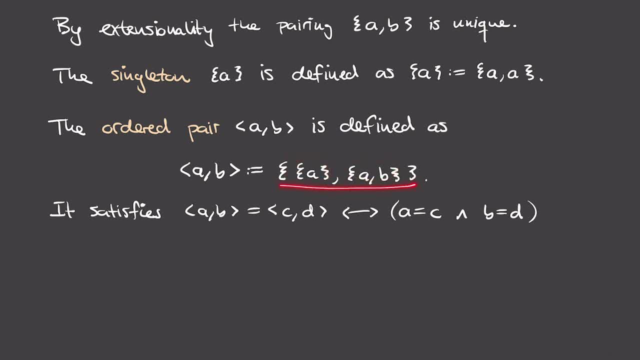 and we pair these sets together in a larger set, like so. Now, at first glance it might not be entirely clear what this is doing, but in fact, what we want from this ordered pair is the characteristic property of the ordered pair that I introduced in the last video on the set theory. 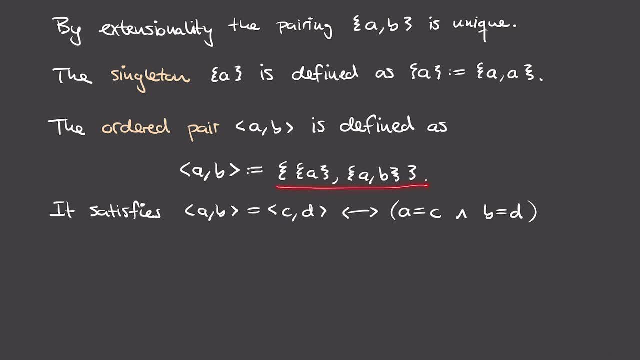 And in fact, if you define the ordered pair in this way, that characteristic property holds. So the property states that 2 pairs, so a, b and c, d, should be equal, precisely when the first components of the ordered pairs are the same and also the second components of the ordered pairs are the same. 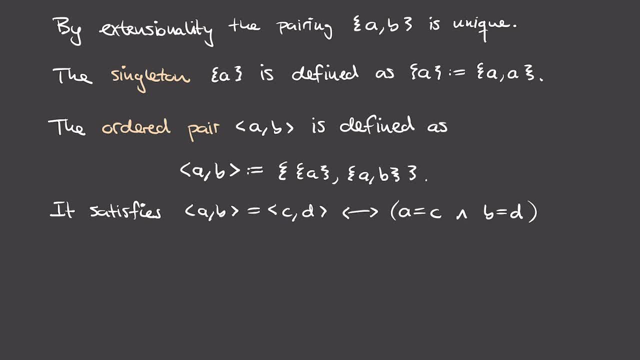 Hence this construction here. using sets allows you to realize ordered pairs as certain types of sets. Now, as an exercise, you could think about how to prove this property here, based on the definition of an ordered pair. Finally, once we have ordered pairs, we can extend ordered pairs to arbitrary n-tuples. 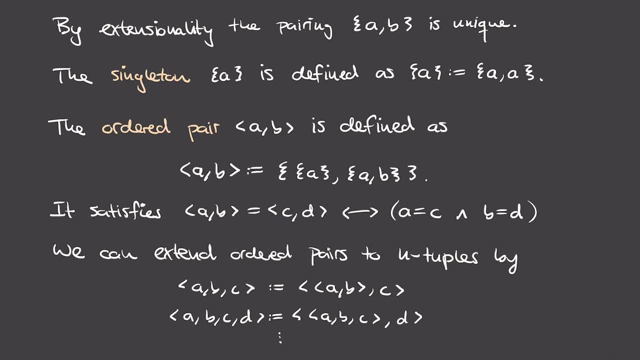 by just iterating the ordered pairing. For instance, if you want to have a 3-tuple like this, well then, you first just take the ordered pair of a with b, and then you pair that with c, And in a similar manner you can just iterate this. 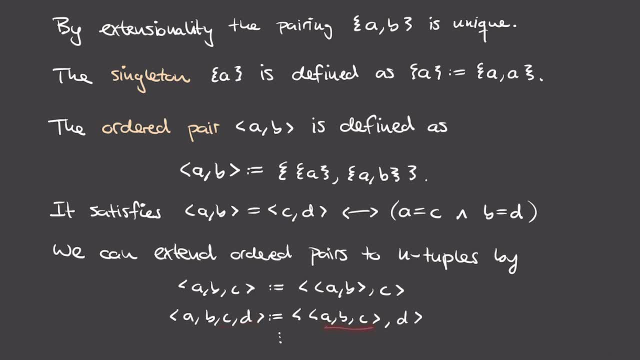 So if you want 4-tuples, then you pair a 3-tuple with an additional element, and so on. If you use this construction method, then in fact this characteristic property of the ordered pair somehow transfers to n-tuples. So in fact you can prove that 2 n-tuples are the same. 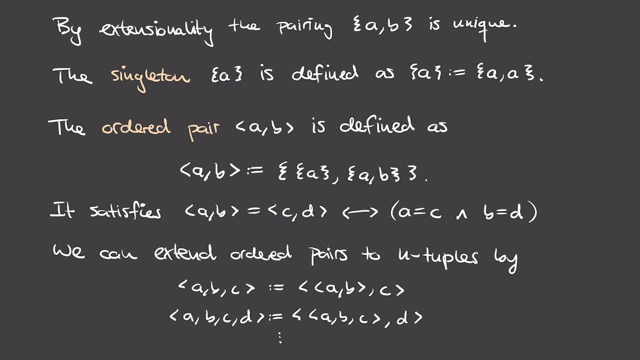 precisely when each of their entries at the corresponding position are the same. Okay, so from the first two axioms, so from just extensionality and pairing, we can already construct quite a few interesting objects, in this case ordered pairs and n-tuples. 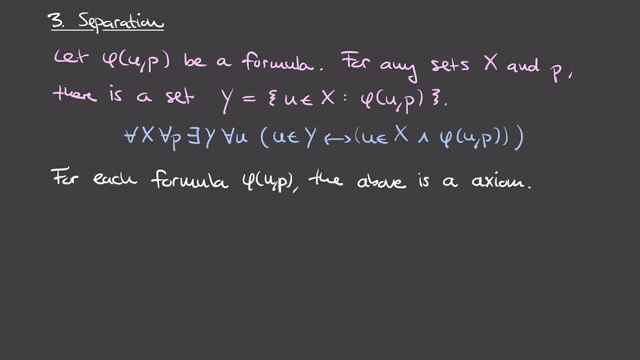 We now move on to the third axiom, which is separation, And, as I have said multiple times, separation is a weaker form of the set comprehension principle we saw in the last video. The statement of the separation axiom in words is as follows: So we let the phi be a sum. 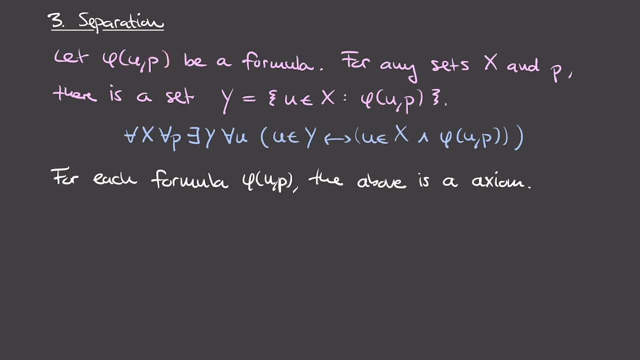 which might have three variables, u and p. And then, for any set x and any set p, there is a set which consists of all the elements u and x that satisfy this formula phi. In other words, the separation axiom allows us to filter the elements of x based on this formula phi. 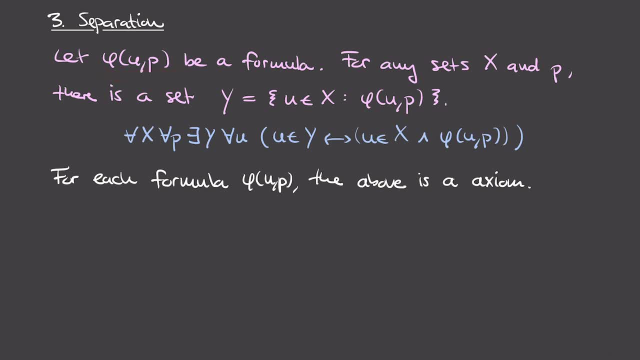 Moreover, this formula here also has a parameter p, which we can vary if we wanted to. Now, in first order logic, the separation axiom is phrased as follows: So it says: for all sets x. so that's the set we want to filter. 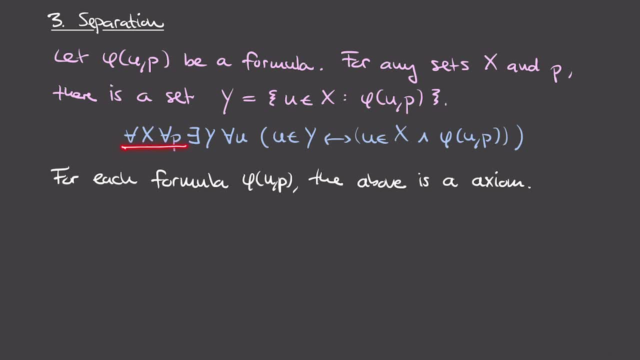 and for all p, so that's the parameter value we're setting. there exists some set y, so that will be this filtered set, such that, well, the following property holds, namely that for all elements u, u is an element of y. 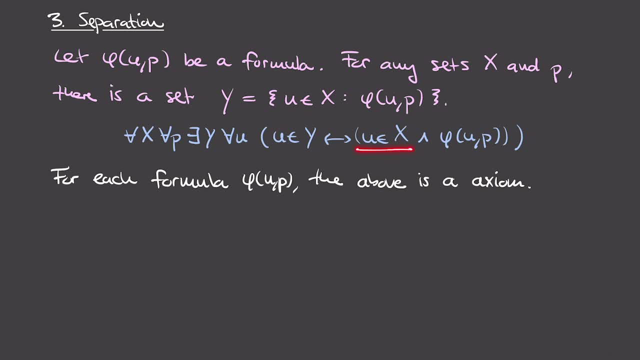 if, and only if, on the one hand u should lie in x, on the other hand u should satisfy this formula phi, with the parameter p fixed. as we did Here, you can again see this pattern which we saw previously in the pairing axiom. So this defines what the elements of the set y are. 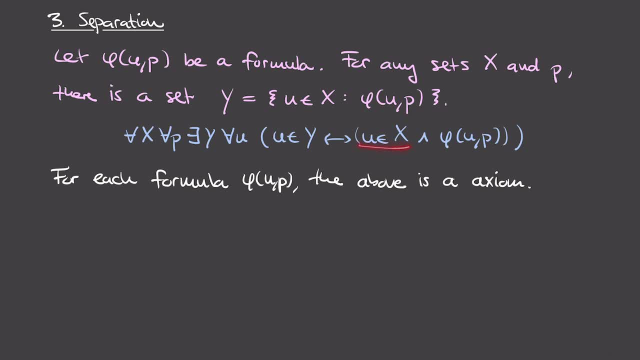 Well, elements of the set y are precisely those elements of x that satisfy this formula here. Now, in contrast to the previous two axioms, the axiom of separation is actually an infinite number of axioms. It's a so-called axiom schema, because for each formula, phi of u, p, 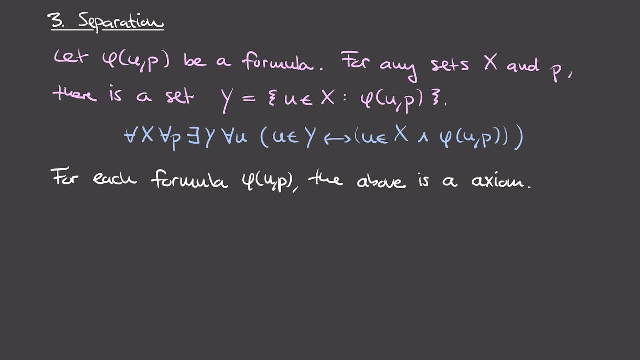 we have such an axiom. So you see here that in the formula phi is like fixed. so for each formula we need to have such an axiom in order to use separation. Notice that in this original formulation of separation, the formula that we give the separation axiom 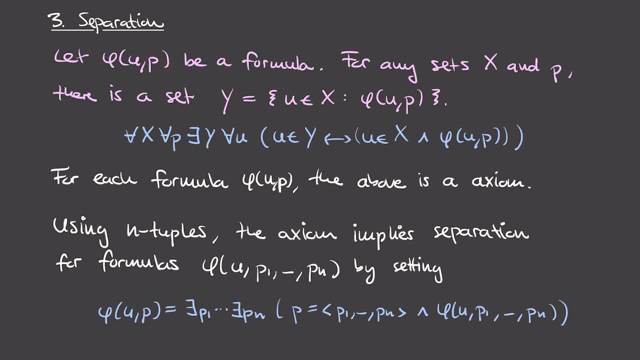 can only depend on one parameter. However, using n-tuples, we can actually extend this type of axiom to be able to accept several parameters, p1 up through pn. The way to do this is well, you start with a formula phi that possibly depends on multiple parameters. 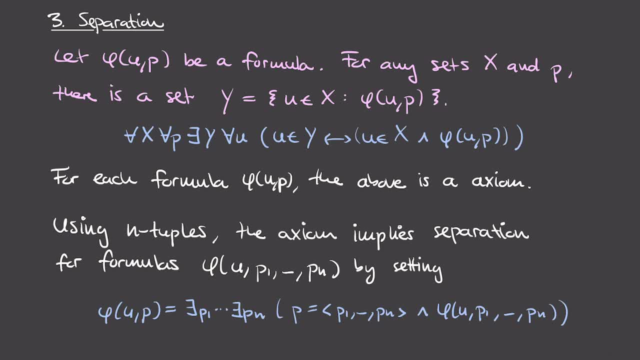 and then you let this phi of u p occurring in the axiom of separation be the following formula: So here you need to think of this p as now being an n-tuple of the parameters p1 up through pn, and so the formula you write is the following: 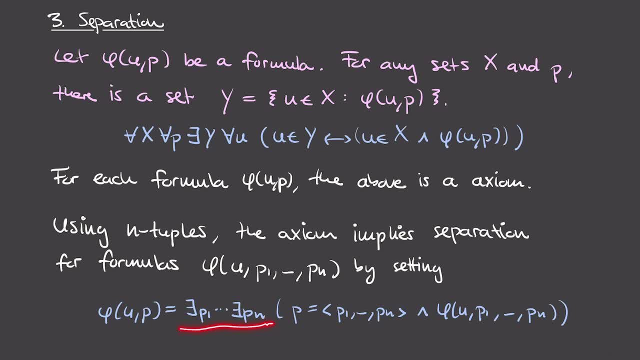 So you write: there exists p1 up through there exists pn, such that on the one hand, this parameter p is precisely the n-tuple of p1 up through pn, and also this formula with the several parameters phi of u, p1 up through pn holds: 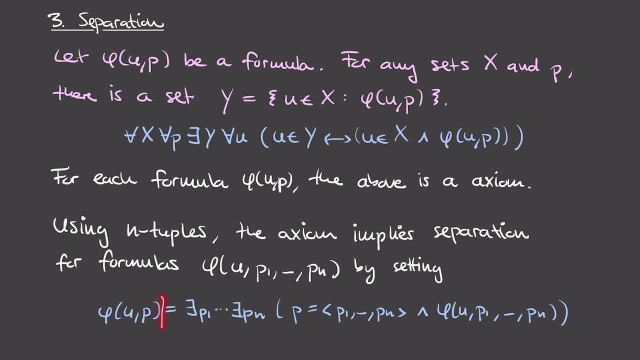 So essentially what you're doing is you're feeding this formula phi here in n-tuple p and you're then unpacking this n-tuple using this there exists, and so on, such that p is equal to p1 up through pn. so that's essentially like unpacking each of the components in the n-tuple. 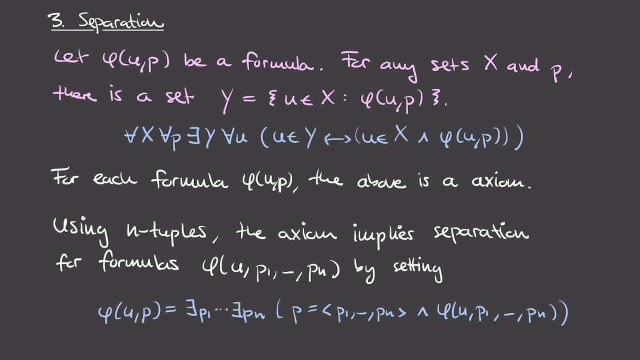 and then you're using this unpacked n-tuple, so the parameters p1 up through pn, to check the original condition you had, which depended on several parameters. Alright, so this is perhaps not the easiest thing to follow. You should probably go through it on your own again. 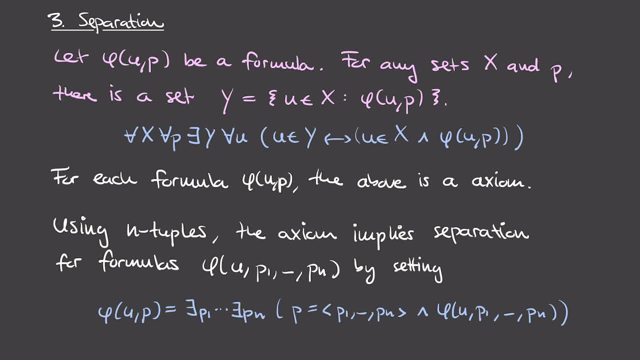 if you want to understand what's going on here. The reason I'm mentioning it here is because, in what follows, we'll actually be using the axiom of separation with several parameters as well, and the reason this is okay is because of this argument that I just presented. 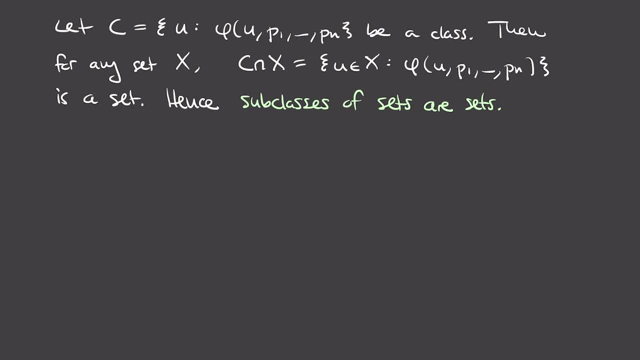 Now, one way to think about the axiom of separation is saying that subclasses of sets are again sets. So basically, classes are defined in terms of formulas. and well, if we filter a set based on a formula, that would be like a subclass. 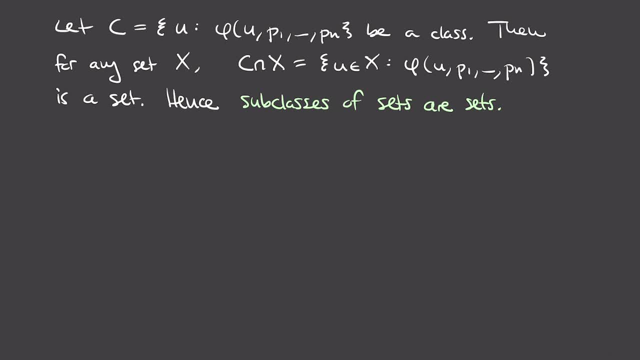 and the axiom of separation is telling us that those things are again sets. This idea is useful in the following manner: So suppose you have some class c, which is all elements u, that satisfies some property phi and that depends on some parameters. So if this is a class, 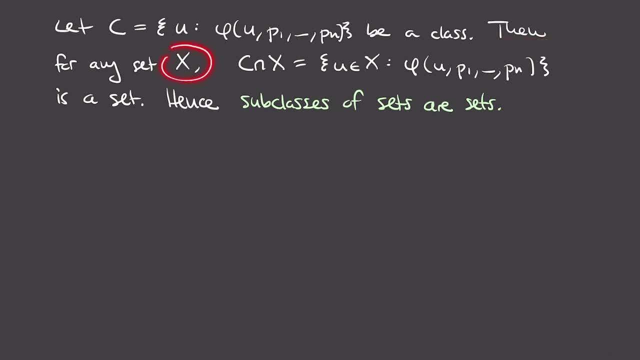 then, well, if you take any set x and consider the intersection of x with c, well then that will consist exactly of the elements u and x, such that this property holds Now, by the separation axiom. this is a set and therefore, if you intersect any class with a set, 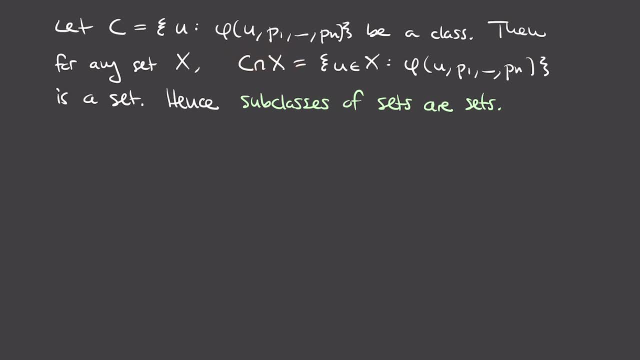 what you get is a set. Another way of saying the same thing is that: well, if c is in fact a subclass of a set x, well then this implies that, well, c intersection x is just equal to c, right? 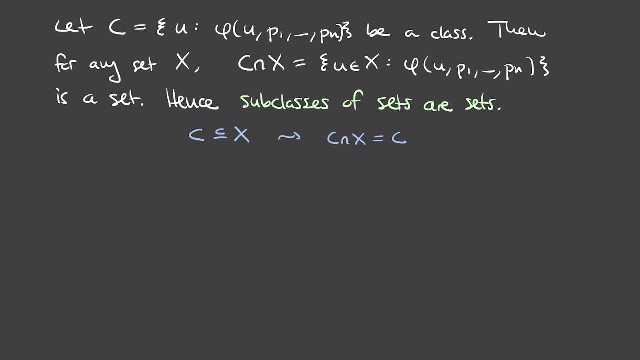 because every element in c is also in x. so the elements that c and x have in common are just the elements of c. And well, we saw above that if x here is a set and this is just a general class for the moment, 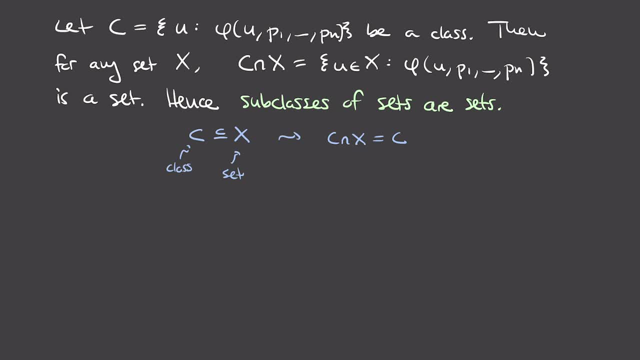 well, we saw that this intersection here, by separation, this will again be a set And hence, because this intersection is equal to c, we now can conclude that c is also a set. Therefore, whenever we define a class and can show that it's in fact a subclass of some existing set, 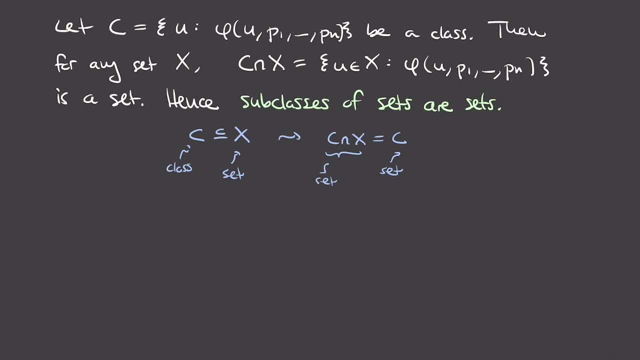 then we can conclude that that class is itself a set as well. In fact, this is how we'll usually be using the separation axiom, so we won't be applying it directly. Rather, we'll just be arguing that certain classes which we define in terms of formulas, 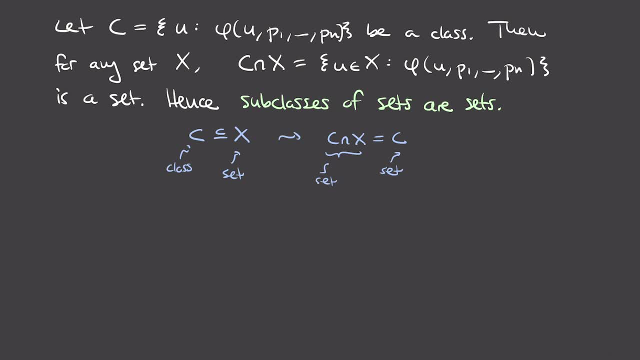 are sets because they are a subclass of some larger set. For instance, we can use this type of argument to now show that certain operations we defined on classes also work for sets. For example, consider the intersection. So the intersection of two classes, x and y. 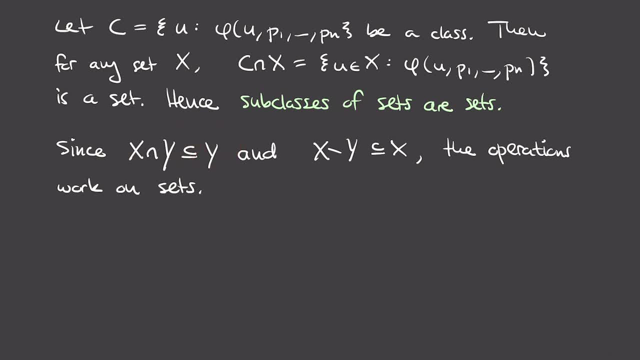 is a subclass of y And therefore, if we assume now that x and y are sets, well then this thing here on the left is a subclass of the set And therefore this is also a set, And this shows that the intersection between two sets is again a set. 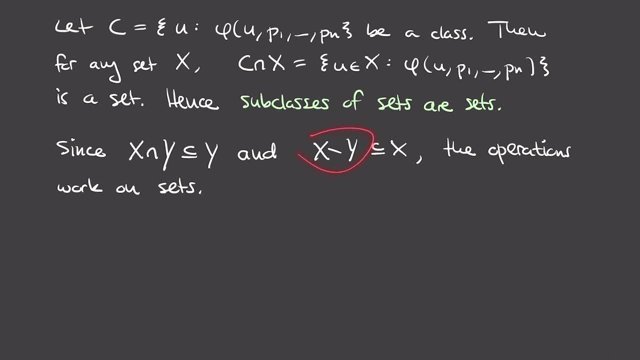 A similar argument works for a set difference. So the difference x minus y is a subclass of x And therefore if both x and y are sets, well, then also the difference between them will be a set. On the other hand, this type of argument doesn't work. 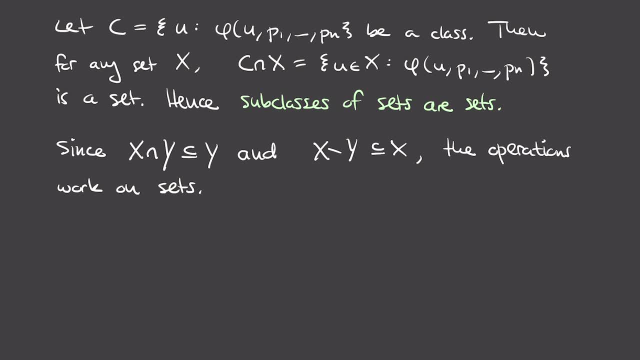 for things like unions and power sets, because those operations give us bigger objects that aren't like a subclass of some preexisting set we can define. Hence we'll have to have axioms that tell us that unions and power sets are in fact sets. 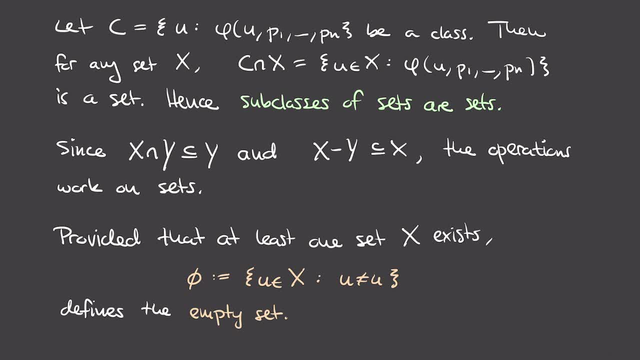 We can also use separation to define the empty set. So, provided that at least one set x exists, we can define the empty set using separation. Namely, we define it to be all the elements u in this set x, such that u is not equal to u. 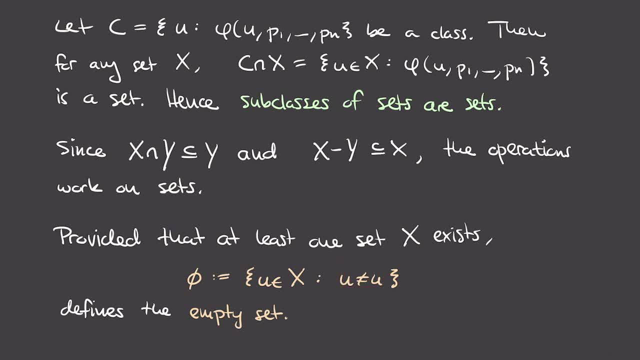 Now, because there are no elements u that are not equal to themselves. this means that the set you get by well applying this condition to all elements in x will in fact be empty. So this is one way of defining the empty set. 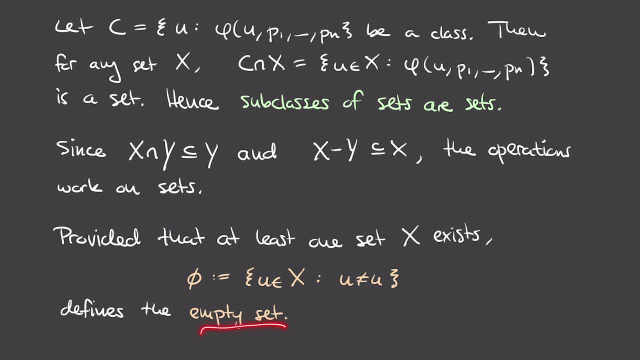 Moreover, by extensionality, the empty set is unique because, well, if you take any other empty set, so a set that doesn't have any elements, it'll have exactly the same elements as any other empty set. Now, so far we don't actually have enough axioms. 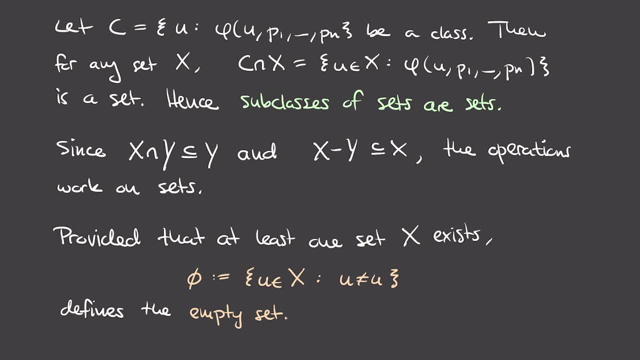 to really conclude yet that the empty set exists. We only know that if there is some set x. so if there is at least one set that exists, then we can form the empty set, and so then the empty set would also exist Now using the empty set. 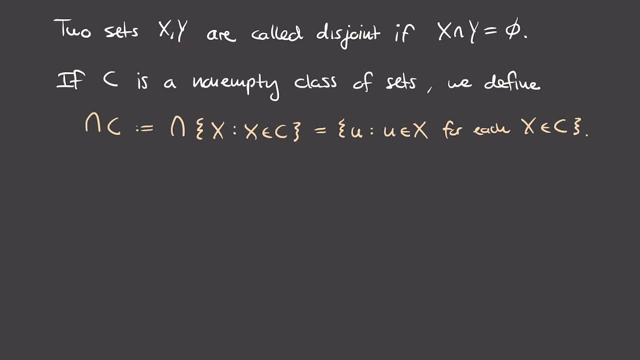 we can say what it means for two sets to be disjoint. So two sets, x and y, are called disjoint if their intersection is the empty set. Finally, we can extend the idea of intersection over families of sets, So if c is some non-empty class of sets. 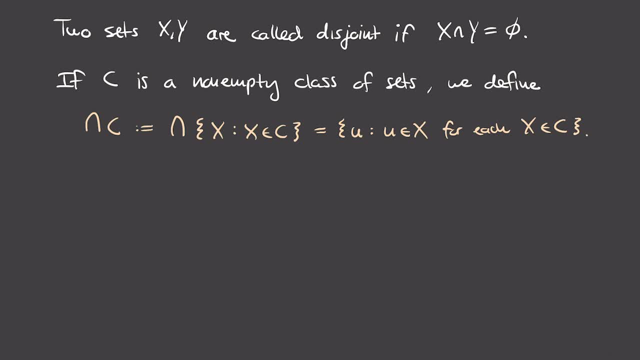 so you have to think about c as being like a collection of sets. then we can define the intersection over c. So this is just the intersection over all sets x that occur in the collection c and it consists of all elements u, such that u is an element of each of the sets x in the collection. 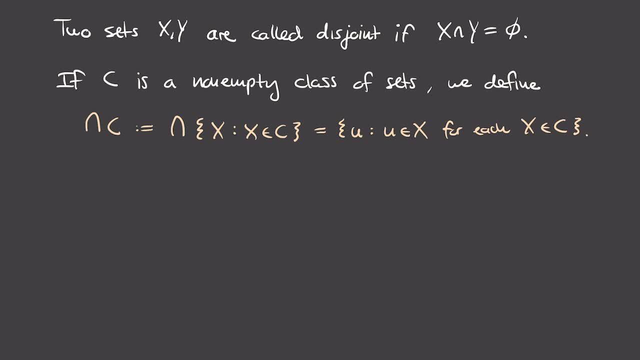 So this is just a generalized version of the intersection that can work also for possibly infinite collections of sets. Now, because this intersection here will be a subclass of any of the x's occurring in it and, moreover, we assume that those x's are sets. 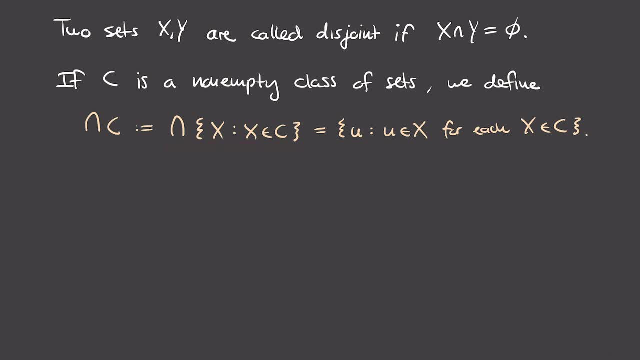 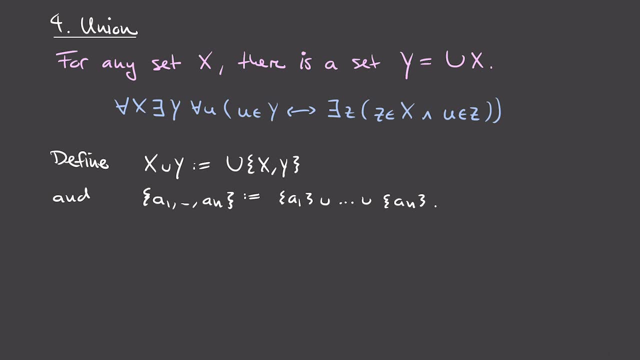 it means that, in fact, this intersection will also be a set. Okay, so we've seen that using just separation we can define the operation. We can define the operations of intersection and set difference. But, as I mentioned, for unions and power sets. 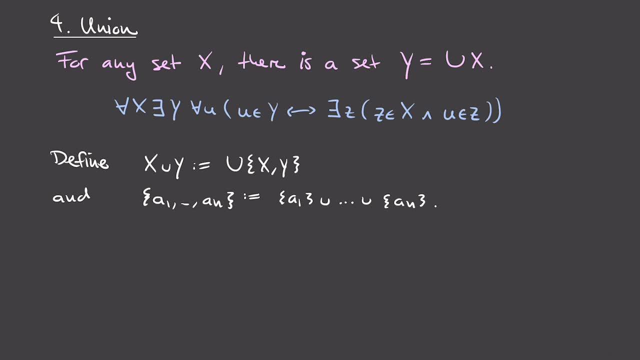 we'll need additional axioms, So that will be the following two. So the axiom of union says that for any set x there is a set y, that is, the union over x. And, as I explained in the introduction here, this big union should again be interpreted. 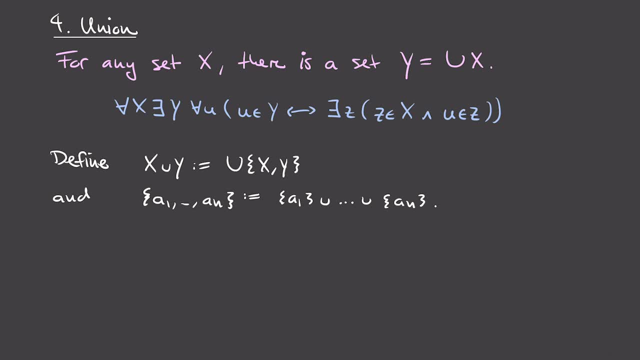 as unioning all of the members of x together. So here you have to think about this as being some collection of sets- let's say s1,, s2, and so on- And the union here is unioning together each of the sets that occur in x. 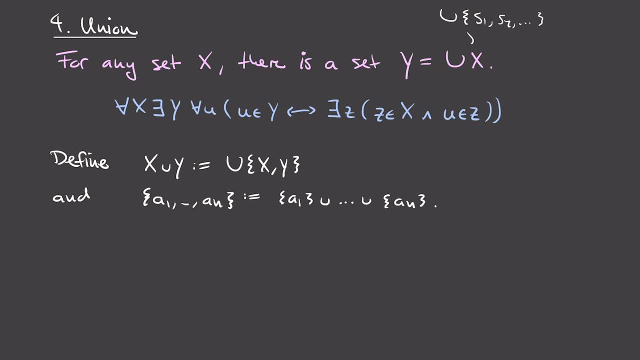 In other words, this union consists exactly of those elements that occur in at least one of these sets s. This idea is expressed in the first-order logic formula for this axiom. So it says that for all sets x. so that's this collection of sets that we want to union together. 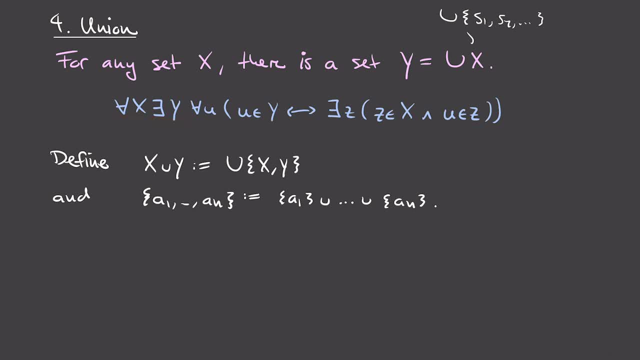 there exists y, which will be the union of those sets, And then we have again this pattern which defines the elements of y. So for all, u u is an element of y if, and only if, the following condition holds, namely there exists some z where z is an element of x. 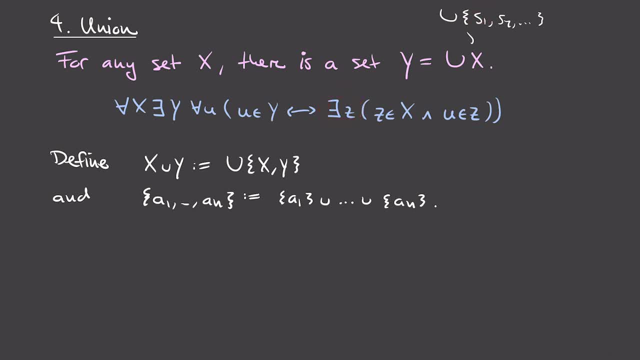 So here this z corresponds to these s1, s2, and so on that I've written up here. So these are like the sets occurring in the collection x. So if there exists a z such that, well, z is an element of x. 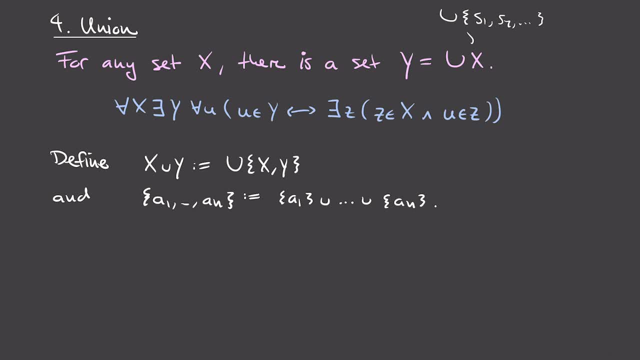 and, moreover, the element u we want to put into the union should be an element of z. In other words, the elements of y are precisely those elements u that occur in at least one of the z's that lies in the collection x. Perhaps this will become a bit clearer. 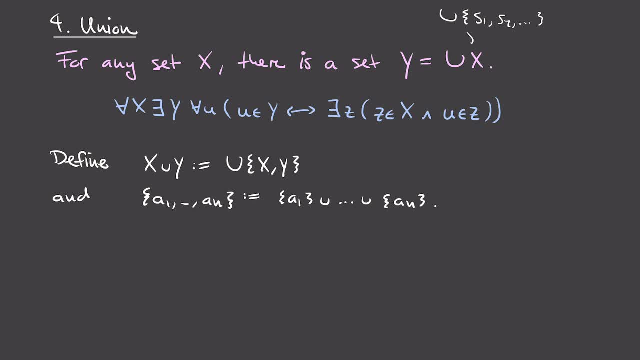 with the following definitions. So, based on this general union, we can define binary unions. So, in order to union together a set x with a set y, what you do is you first pair x and y into a set, So now you have a collection of sets. 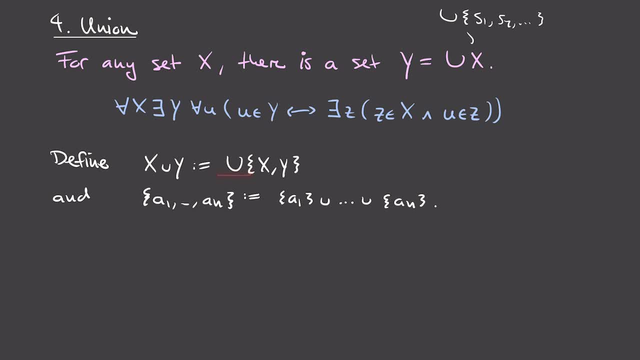 that contains the sets you want to union together and then you take the union. Then, once we have these binary unions, we can actually express sort of sets containing finitely many elements. The way to do this is just to say that a set consisting of finitely many elements. 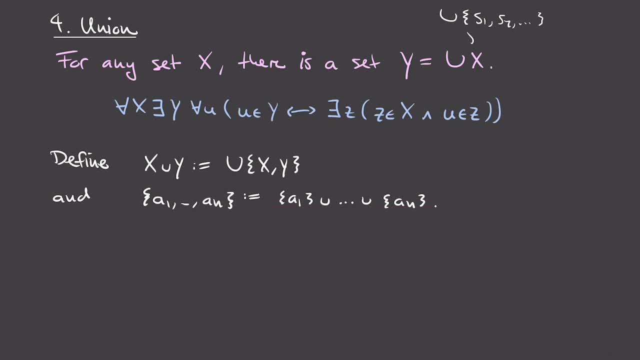 is just the union of all of the singletons containing those elements. So while the pairing axiom allowed us to create sets containing exactly two elements, the union axiom now allows us to create sets that contain a finite number of specified elements by just unioning together the corresponding singletons. 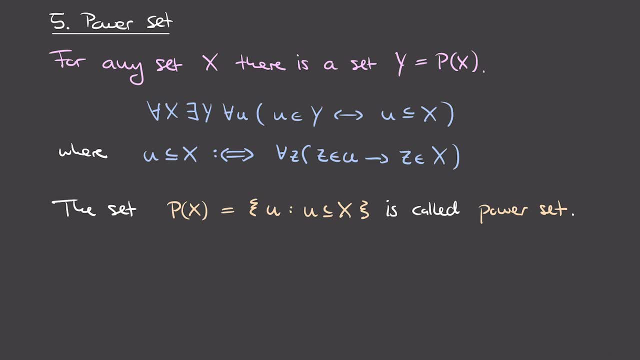 We now move on to the fifth axiom, which is that for power sets. so it says that for any set x there is a set y which is the power set of x. In first-order logic this becomes for all sets x. 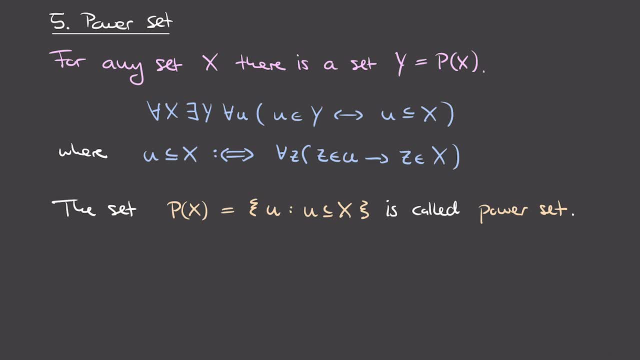 there exists a y which will be the power set of x, such that, while y is defined using again this pattern, so for all u, u is an element of y if, and only if, u is a subset of x. In other words, the power set y consists of all subsets of x. 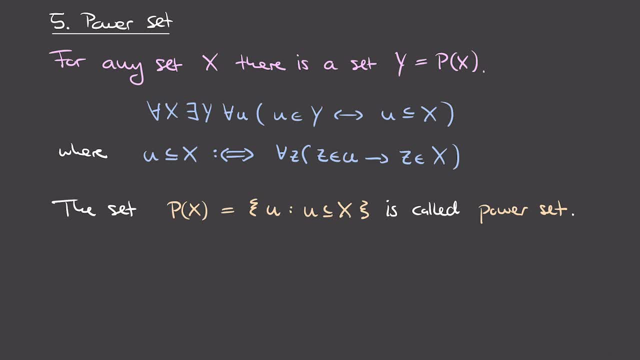 Now, this subset relation here isn't something that's primitively defined in set theory. hence we need to define this subset relationship as follows: So, u being a subset of x, this is equivalent to the following formula, namely that for all elements, z, 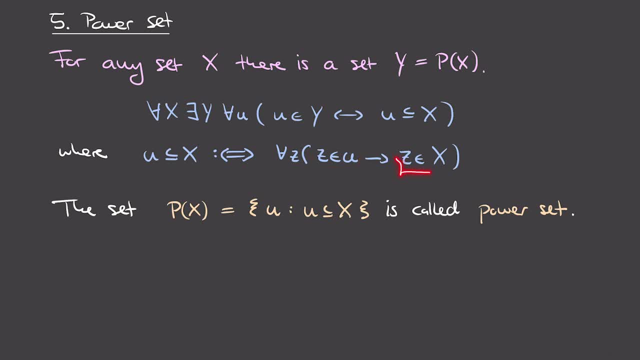 if z is an element of u, well then z is an element of x. So if you wanted, you could just substitute this formula here into this axiom up here, and it would be the same thing. However, the axiom stated in this form is much more clear. 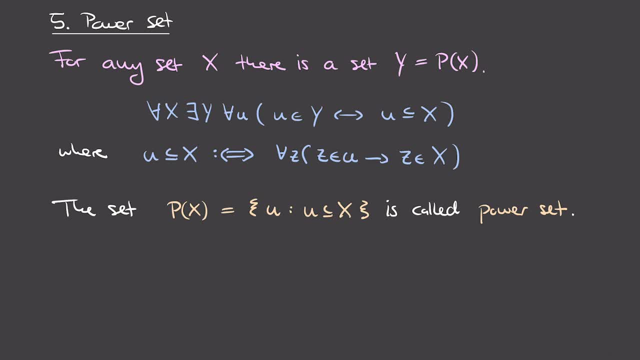 about what this set y we're constructing is Now the set that we obtain here. so all elements u, such that u is a subset of x, so this will be called the power set. Again, this set is unique by the extensionality axiom. 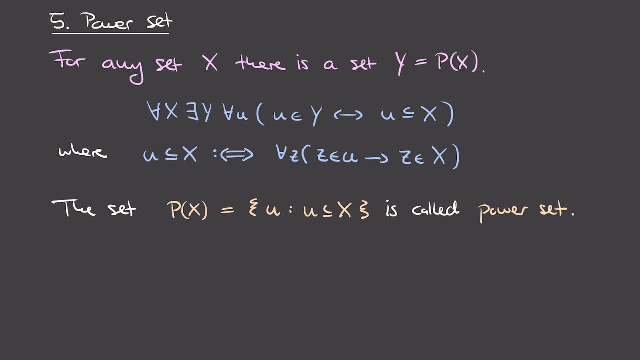 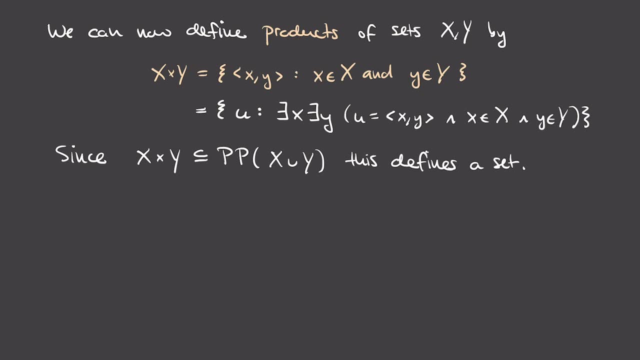 and, as we'll see in just a moment, the power set axiom, together with unions, will allow us to build more interesting set theoretic constructions. The first thing we need to do, the first thing we can do now using the power set axiom, is we can define Cartesian products of sets. 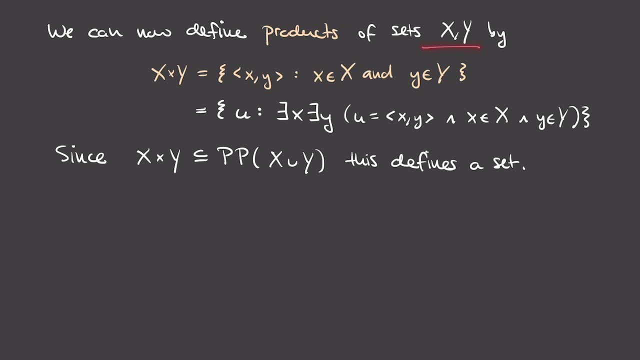 So, given two sets, x and y, their Cartesian product is just the set of ordered pairs x- y, where x lies in x and y lies in y. Now the reason this comprehension here is legitimate and defines a class is because we can rewrite it as follows: 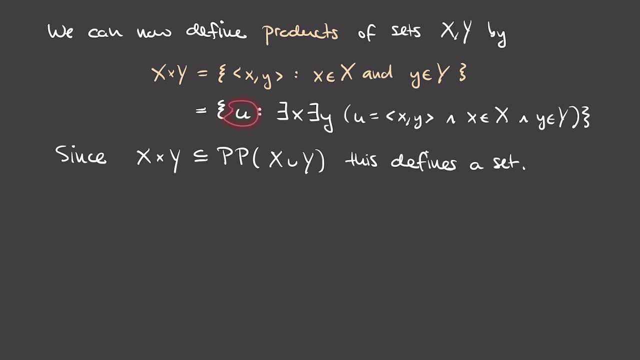 So we can rewrite it as all elements u, such that there exists x and there exists y, such that u is equal to the ordered pair of x and y, and also this first component, x, lies in x and the second component, y, lies in y. 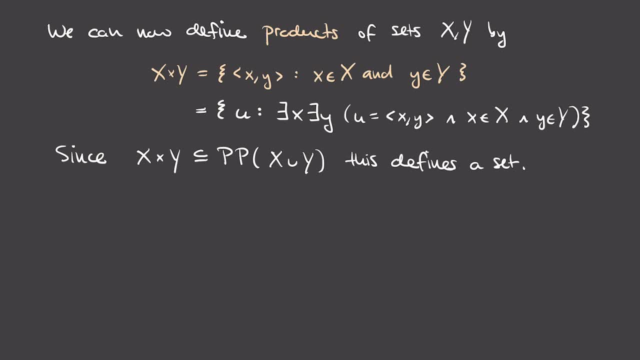 Now, a priori, we only know that this thing here defines a class, but we actually want it to be a set, and the way to show that it's a set is to show that it's a subset of something we know to be a set. 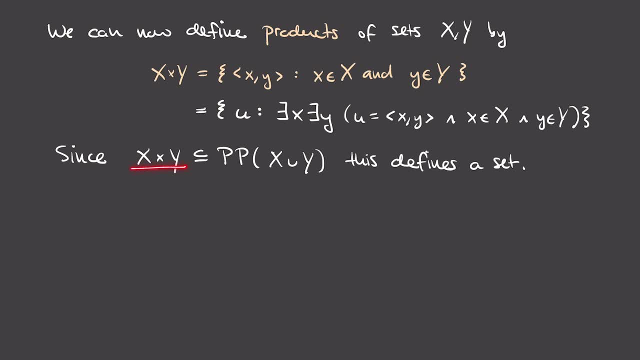 And in fact the Cartesian product x times y is actually a subset of the power set, of the power set of x unioned with y, Now by the union axiom- the union of two sets is a set- and then by power set axiom. 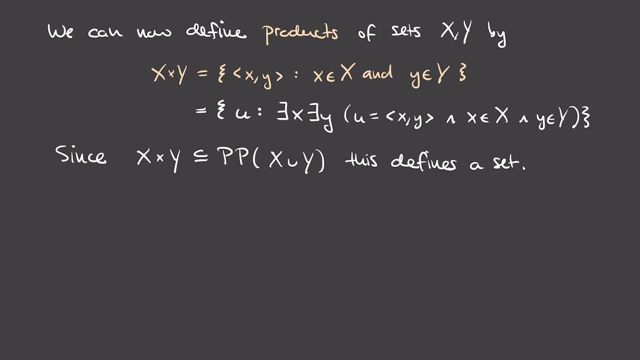 taking power sets of sets again gives you sets and therefore this thing over here is a set, and because this thing is a subset of this very large set here, it means that this thing is also a set. Now, for me at least, it's not clear at first glance that this subset relation here actually holds. 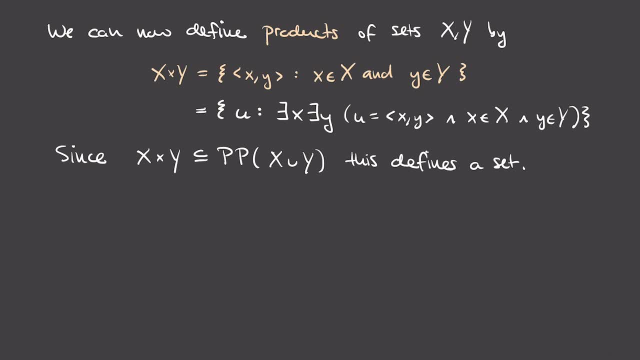 So let's think about this for a moment. So the elements of the set x times y, are these types of ordered pairs right? Thus, in order to show that this relationship here holds, we need to show that, well, every pair like ordered pair is actually an element. 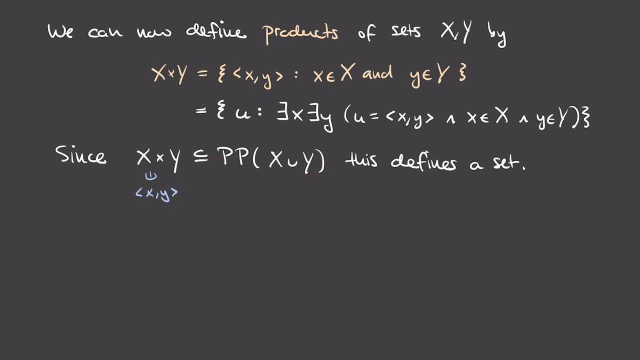 of this large power set, of the power set of x unioned y. Now, if you remember, we defined ordered pairs in terms of, in terms of the following construction: So we took the first component and put it in a singleton and then we paired that with both components. put in a set by pairing. 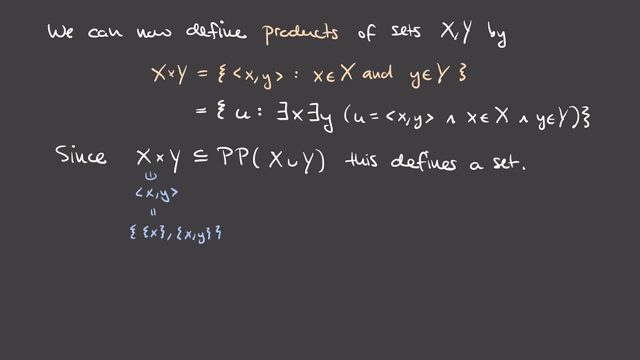 Now, because x is an element of the set capital X. this set here the singleton of x. this is in fact an element of the power set of x And, moreover, this thing here is in fact an element of the power set of x. 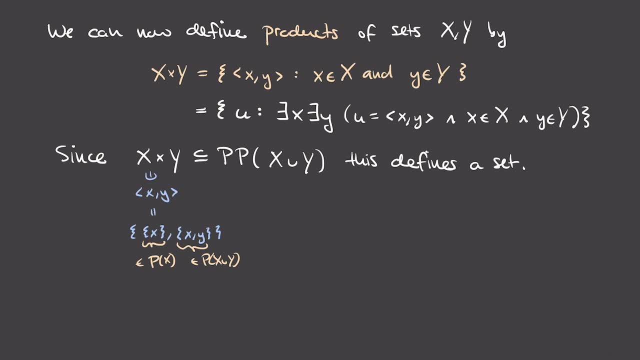 This is an element of the power set of x union y. This is just because the set here containing small x and small y is itself a subset of the union of capital X, capital Y. Now, if you wanted to, you could also think of this singleton containing x. 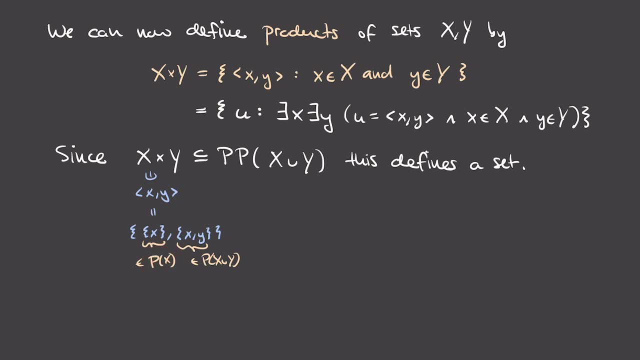 which is an element of the power set of x, as being an element of the power set of x unioned with y. In other words, the power set of x is itself a subset of the power set of x unioned y, and every subset of x is also a subset of the union x unioned y. 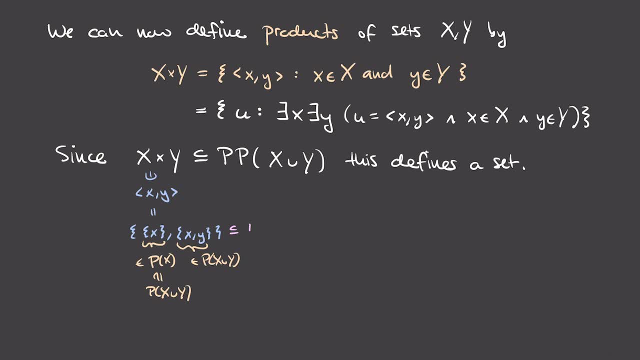 So, overall, this argument shows that this ordered pair is a subset of the power set of x unioned y. The reason for this, again, is because each element in this set is an element of this power set. Now, by the definition of power sets, 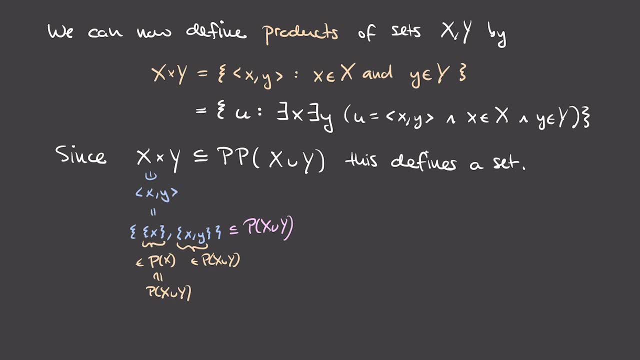 if you're a subset of some set, well then you're an element in the power set of that set. so this in turn means that, well, this thing you could also consider as an element of the power set, of the power set of x unioned y. 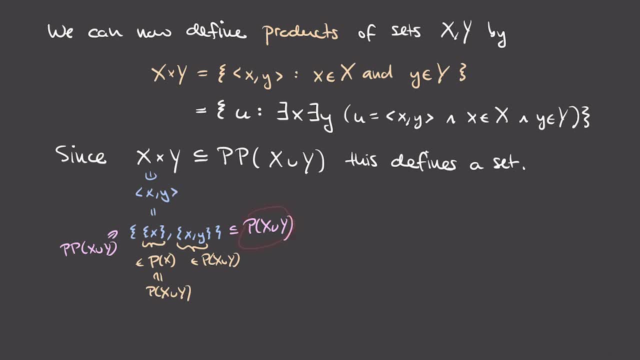 because, well, it's a subset of this one level power set here. Hence we've shown that any ordered pair, so any element of this Cartesian product here, is actually an element of the power set, of the power set of x unioned y. 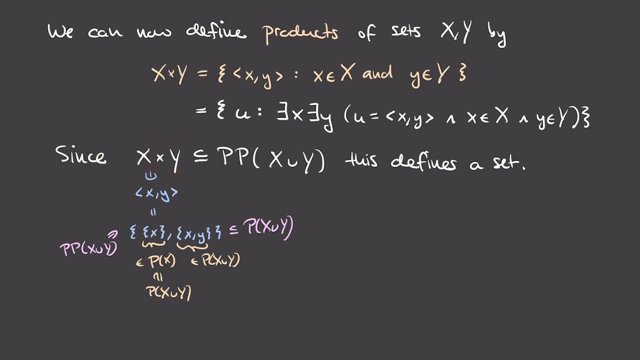 and therefore this entire thing here is a subclass of this power set, of the power set of x unioned y, and because this thing is a set, it means that this thing is now also a set. Finally, we can extend this binary Cartesian product. 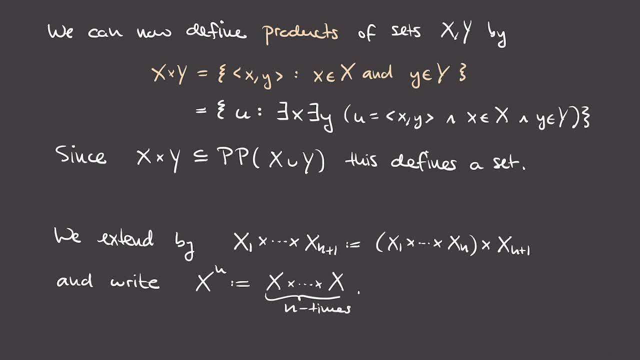 to finitely many sets by just iterating this binary operation. In other words, we define the product of x1 up to xn plus 1 to be the product of x1 up to xn, just times xn plus 1.. So this just corresponds to iterating this binary product here n times. 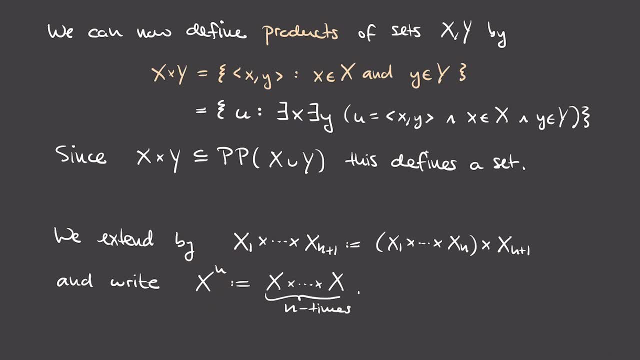 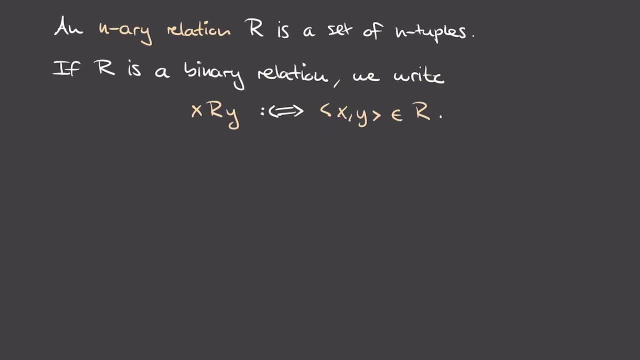 Moreover, we can introduce this notation here: x to the power, n, to mean that we take the Cartesian product of n copies of the set x. Now that we've defined Cartesian products of sets, we can introduce relations, and then from relations we can introduce functions. 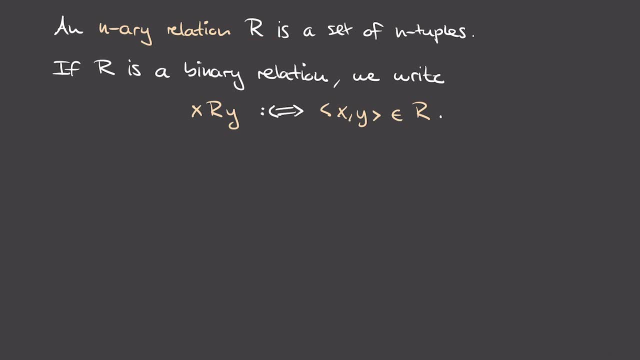 So an n-ary relation R is just a set of n tuples. In other words, a relation R is just a subset of some Cartesian product. Now, if the relation R is a binary relation, meaning it's a subset of just the Cartesian product of two sets- 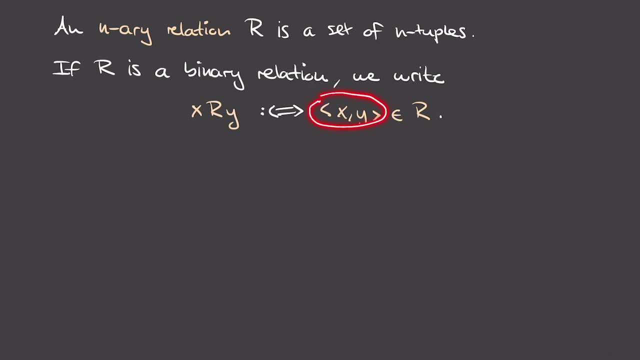 then well, its elements consist of ordered pairs x- y and, in order to write this a bit more nicely, whenever a pair x- y occurs in the relation R, we just write x, R- y. The intuitive way to think about this is that the relation 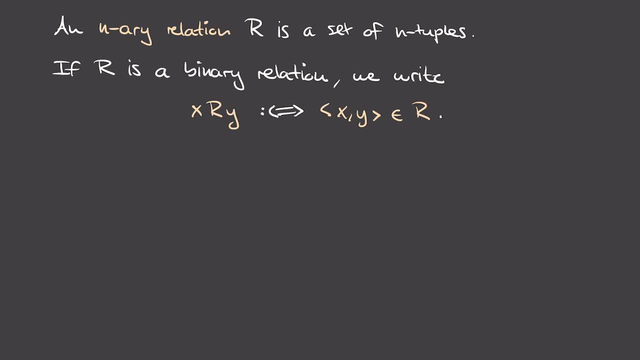 describes certain relationships between elements of a set x and elements of a set y, and two elements are related precisely when the corresponding ordered pair is an element of the relation, And hence we write x, R, y to express that x is related to y. 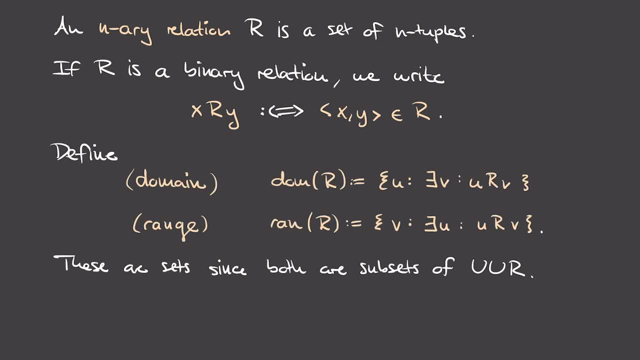 Once we have relations, we can define their domains and ranges. So the domain of a relation is just all of the first components that occur in the relation. So it's the set of u, such that there exists a v where u is related to v. 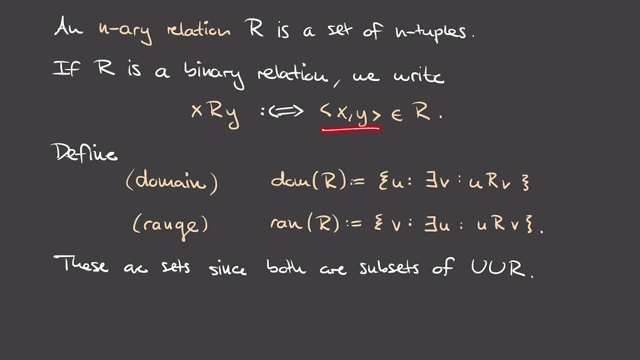 In other words, we're just projecting these ordered pairs that occur in the relations onto the first components. Similarly, the range is just the set of all v, such that there exists a, u, such that u is related to v. This just means that we're taking all of the ordered pairs. 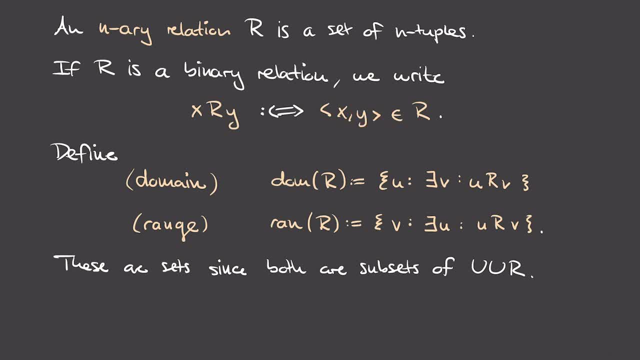 occurring in the relation and projecting onto the second component. Now, again, in this definition, a priori these things are just classes. We don't yet know that they're sets, But in fact it turns out that both the domain and the range of a relation 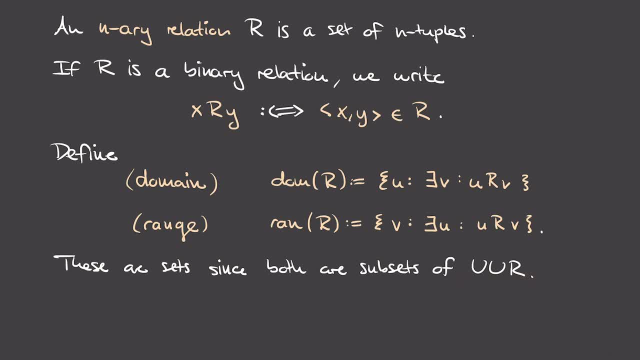 are subsets of the union, over the union, over the relation. Let's think about why this claim is true. So the relation R consists of some set of some ordered pairs- right, And I'll just write a single one here. And this ordered pair here is equal to the set containing the singleton x. 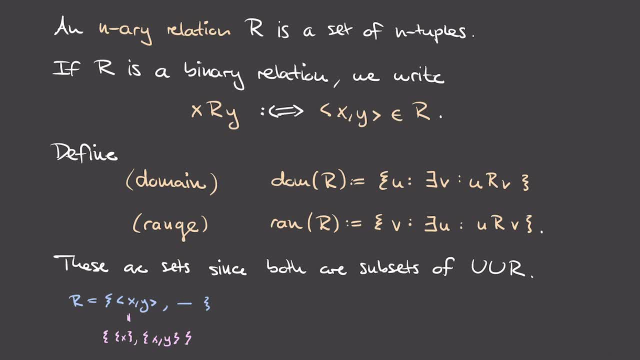 and also the set containing x and y. And now let's think about what happens if we union over R. Remember that unioning over a collection basically just takes the union of all the sets occurring in the set. So here the collection is denoted by these outer parentheses. 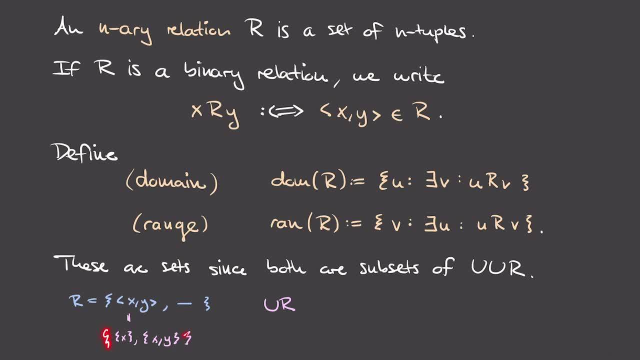 And then the sets that we're unioning over are basically these sets that occur inside. In other words, the union over R will consist of all sets that occur in at least one of these ordered pairs. So for this first ordered pair, things that occur in the union will be: 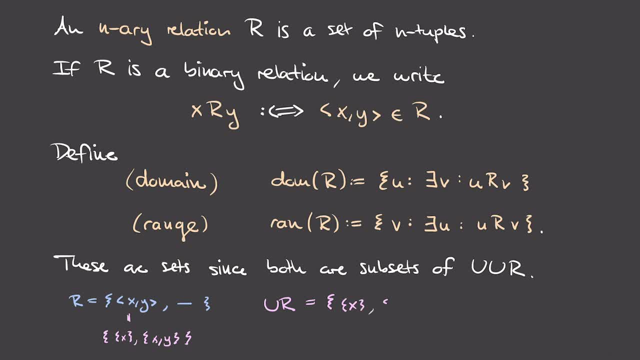 well, the singleton containing x and also this set containing x and y, And then we'll have additional elements here occurring. that well are basically the singletons of all of the first components of the ordered pairs, and then also sets containing both the first and the second components. 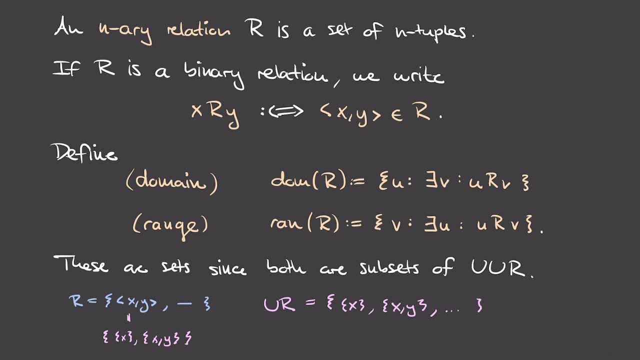 of each of the ordered pairs that occur in the relation. Okay, and now if we take another union over this set, well then we're just unioning together all of these sets that occur in this larger set here, And so this union over the union of the relation. 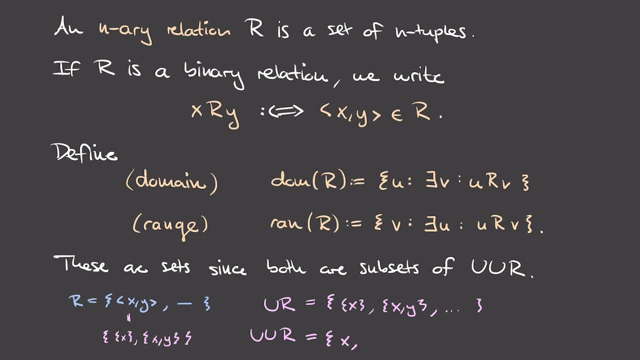 will, for instance, contain just the element x. It'll also contain the element y, because, well, we're including this set here in the union, And, moreover, it'll contain, basically, well, any of the components that occur in the ordered pairs in the relation. 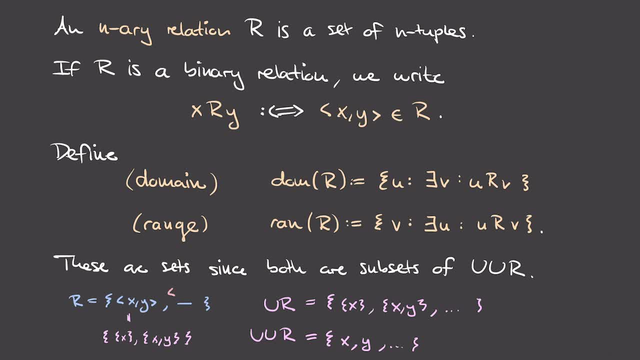 Okay, So let's say I had some additional ordered pair here, Let's call it uv. Well then, in this union over r, I would have now an additional set singleton u and the pairing u and v, like so. And then now in this union over the union of the relation, 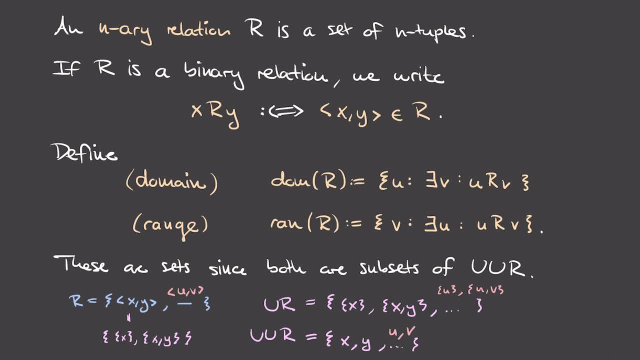 I would now also have the elements u and v occurring, since, well, u and v both occur in at least one of the sets occurring. in this set here In particular, you can see that the domain which is just the first components of the ordered pairs in the relation 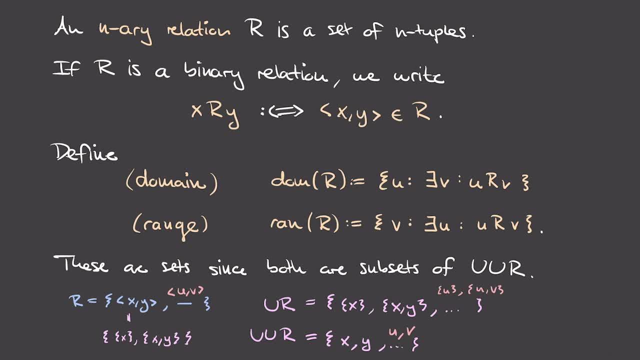 well, each of those first components occurs in this set And therefore the domain is a subset of this union over the union of the relation. And a similar thing goes for the range, because each of the second components of the ordered pairs occurring in the relation. 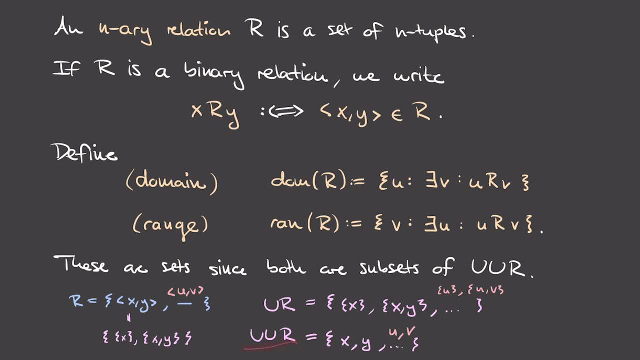 will also be an element of this double union here. So that proves that these things here, which are in principle just classes, are in fact sets, because they are subsets of this larger set. And we know that this is a set well because 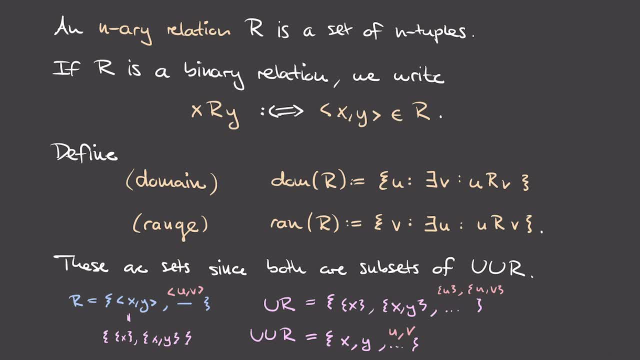 well, on the one hand, we know that the Cartesian product is a set, And well, r is just a subset of the Cartesian product. And well, if we union together sets, we get sets by the union axiom, And so this thing is definitely a set. 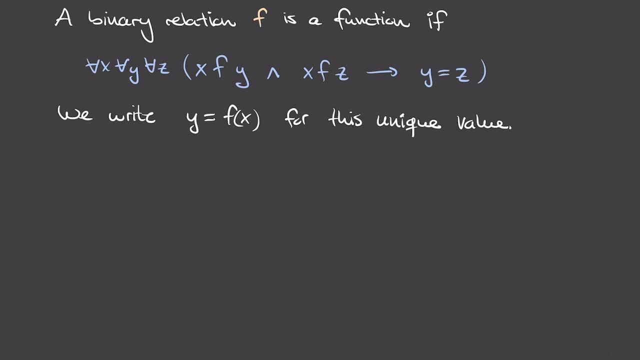 Once we have relations we can also define functions to be special types of relations. So we say that a binary relation f is a function if it has the following property: So we want that for all x and for all y and for all z. 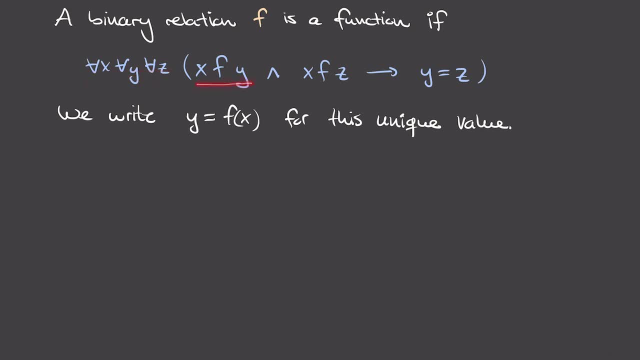 If x is related to y via f and also x is related to z via f, then in fact we want y and z to be equal. In other words, this property is saying that f relates some given element, x, to at most one other element. 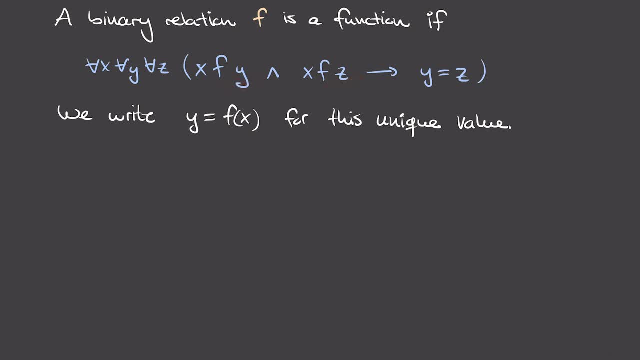 So this is saying that a function should be single-valued. So for each input to the function, you want to have at most one return value. Now, because of this uniqueness expressed in this property, we can write: y is equal to f of x. 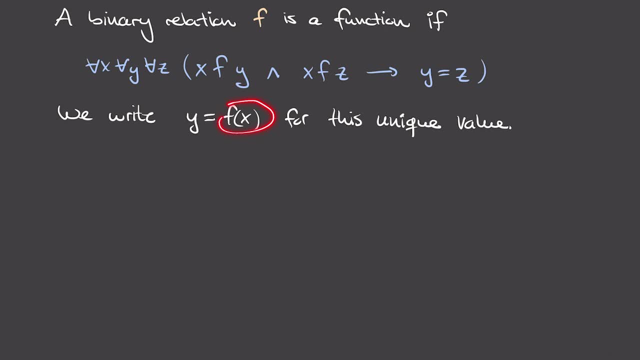 for the unique value y that x is related to via f. So this gives us our usual notation for functions where we write f of x for the value that f assigns to x. We can now further think of a function as going between two sets in the following way: 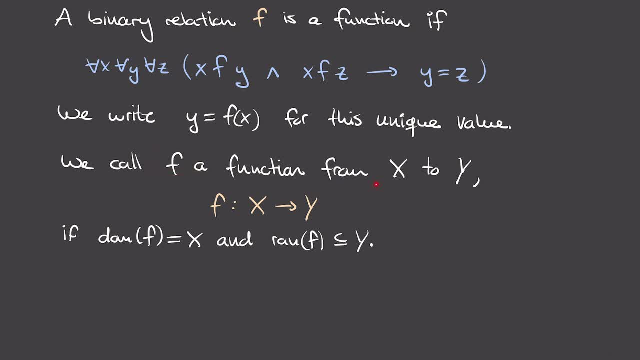 So we say that a function, f, goes from a set x to a set y and we denote it like this: so f going from x to y with the arrow. This holds if, on the one hand, the domain of the function is equal to x. 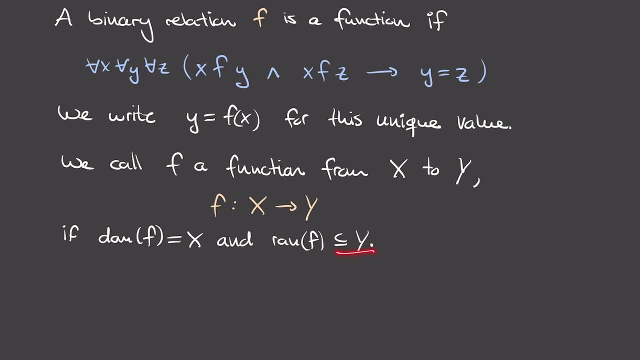 and, on the other hand, the range of the function is a subset of the target set y here. In other words, we want our function to be mapping f, mapping every element in the set. it's starting from to some element and we want that element that it maps to. 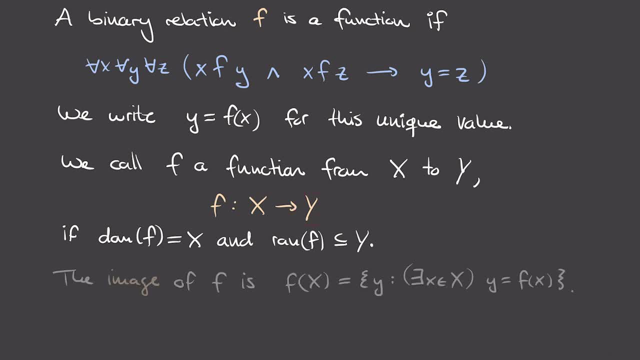 to lie in the target set y. Moreover, we can then define the image of a function, So the image is basically just the set of values in the target set that are mapped to by f, In other words the image f of capital X. 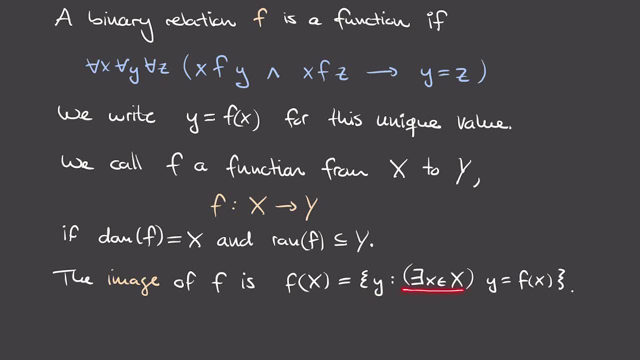 is the set of all y, such that there exists an x in x, such that y is equal to f of x. Now, here in this formula I've used this restricted quantification, so there exists x in the set x. This is not formally part of our language. 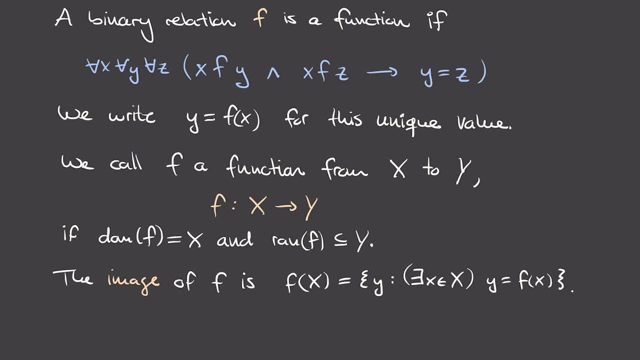 but we can convert this restricted quantification to an unrestricted version in the manner that I discussed in the video on first-order logic. Finally, we can consider the class of all functions going from a set x to a set y, and in fact it turns out that this class 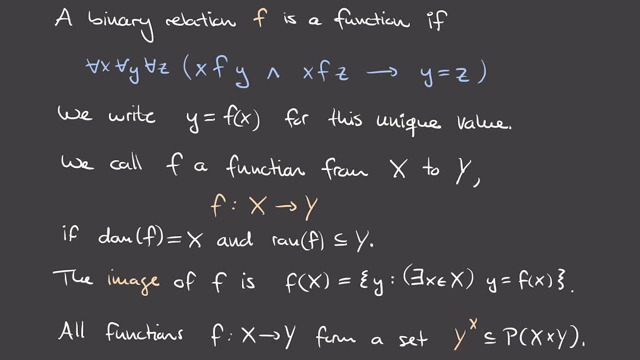 which we denote y to the x, is in fact a subset of the power set, of the Cartesian product of x and y. Why is this? Well, a function is just a relation, right, And a relation is just a subset of the Cartesian product of x and y. 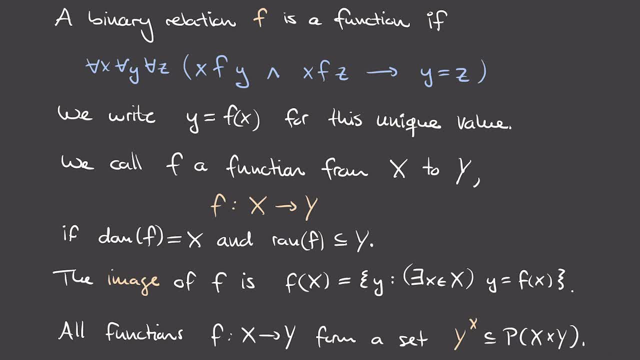 Hence every function is a subset of the Cartesian product and thus every function is an element of the power set of the Cartesian product x and y. Hence we conclude that every element of this function space here is an element of this power set and therefore this inclusion here holds. 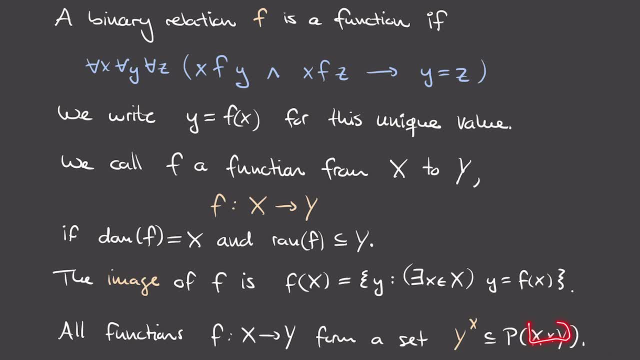 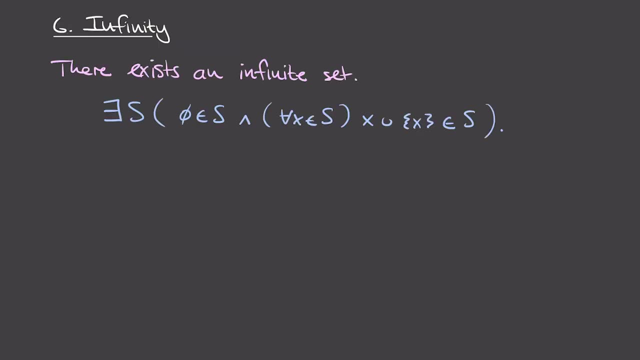 Now, because we know that the Cartesian product is a set and the power set of some set is a set, by power set axiom, we can now conclude that also the class of functions from x to y will form a set. We can now move on to our next axiom. 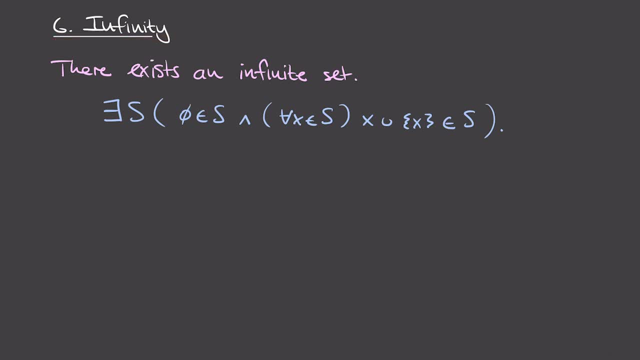 which is the axiom of infinity. Informally, this says that there exists an infinite set. Now, finiteness is usually well phrased in terms of the natural numbers, and so far we haven't yet constructed any natural numbers, so we'll need some other way of defining an infinite set. 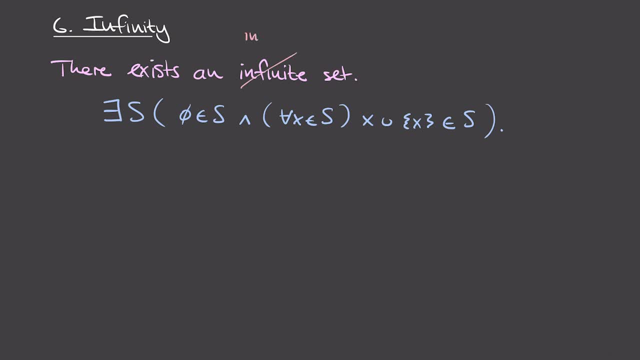 So, rather than saying what an infinite set is, we're in fact going to define what's called an inductive set, and it'll turn out that inductive sets are in fact infinite once you construct the natural numbers. but for the moment, this inductive set definition. 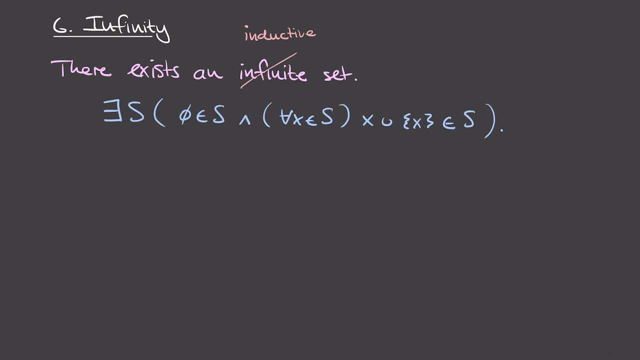 is much simpler. What it says is the following, in first-order logic: So it says that there exists some set, S, so that's the inductive set we're interested in, such that the empty set is an element of S, and also for all elements x and S. 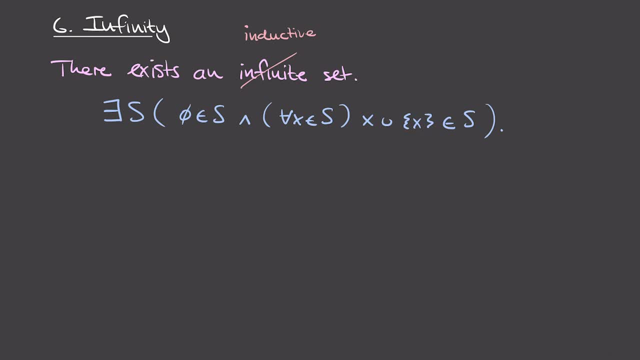 x union. the singleton x is also an element of S. Okay, why does this give you an infinite set? Well, let's start writing down S, right? So, on the one hand, we know that the empty set is an element of S. 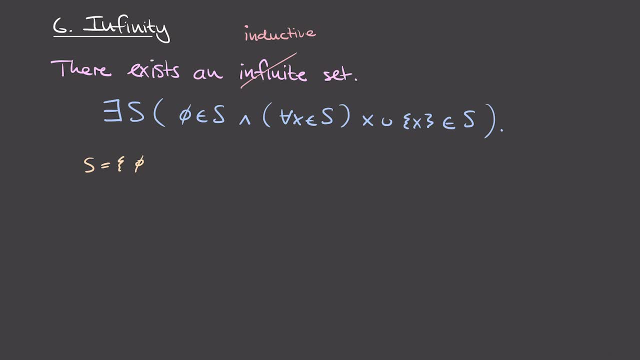 so that's the first part of the definition of S. and then we know that for any element x that occurs in S, if we union that element together with the singleton containing that element, that also needs to be an element of S. Now, so far we only know that the empty set is an element of S. 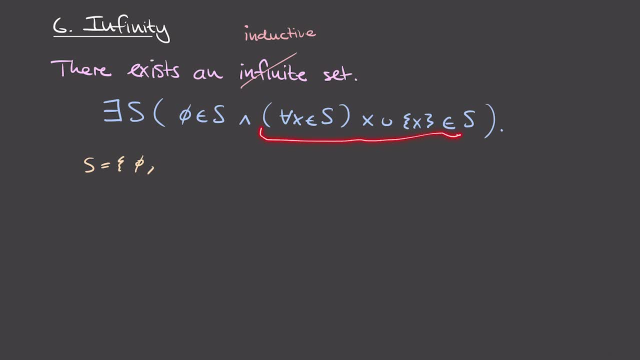 but now we can apply this inductive part of the definition to conclude that S has to have an additional element, so that element would be of the form x union, the singleton containing x. so in this case we instantiate this with the empty set being x. 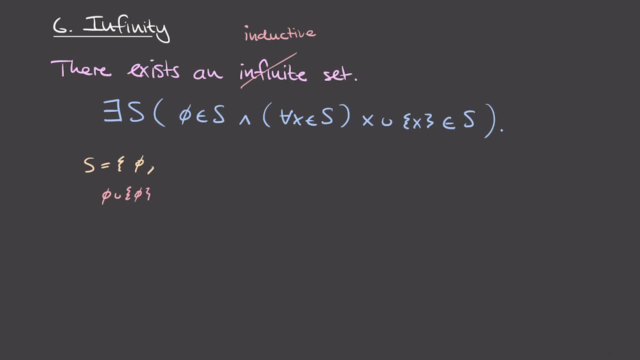 so we know that the empty set unioned the singleton containing the empty set. this also needs to be an element of S, On the other hand, because the empty set has no elements. if you union with the empty set, you just get back whatever set you're unioning with. 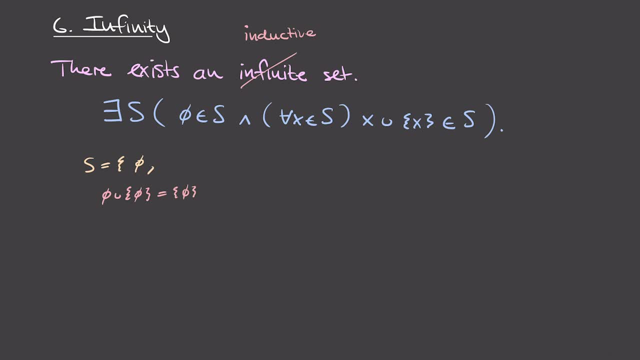 so this is equal to just the singleton containing the empty set. Alright, from this we can conclude that also the singleton containing the empty set will be an element of this set S. and now we can proceed in the same manner. we now know that by the inductive condition that the following set here: 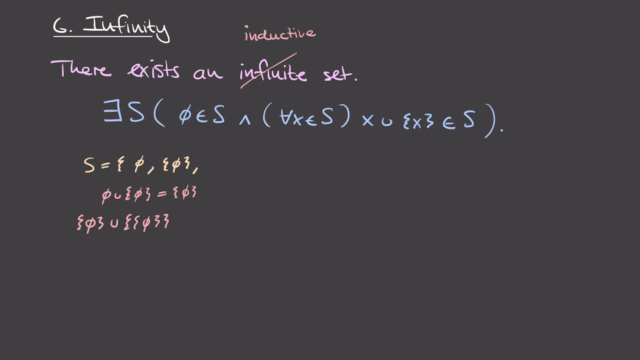 so the set containing the empty set, unioned with the set containing the set containing the empty set, has to be an element of S. and what is this? Well, here we're unioning the set containing the empty set with this larger set, so the result will be the set containing the empty set. 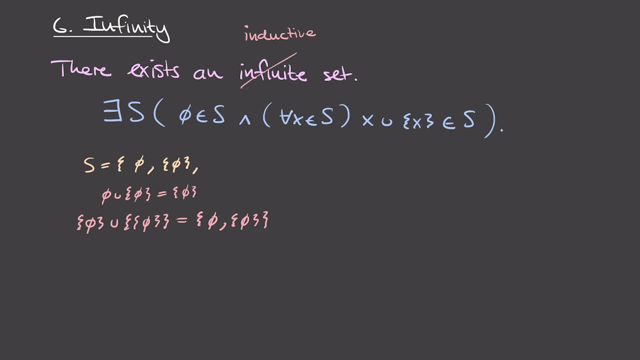 and also the singleton containing the empty set. So from this we now conclude that also this set is an element of S, and so on. So each time you apply this inductive part of the definition, you'll get a new set, and therefore this process will continue on indefinitely. 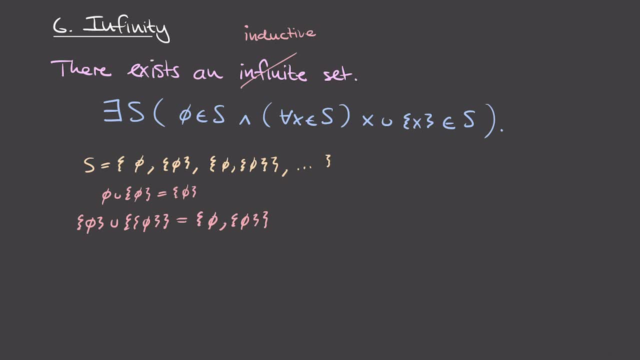 and this means that this set S actually has to have an infinite number of elements. Now, if you were paying attention before, you might notice that. well, we said when we defined the empty set that the existence of the empty set depends on the existence of another set. 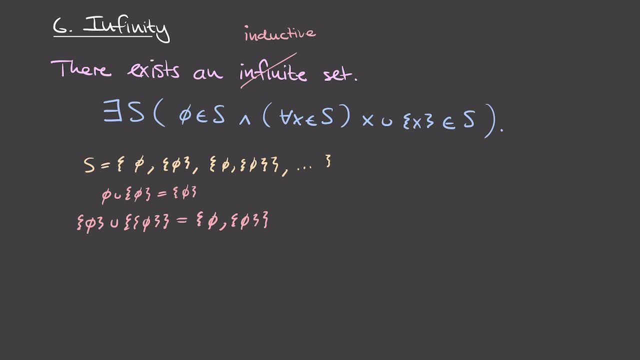 and the set we're using to sort of obtain the empty set is in fact this infinite set here. So it might seem like this definition here is circular, because in order to know that the empty set exists and define it, we somehow need to first assume that S exists. 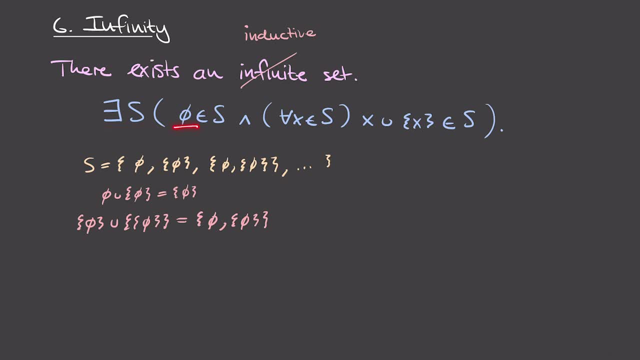 but somehow the definition of S is in fact making use of this empty set. But in fact there's no circularity occurring here. To see this, you would just replace this empty set symbol here by its definition. so it's all the u's in S, such that u is not equal to u. 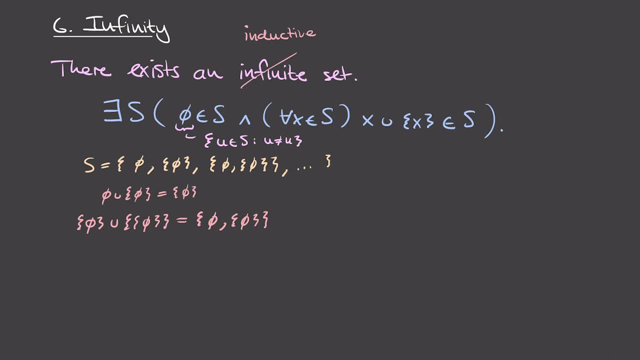 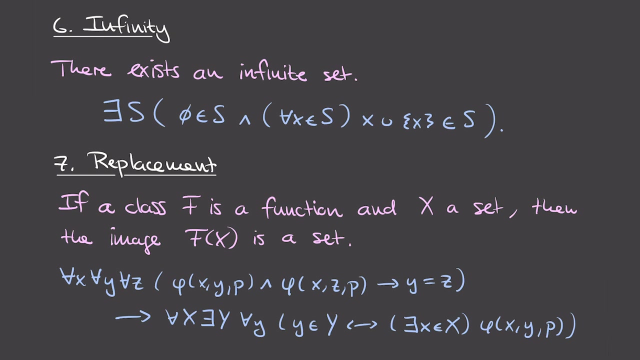 And in this case the statement then just becomes a statement about the existence of a set S, such that it contains as an element some set which is defined in terms of that set S, and it also satisfies this additional condition here. We now move on to the replacement axiom. 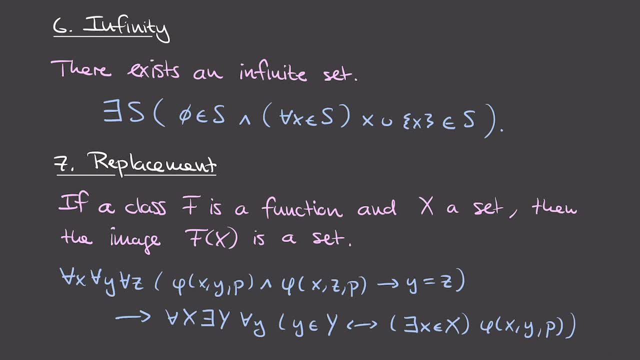 which should now be clear that we've defined functions. In words, it says: if a class F is a function and x is a set, then the image capital F of x is also a set. Now, in our definition of functions, we defined functions as being certain relations. 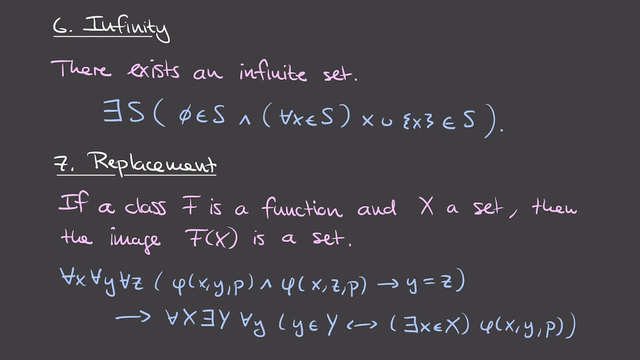 and relations were, in term, subsets of a Cartesian product of sets. So in this example now if you replace the Cartesian product of sets with a Cartesian product of classes- so that would just be ordered pairs where each component occurs in the corresponding class- then you get basically a definition of a function that isn't necessarily a set. 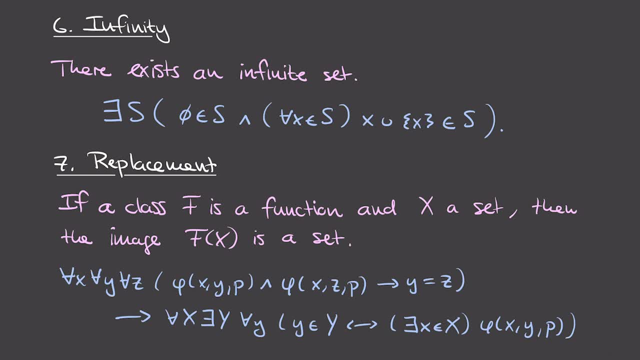 So these would be more general functions which are not necessarily a subset of a Cartesian product of sets, but rather are subsets of a Cartesian product of classes. Now what this axiom is saying, if we have such a function, which doesn't even necessarily need to be a set, 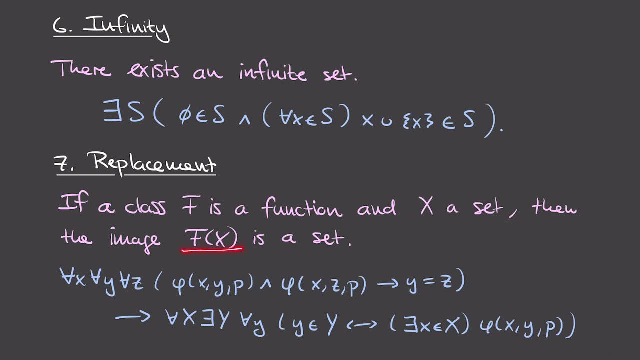 and we look at the image of a set under that function, then that image is in fact again a set. In other words, we can somehow map existing sets using functions, and even if those functions aren't necessarily sets themselves, the image that they define will again be a set. 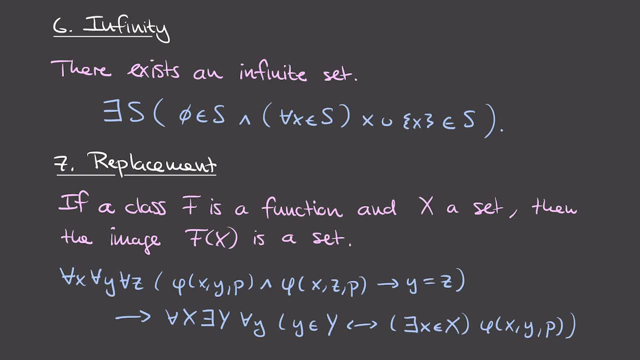 Now, in first-order logic you express this as follows: It's a bit lengthy because we have to kind of include the definition of a function in the formula. So we say that, okay, for all x, for all y and for all z. 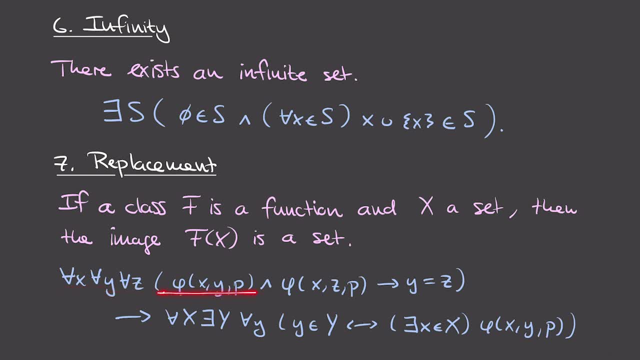 if phi of and phi of both hold, then y is equal to z. So this part here of the definition is essentially saying that the formula phi here defines a function. So you need to think about this. phi of is saying that phi maps x to y. 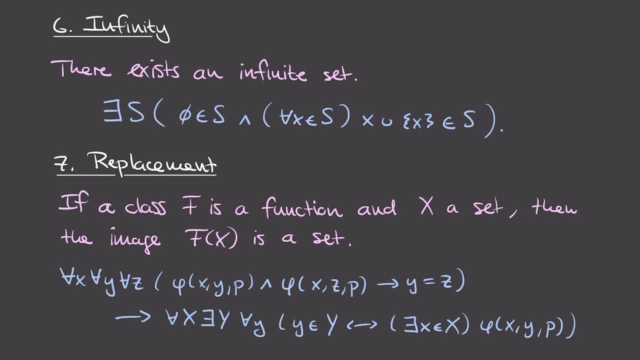 if we fix the additional parameter p, And similarly here the second one is saying that phi maps x to z under the fixed parameter p And hence in total this condition here is saying that x is mapped to a unique target value, because if you have x being mapped to y, 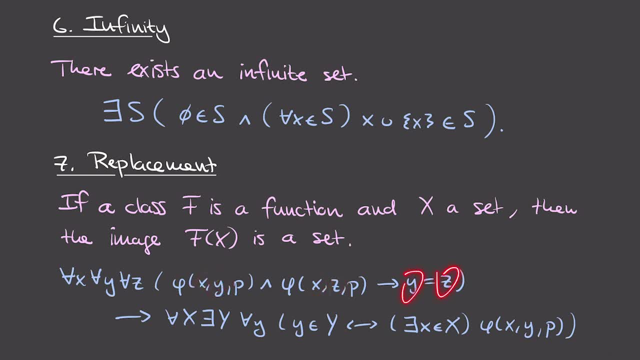 and x being mapped to z, then in fact y is equal to z. In other words, this formula phi here defines a function, and if this is the case, so that's basically what this premise here is saying. so if the formula phi defines a function, then well, for all sets x. 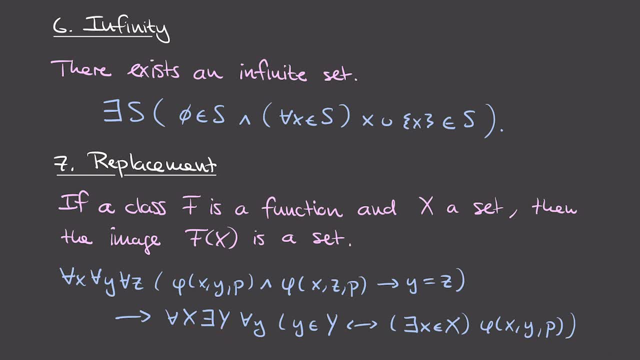 there exists a set y, namely the image set, such that for all elements y, y is an element in small y. so this is defining the elements of y if, and only if, there exists a small x in x, such that phi of. 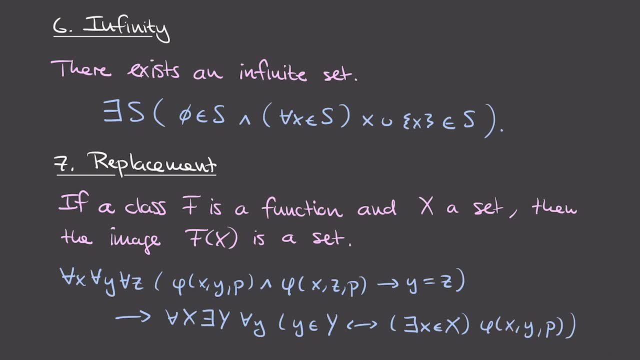 so phi maps x to y. Okay, so this formulation is perhaps a bit confusing, but the easier way to think about it is just saying that we define some class of pairs, such that, well, phi of holds. now, in that case, the hypothesis here is precisely saying that this class 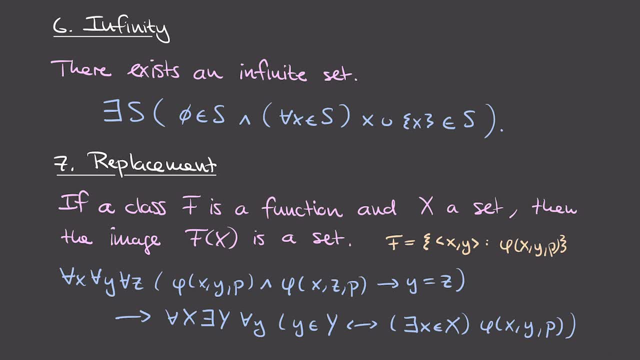 is a function for each fixed p, so maybe I should call this like f sub p or something like that. and then the premise is saying that well, under this assumption that f sub p is a function, then there exists a y, namely the image, and the image is defined using this formula. 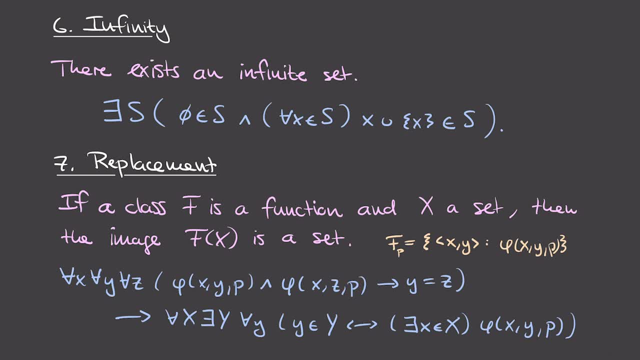 Now, since p here occurs free in the formula, so it's not being bound by any quantifier, the way to interpret this axiom is probably to say that: well, this type of axiom holds for any choice of parameter p. so perhaps a better way to formulate it would be to put a quantifier. 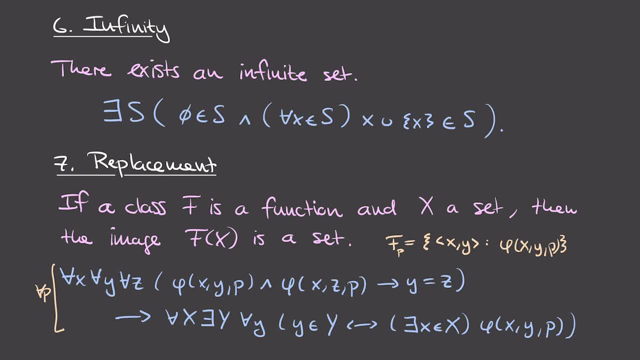 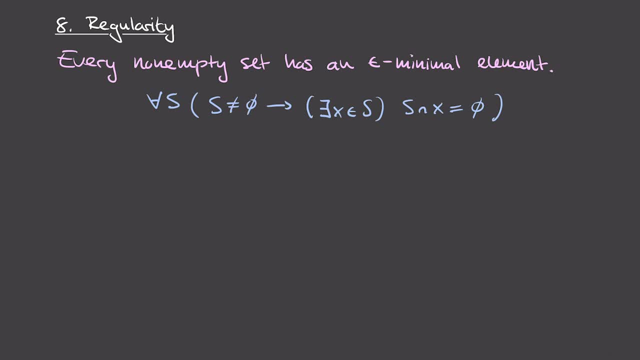 for all p in front of this large formula. This already brings us to the final two axioms, which are regularity and choice. These are perhaps also the most difficult to understand. so regularity says that every non-empty set has an element-minimal element. 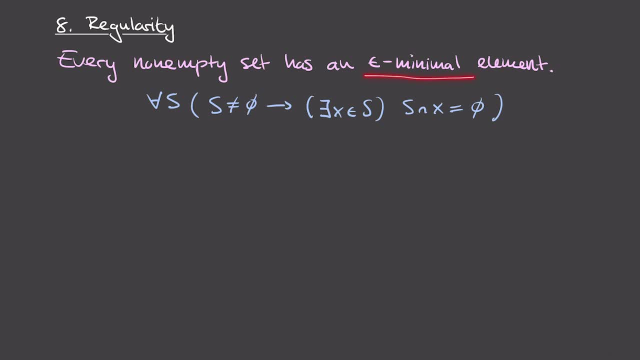 and well, essentially, this is just the term for what this formula is expressing. So it says that for all sets S, if S is non-empty, then this condition holds. This condition is precisely what it means to have an element-minimal element. 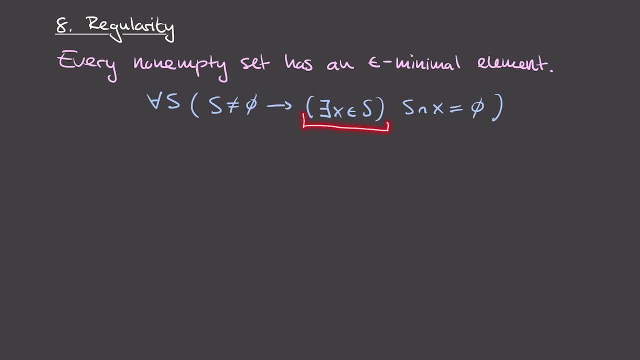 So this condition says that there exists some element x in S such that that element is disjoint from S, So S intersected with x is the empty set. In other words, regularity is asserting that in each set you have to have at least one element that is disjoint from the set that it's contained in. 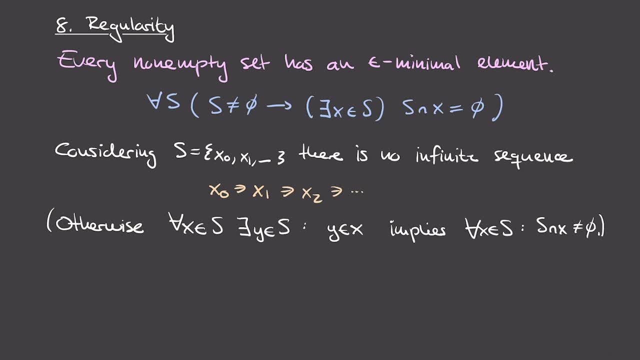 Now phrased in this form, the axiom isn't particularly clear about what its consequences are. but one consequence of the axiom is that you can't have these infinite sequences of inclusions of sets. In other words, you can't have a set x0,. 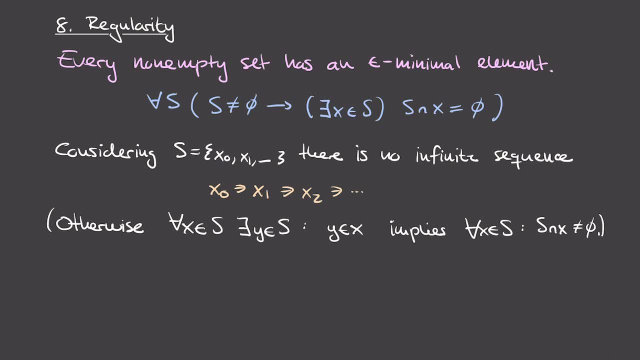 which has as an element a set x1, which has as an element a set x2, and so on. You can't have an infinite sequence of like this being an element of Now if you consider this set here, so the set containing x0,, x1, and so on. 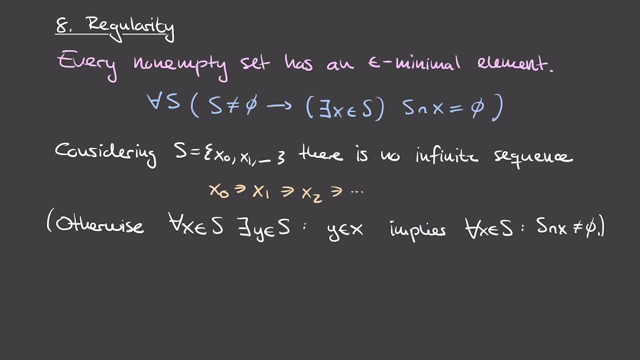 and you additionally assume that each xn plus 1 is an element of xn, so you have an infinite sequence like this of being an element of. well then, for every x in S, so for any x you choose here, there will exist a y in S. 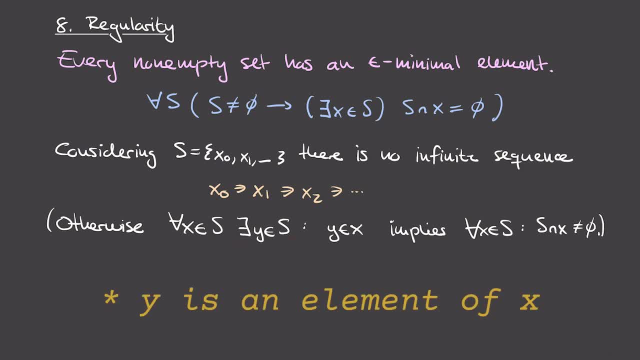 so some other set, namely the next one, such that y is an element of S, So for any choice here, for instance x0,, I can find another set, namely the next one, so in this case it would be x1,. 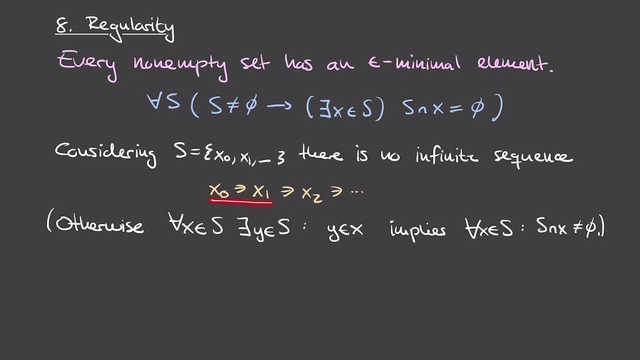 such that, well, x1 is an element of x0, so that's what this hypothesis here is asserting, And this holds for every element of S, because I can just always choose the next set occurring in S, and this will be by this hypothesis here. 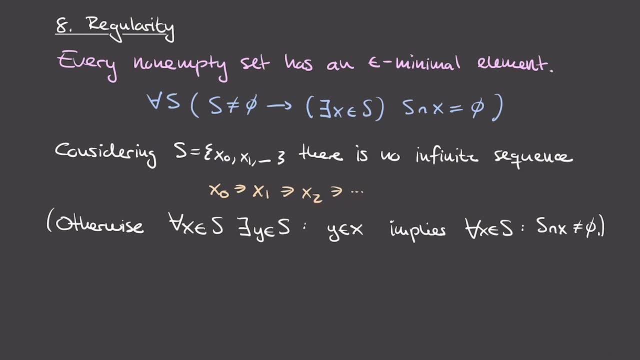 an element of the set preceding it. Okay, but if this statement here holds so, for all x in S, there exists a y in S, such that y is an element of x. well then, it's the case that for all x in S. 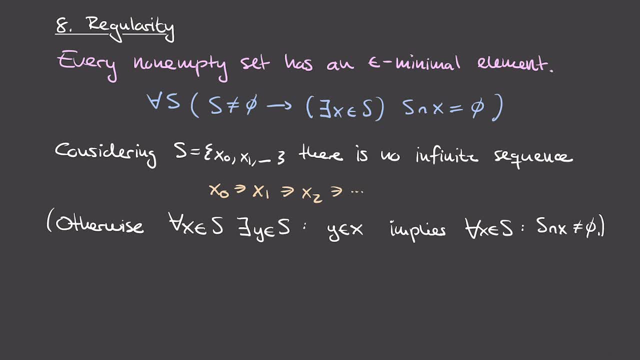 S intersected with x is actually non-empty. But why is this? Well, you just pick some, let's say, an xn occurring in S right, And now we know that xn plus 1 is an element of xn. but on the other hand, 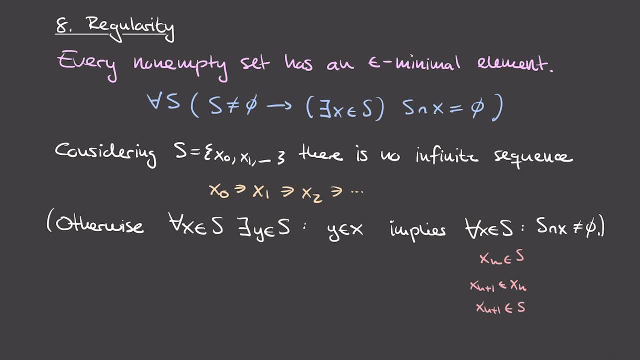 xn plus 1 is also an element of S and therefore S intersected with this. xn will at least contain this element- xn plus 1, because this is an element both of xn and also an element of xn, so an element of S. 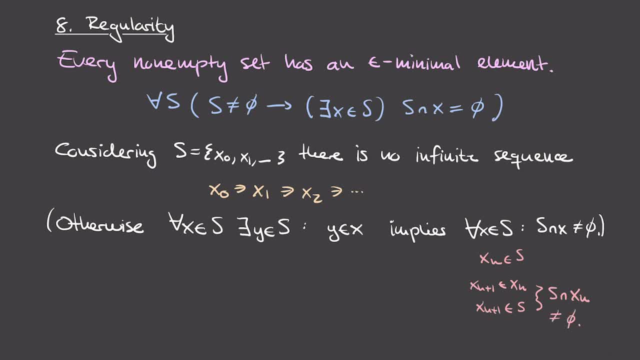 So this means that this is non-empty and this holds for any choice of x in S. okay, Hence, in conclusion, if we assume this type of infinite sequence here, then this implies that for all x in S, that x is not disjoint from S. 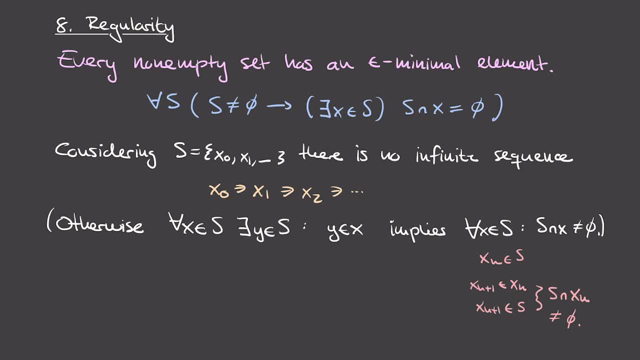 But that is exactly the negation of what this statement here is saying. so this condition, So in that case this set S would violate the regularity axiom, and hence we conclude that such infinite sequences here can't exist. Okay, so we've converted this regularity axiom. 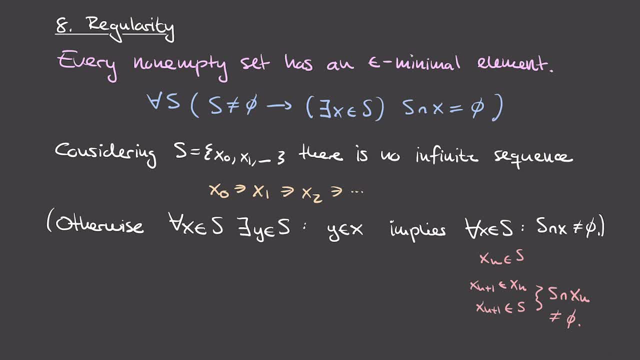 into one of its consequences. saying that we can't have such an infinite sequence of being an element of Perhaps forbidding such infinite sequences here still seems a bit mysterious. but it has some consequences which are desirable. So if you can't have such an infinite sequence, 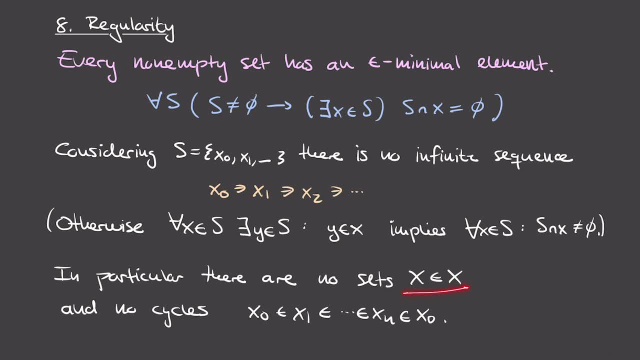 in particular, you can't have any set that's an element of itself, Because otherwise you could write out an infinite sequence as follows: So you would just write like: x is an element of x is an element of x, and you can go on forever like this. 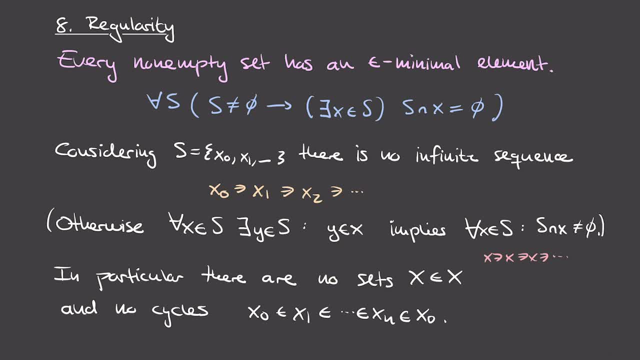 So in this case, you can't have any x, which is an element of itself, And, moreover, for similar reasons, you also can't have any cycles, So you can't have a set x0 being an element of a set x1,. 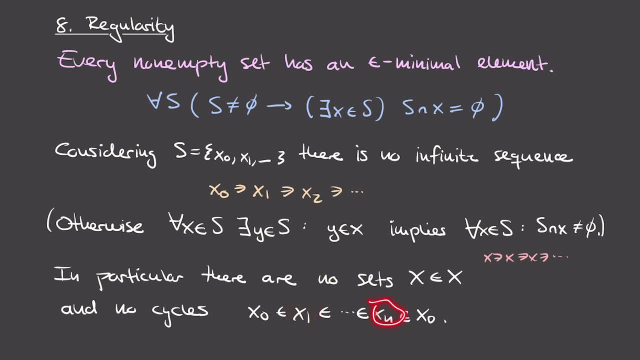 and so on Up to a set xn, And then that xn is again an element of x0. Because otherwise you could again write out an infinite sequence. So you could write out x element, x1, element, and so on up to xn. 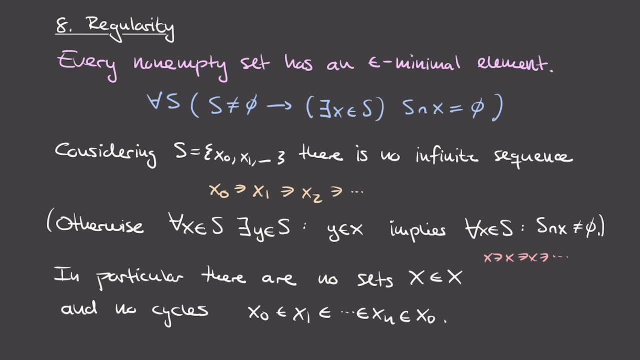 and then is an element of x0,, is an element of x1, and you can go on like that forever. That would again give you one of these forbidden infinite sequences, And hopefully these two conditions seem like reasonable things you would want to forbid. 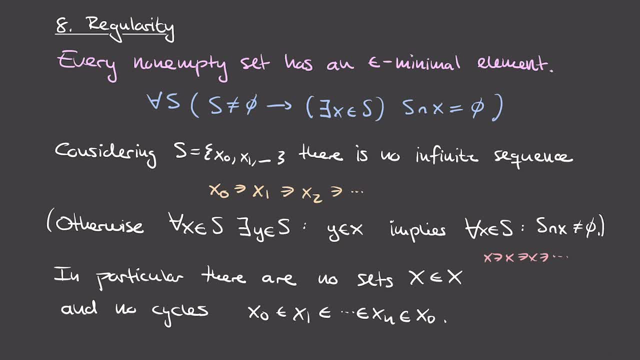 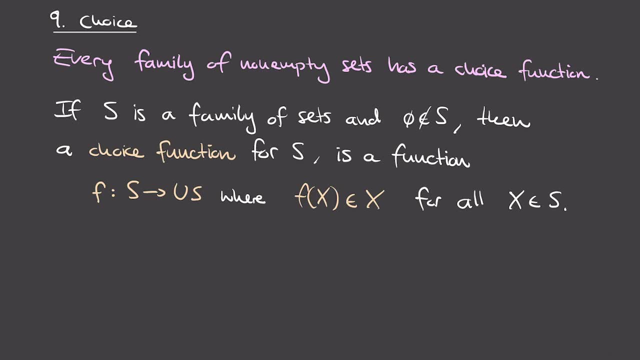 if you start thinking about what sort of sets would satisfy these conditions. Finally, we move on to the last axiom, namely the axiom of choice. It says that every family of non-empty sets has a choice function. So here I need to explain what such a choice function is. 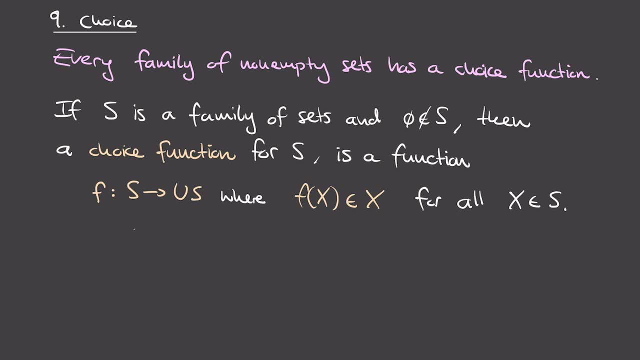 And I think the easiest way to do this is just to draw a picture. So we suppose that we have some family of non-empty sets, So I'll draw it like so. So we have like some sets here. Let's call them like x1, x2, x3. 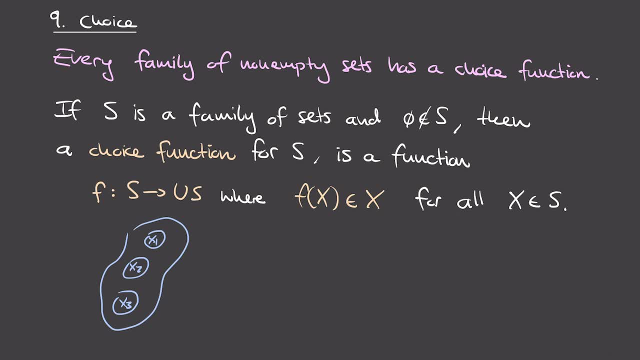 And now the idea is that for each one of these sets occurring in the family, we want to pick an element out of each one of them simultaneously. Okay, so somehow a choice function will select from each of the sets in this family some element. 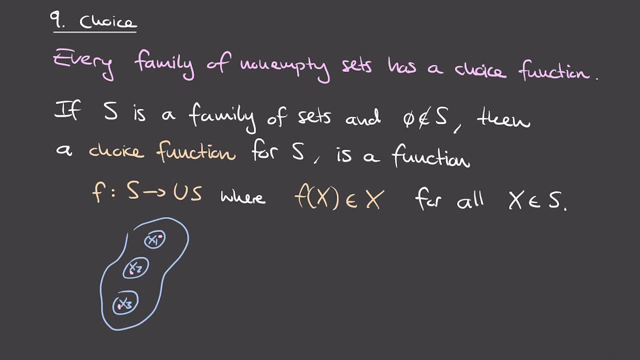 Now, the way to express this mathematically is as follows: So you have this collection here of these x1, x2, x3, and so on, And now what we're going to do is we're going to define a function from this collection. 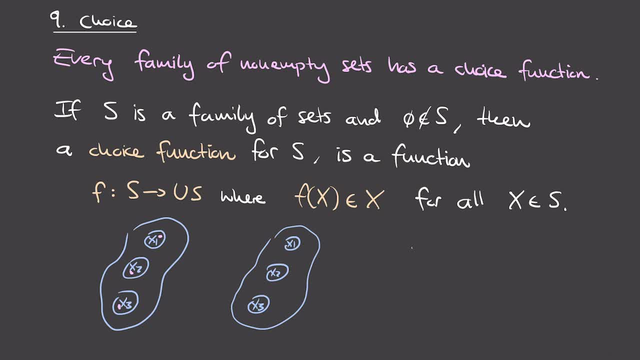 to the union over this collection. So the union will again be a set, but it now somehow contains all of the elements that originally were in x1,, x2, and x3, and so on. So up here we can think about this part. 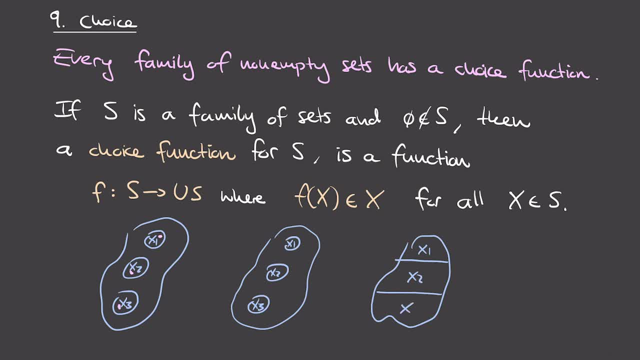 of the union being x1,, this part of the union being x2, and this part of the union being x3. So this thing here I'll be calling s, and then this over here would be the union over s. And now the idea behind picking these elements. 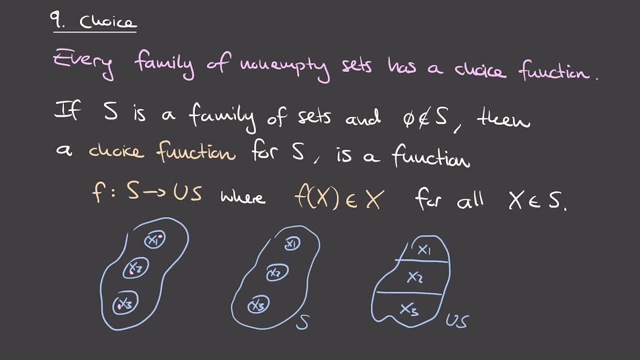 as I've drawn in this picture will be to define a function going from s to the union of s, but in such a way that each of the sets in the collection is mapped to some element occurring in the corresponding part of the union. So here I map x1,. 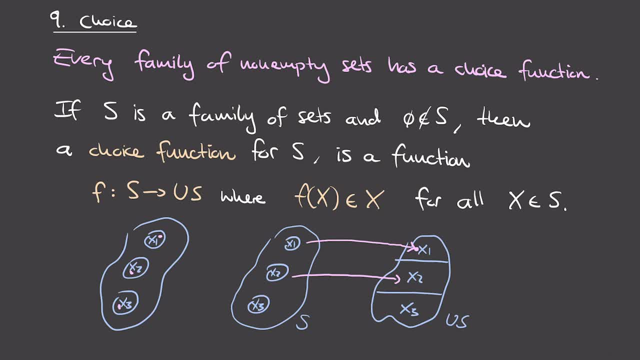 so the set x1 to some element in x1, and I map the set x2 to some element in x2, and I map the set x3 to some element in x3.. And this thing here, so this f, this is a so-called choice function. 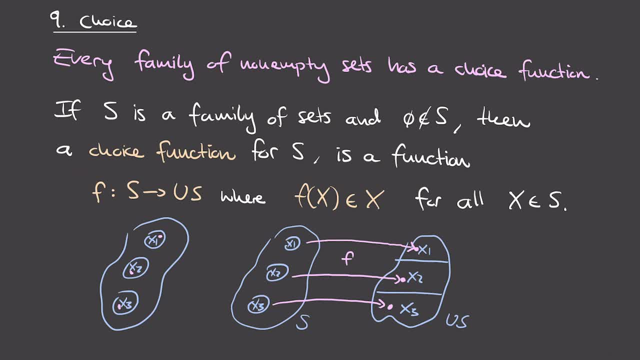 and it satisfies this condition down here. So f is a function going from s to the union of s, and it satisfies that the image of each set x occurring in this collection lies in the set x itself. For instance, if I look at x1,. 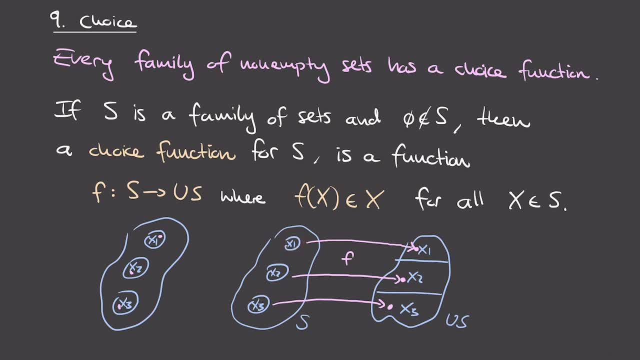 so the function f maps this set x1 to a point, and that point itself is an element of x1. And similarly, x2 is mapped to a point in x2, and so on. So here, what's maybe a bit confusing about this choice function is that somehow 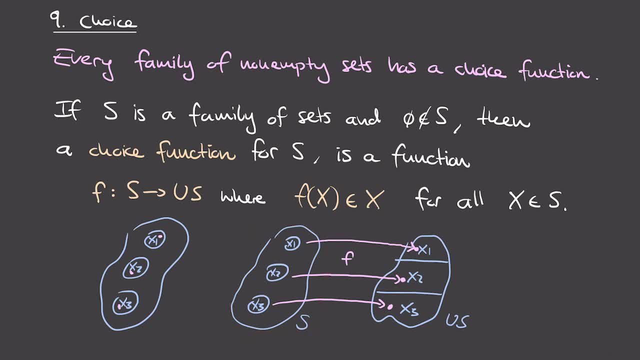 on the left-hand side here we have this family of sets. so in this family, basically these sets here are like the points, right. So each of these sets occurring in the collection is like a point and you map that point to another point. 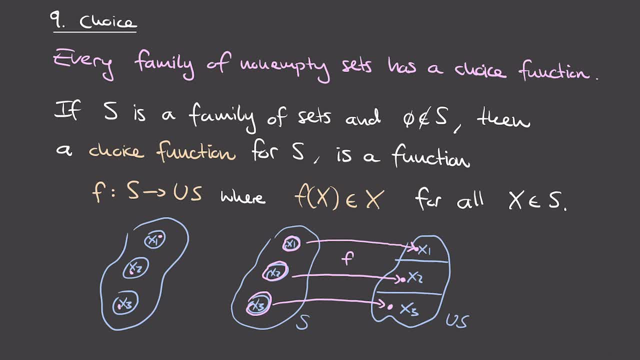 but the point you're mapping to is now a part of the union. So here this point x1 is mapped to some element of x1, and this point x2 is mapped to some element of x2, and so on, And this realizes this idea I presented over here. 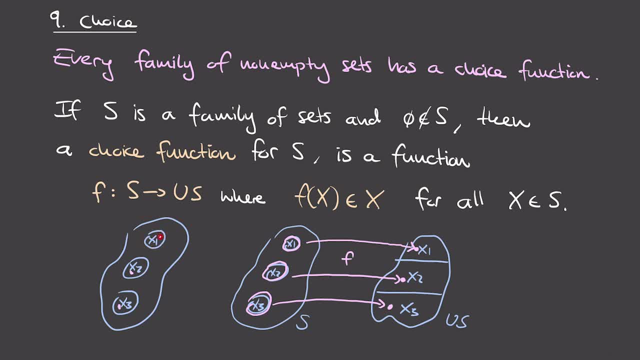 where you want to, for each set, select some element occurring in that set. Okay, with that we can now again read the axiom of choice. So it says: for any family of non-empty sets. so whenever we have this situation here, where all of the sets are non-empty, 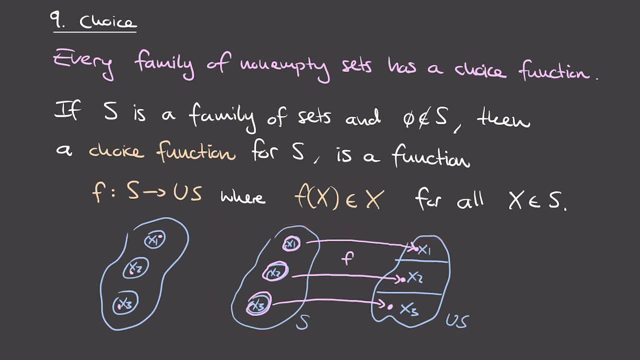 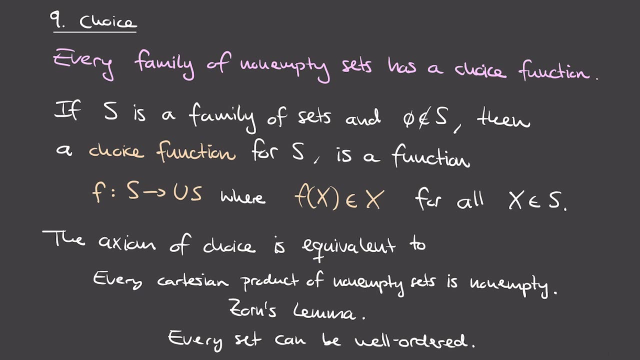 well then, there exists some choice function which allows us to, for each set in this collection, to pick out one of the elements occurring in that set. Now, the axiom of choice is quite strong and it has certain consequences which seem counterintuitive. 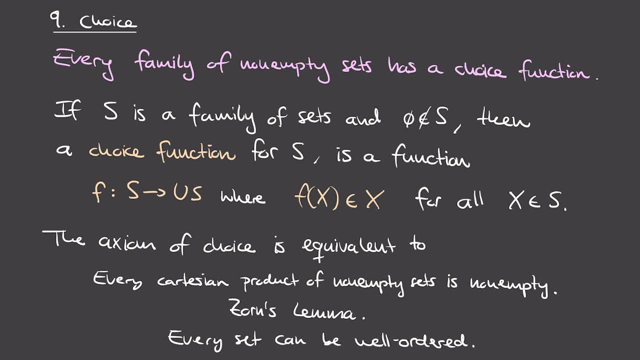 On the other hand, it also has consequences which you really want to have. So it's kind of a weird thing where the axiom of choice is equivalent to certain statements which are very counterintuitive, but it's also equivalent to certain statements which you think should be intuitive. 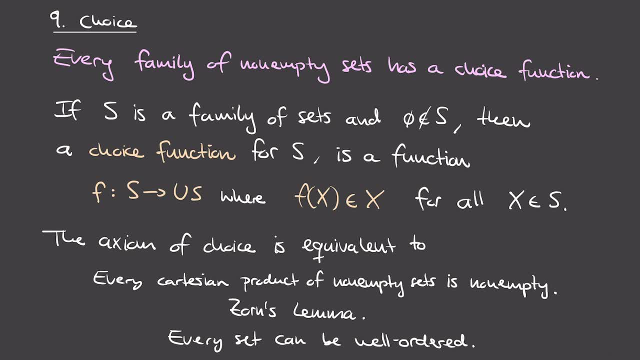 For instance. here I've listed three statements which are equivalent to the axiom of choice. So the first statement here says that every Cartesian product of non-empty sets is non-empty. In other words, the axiom of choice implies that every Cartesian product of non-empty sets is non-empty. 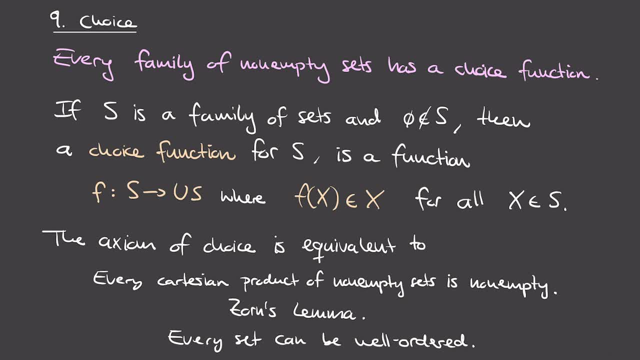 and also, if you don't have the axiom of choice, then there in fact are Cartesian products of non-empty sets that are themselves empty, And here it seems like, well, this is a type of property you would want. so it's weird if you somehow can take Cartesian products. 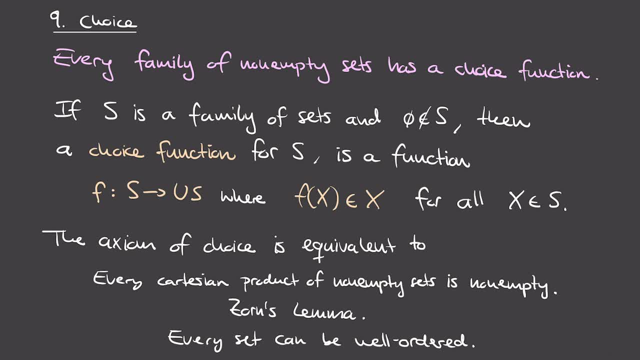 of non-empty sets and somehow have the resulting set be an empty set. Another statement which is equivalent to the axiom of choice is Zorn's lemma. This is something that's used in many parts of mathematics in order to get certain maximal or minimal elements. 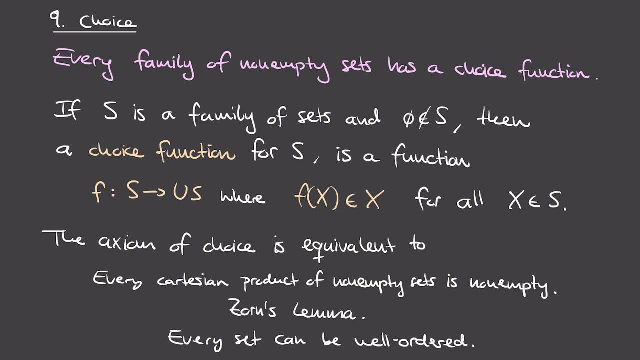 I'm not going to go over what Zorn's lemma is here, but you might have heard of it and well, it's something that's very useful and is in fact required for certain types of arguments, for instance in algebra. So from that perspective also, you would want the axiom of choice. 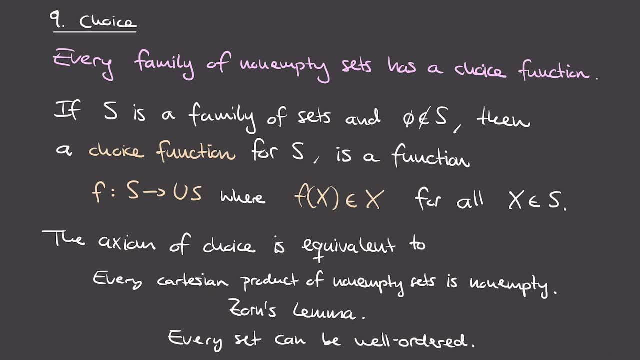 because you want to be able to use Zorn's lemma in math. On the other hand, the axiom of choice also has certain counterintuitive equivalents. For instance, it's equivalent to the statement that every set can be well-ordered. Now, a well-ordered set is a set that has an order relation on it. 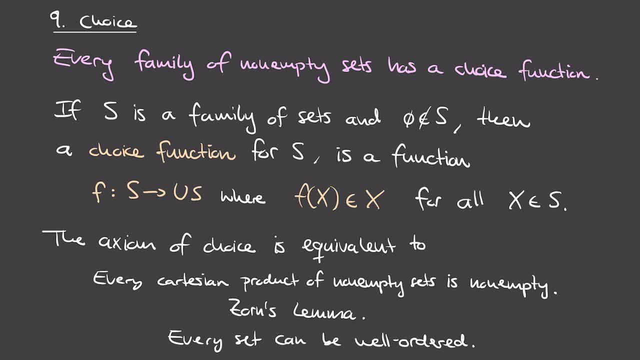 such that every non-empty subset has a minimal element. The standard example for a well-ordering are the natural numbers. So you have like 1, 0, 1,, 2, 3, and so on, and you have 0 being less than or equal to 1,. 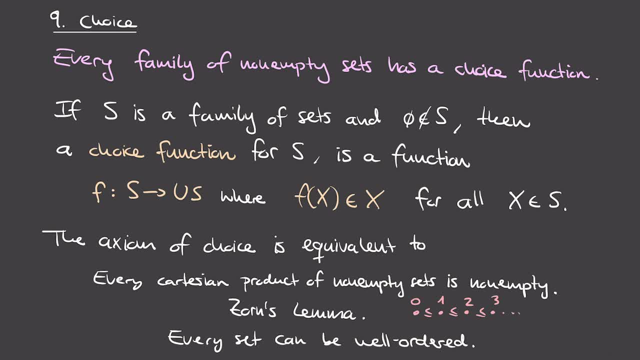 and it continues like that. Now if you take any non-empty subset of the natural numbers, that will have a minimal element. So the entire natural numbers have a minimal element 0, but then if you take any subset you can find a minimal element in it. 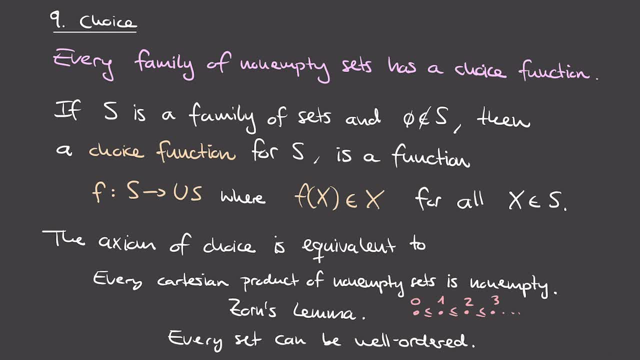 This is, in fact, sort of one of the defining properties of the natural numbers, So it's like the basis for that. you can do induction on the natural numbers. So in this context, having a well-ordered set seems perfectly intuitive. However, this statement is much stronger. 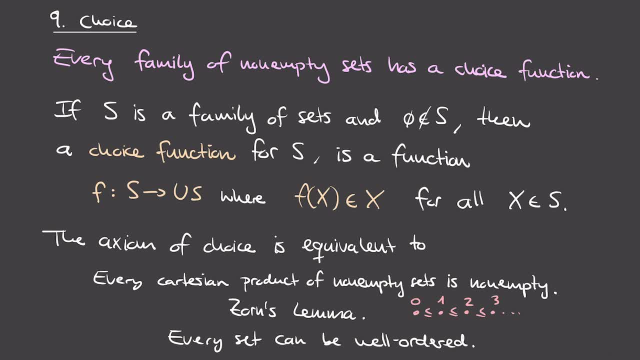 It's saying that every set can be well-ordered, which means that, given any set whatsoever, you can find such a linear order on the set that is a well-ordering. In particular, this means that, for instance, the real numbers can be well-ordered. 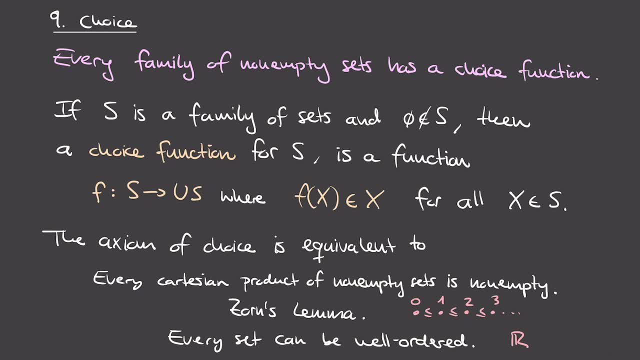 and that's sort of a counterintuitive thing if you think about it. So a well-ordering on the real numbers would be a linear order on the real numbers. but that has the property that if you take any subset of real numbers whatsoever, 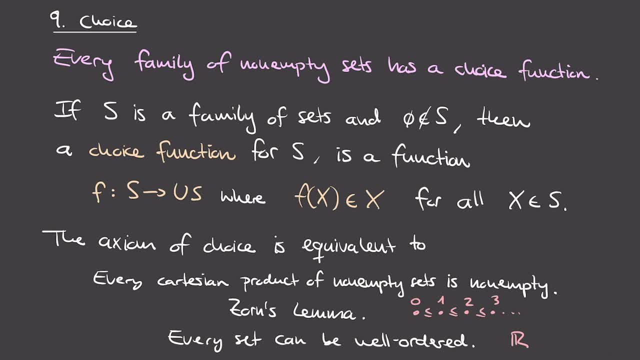 that will have a minimal element. Now, if you think about how this order needs to look in order to be a well-order, you'll find that it's quite hard to do. It's hard to think about and it seems like it should be impossible to construct such an order. 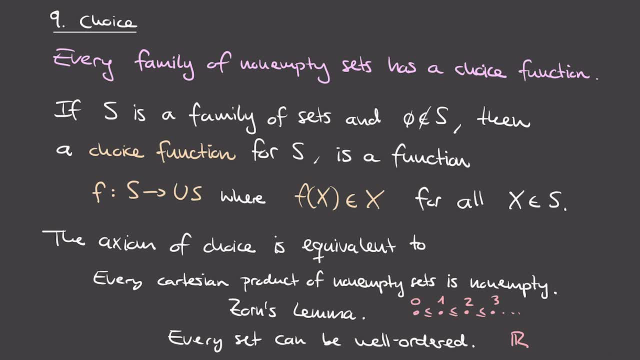 However, you can prove from the axiom of choice in a non-constructive manner that such a well-ordering must exist for any set and therefore, in particular, there must be such a well-ordering for the reals. but the proof doesn't tell you what this ordering looks like. 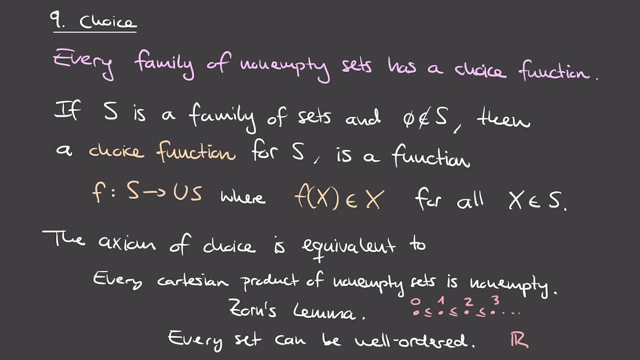 So you're left in the situation where you think that such an ordering probably shouldn't exist, but you can prove that it does, but you still have no idea what the ordering actually should look like. So this is perhaps a counterintuitive property. that is equivalent to the axiom of choice. 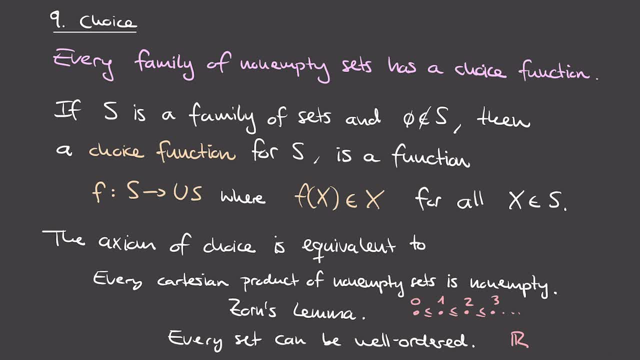 and well, if you look at that sort of property, you might think that you might want to avoid using the axiom of choice because it has these sort of counterintuitive consequences. In fact, there are weaker versions of the axiom of choice that you could still use to build up math. 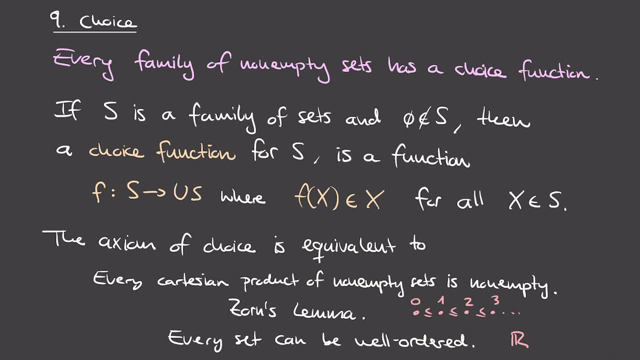 However, in those cases, well, this intuitive property here would then fail. So you would have, for instance, Cartesian products of non-empty sets that are in fact empty, because this statement here is equivalent to the full version of the axiom of choice. 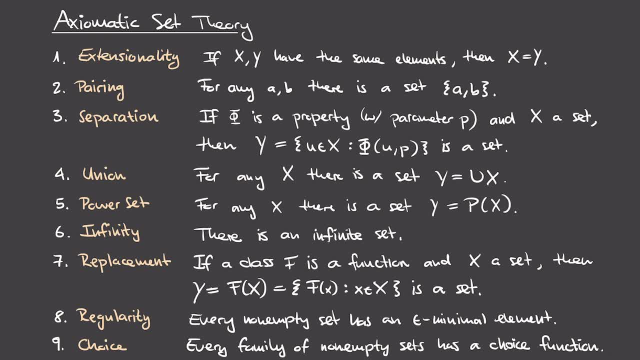 All right With that. we've covered all of the ZFC axioms, so that's quite an accomplishment. and we've also, in the process, built up the basic definitions of set theory. In particular, we've defined relations and functions.